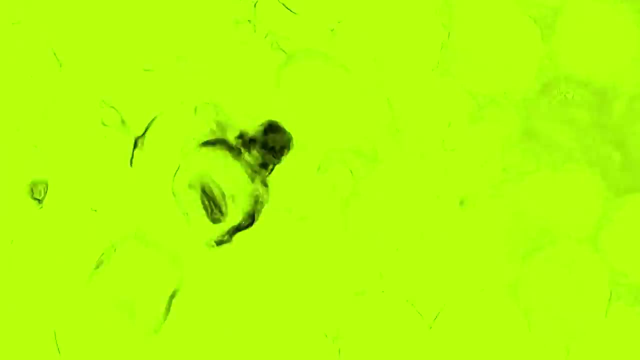 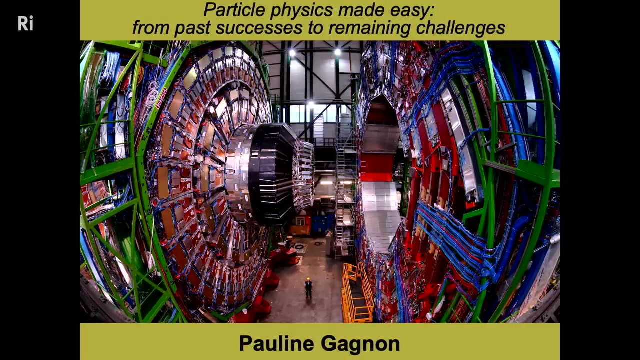 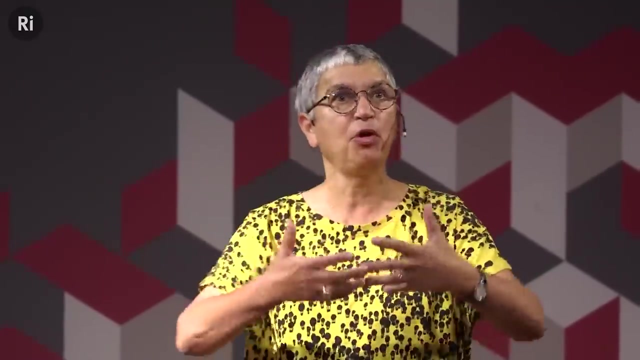 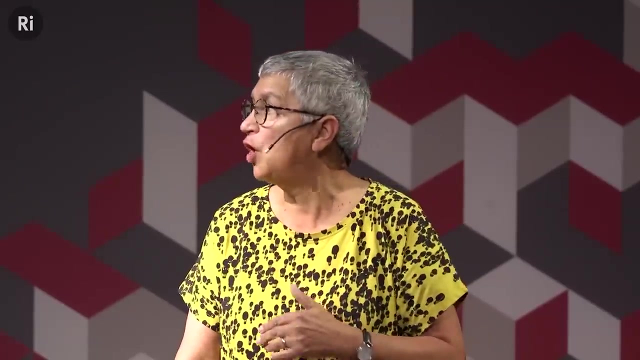 My goal tonight will be to give you an idea about what is particle physics. We'll try to make that as simple as possible, to give you a sense of what we do as particle physicists, Looking at what we have achieved so far and then looking in the future, what is left to do? 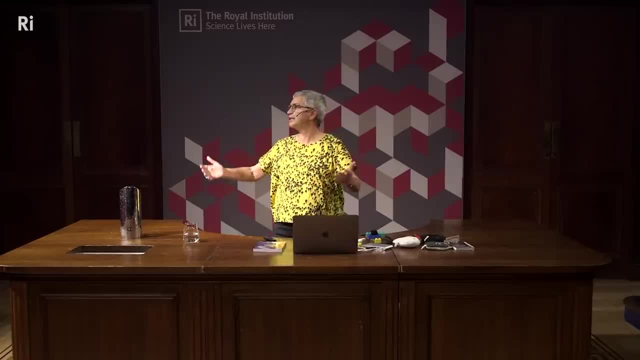 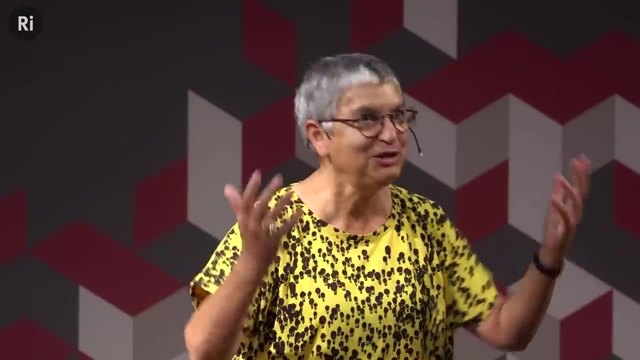 And you know, London is the capital city of musicals and I had the occasion to see my first musical on Saturday night- the Tina show. It was absolutely mesmerizing and I don't know if we'll be able to do something as entertaining here tonight, but I'll certainly do my best. 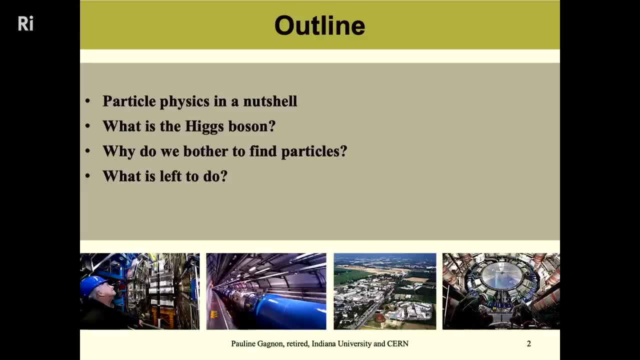 So the outline for the talk tonight first will be particle physics, in a nutshell, how it works. Then, what is the Higgs boson? I know you've all heard something about it, but if you have to describe it it might be something else. 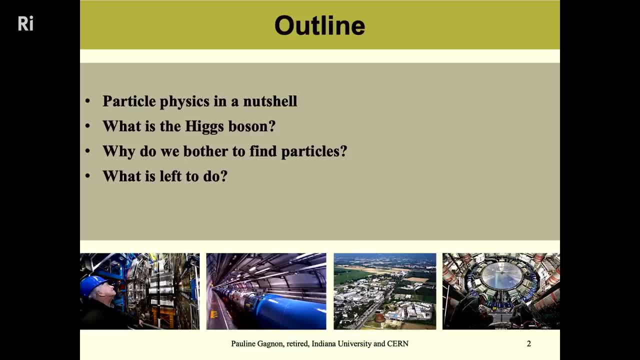 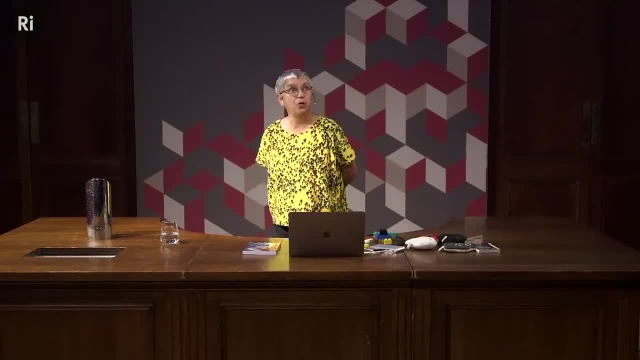 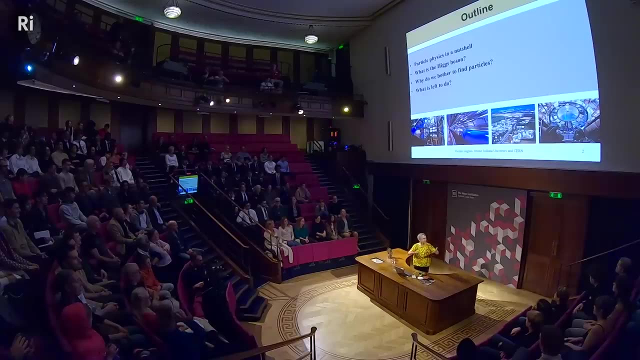 So I'll say a few words to help you better understand what it does. And why do we bother to look for those particles? That's a good question. And what is left to do? because there are lots of students here and it's not much fun when you realize that we have already done all the jobs. but you'll see, we are far from there. 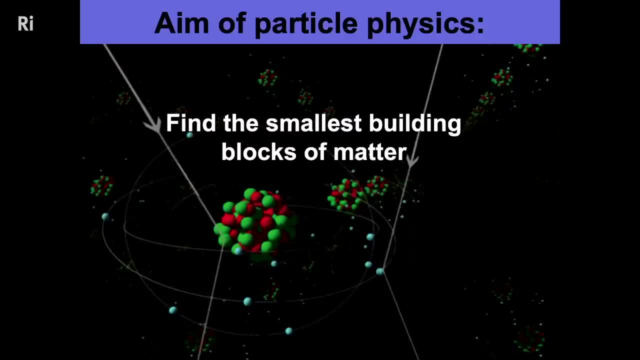 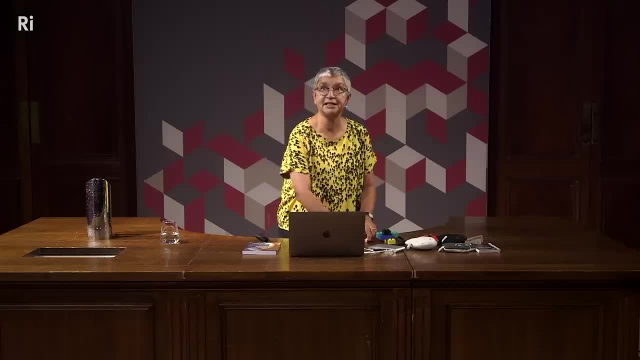 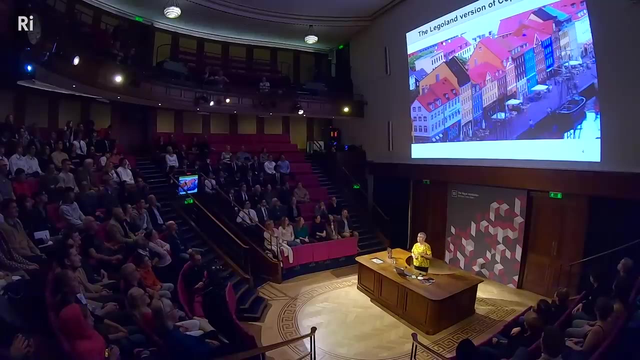 So the aim of particle physics is quite simple: It's to find out what are the smallest constituent of matter. We want to know what are the building bricks of matter, And if we were in Copenhagen, that's where Lego bricks were invented in Denmark. 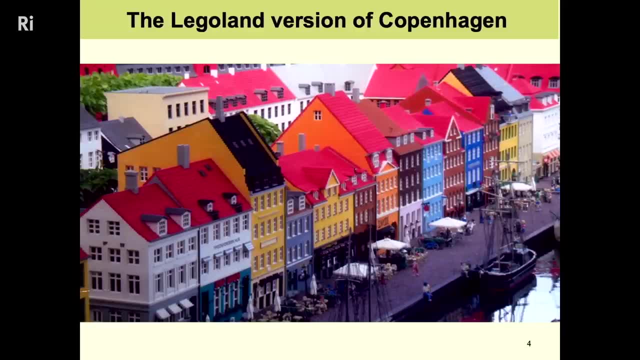 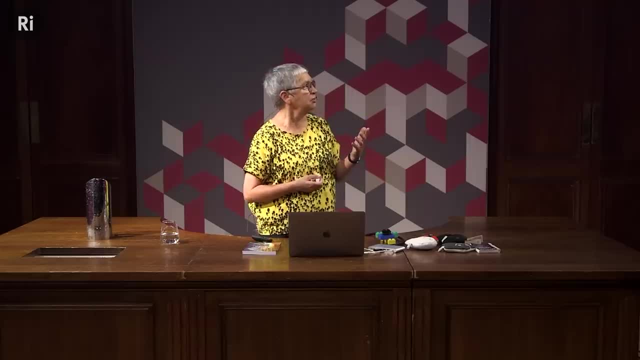 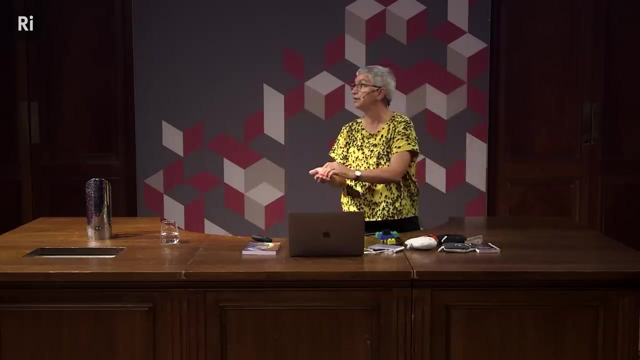 And there is a museum called Legoland and there everything is made of Lego bricks. So if someone there was to ask me what are the smallest constituent of matter, it would be easy. When nobody watches, I would take one of the exhibits, I would break it apart and I would see all the fundamental particles coming out of it. 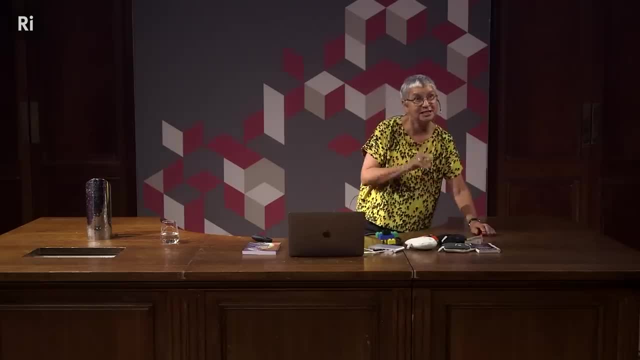 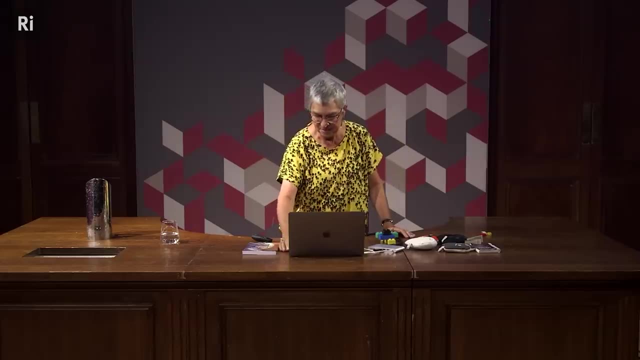 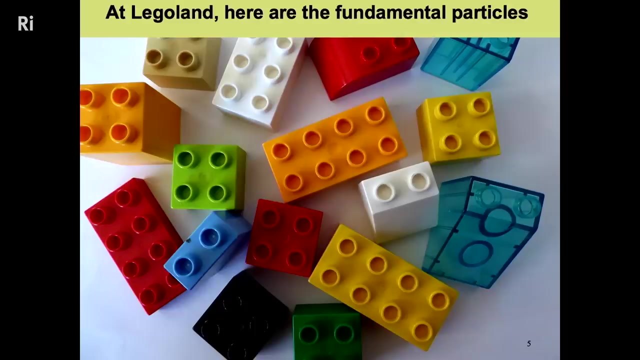 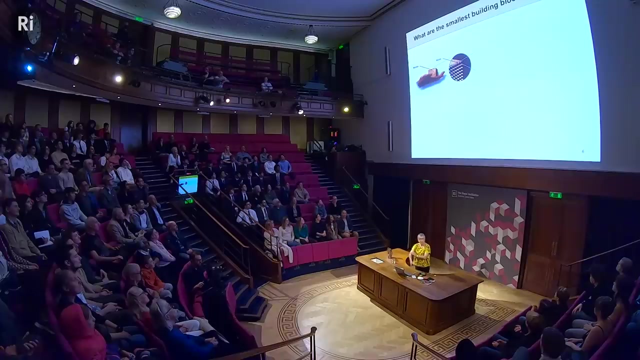 All the building bricks. But Lego bricks is not so simple because they have more than 3,700 different fundamental bricks. But when we look at So at Legoland, these are the smallest constituent of matter. But when we look at real matter, like a piece of wood, our body, this room, everything, the stars and galaxies- 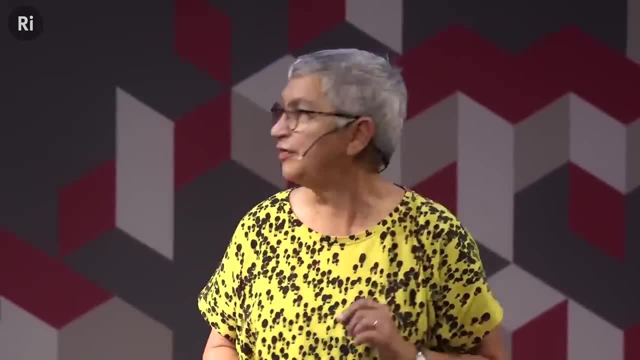 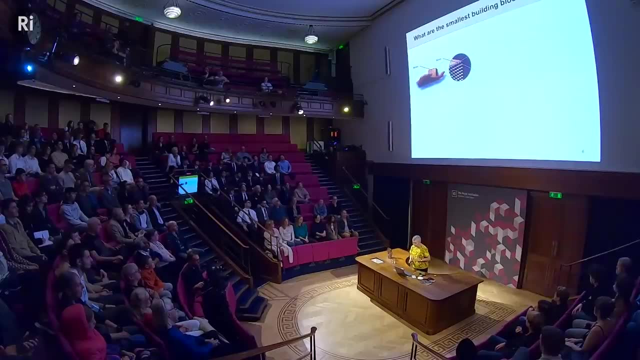 it's not so simple because you know it's made of atoms. but the atoms are so small we don't see them, So it's not so easy. An atom is, in fact, a million times smaller than a human head, So it's really not big. 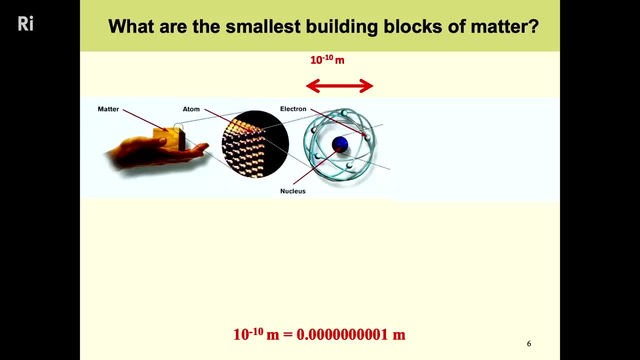 It's 10 to the minus 10 meter. So a meter is a yard roughly, And 10 to the minus 10 is the scientific notation. So you take the decimal point and you move it by 10 positions. So instead of being 1, it's 0.00000.. 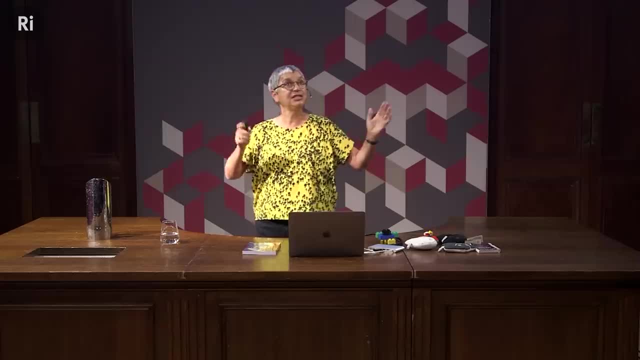 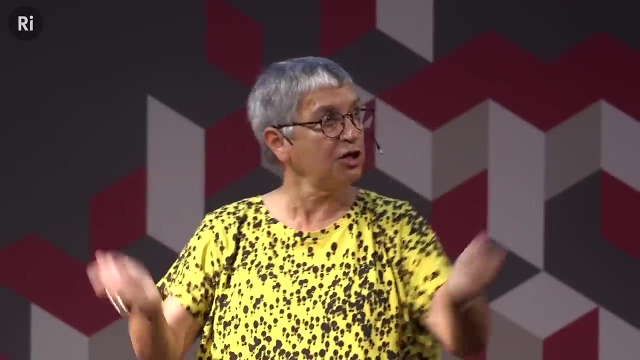 You insert nine zeros in there, And so that's the size. So it's 10 billionths of a meter. An atom, as you know, is made- Sorry, I backtrack- An atom is made of a nucleus and some electrons that gravitate around it. 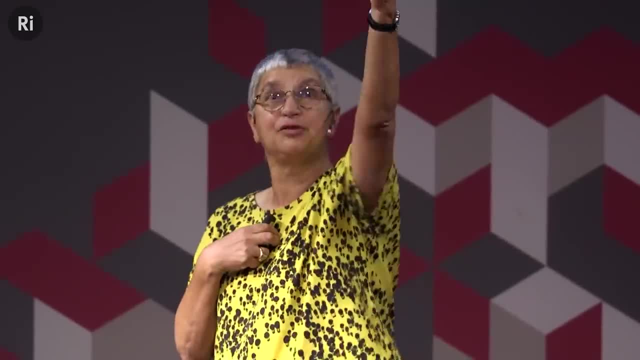 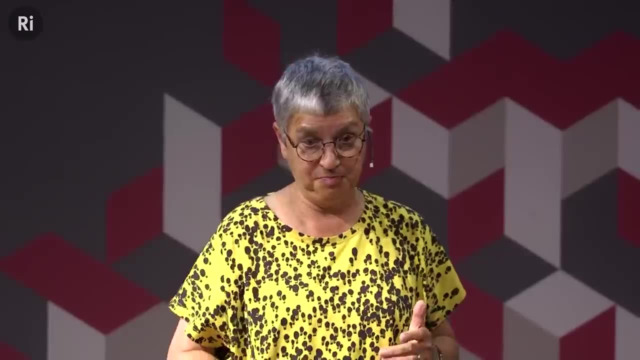 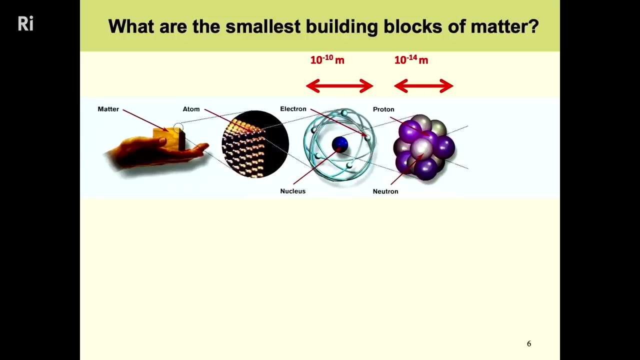 If I was a nucleus, my electrons would be 12 miles apart. So most of an atom is in fact emptiness, vacuum. The nucleus itself is quite small: It's 10 to the minus 14. It means 10,000 times smaller than an atom. 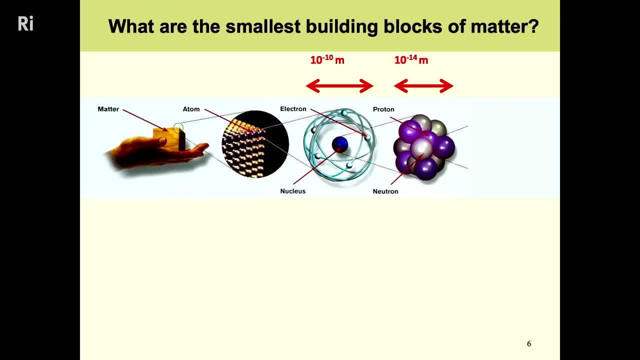 And inside the nucleus you find protons and neutrons. I think up to here you have probably all heard this. So the protons and the neutrons themselves, they are much smaller, They're about 10 to the minus 15,, I believe. 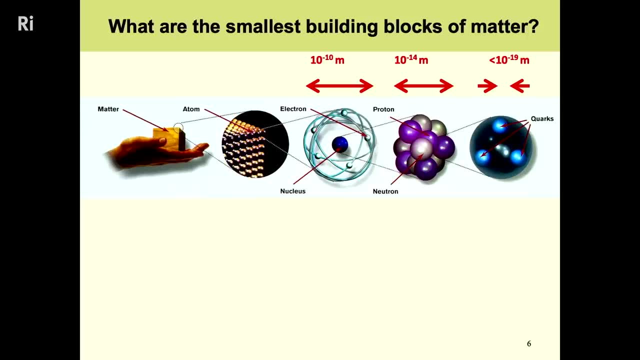 And inside, And inside the protons and the neutrons, you will find quarks, And the quarks are smaller than 10 to the minus 19 meters. So if I ask you now, what are the smallest constituent of matters that you see there? 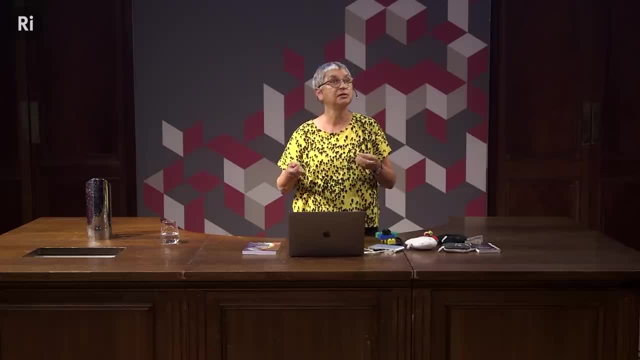 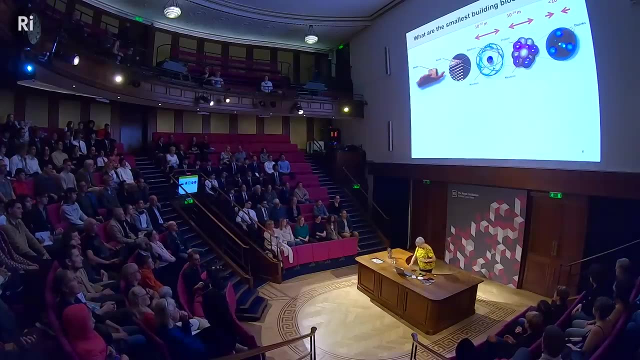 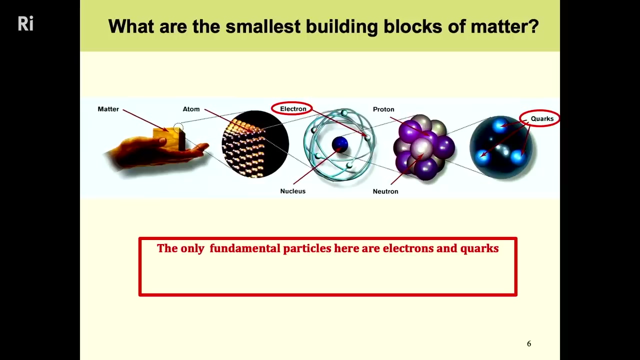 that we cannot break any further. Which ones do you see? Quarks, yeah, And Electrons. that's it. Those are the only fundamental particles there, Electrons and quarks. I'll show you that with just two types of quarks, two different types of quarks. 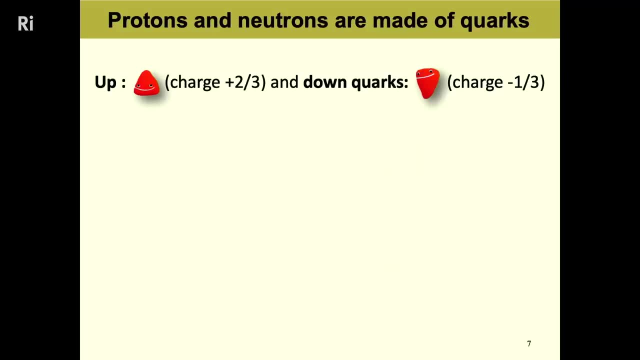 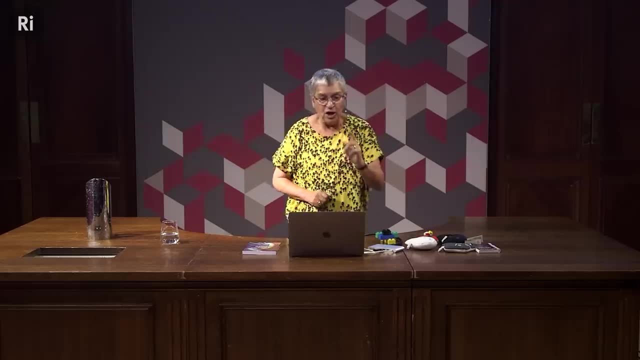 The up quarks and the down quarks I can build And electrons I can build- all the matter that we see here on Earth, stars and galaxies. See, if you take an up quark, an up quark has an electric charge equivalent to two thirds. 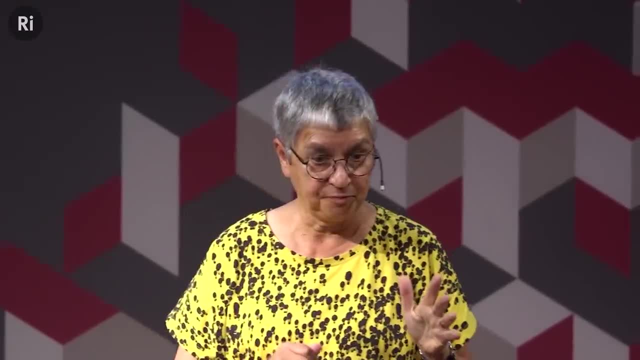 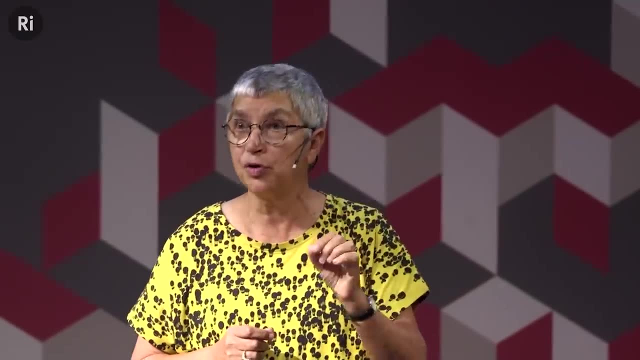 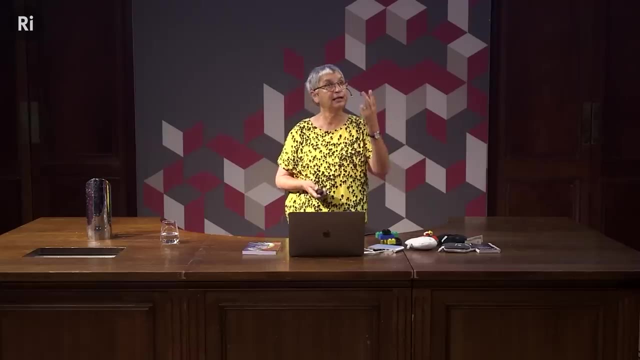 of the charge of an electron, But it's positive And a down quark has a negative charge And it corresponds to one third of the charge of an electron. So if I want to make a positively charged particle then I can take two up quarks. 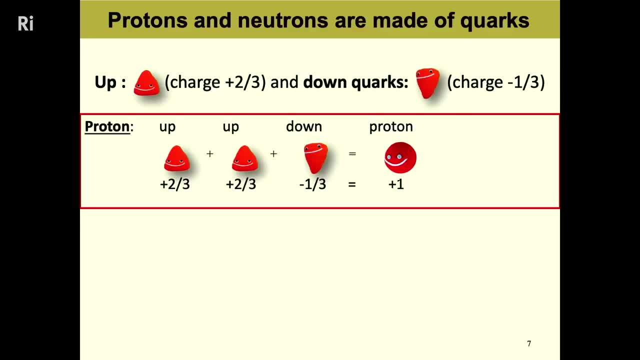 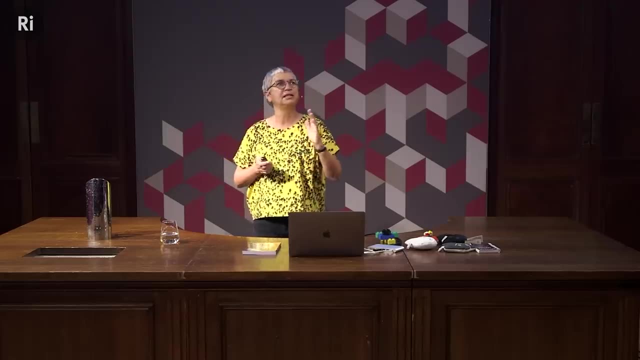 two thirds of the charge of an electron. twice so it's four thirds. And I add to that a down quark And then I get two plus one, So that's the charge of a proton. And so with up and down quarks could you make up a particle that is neutral. 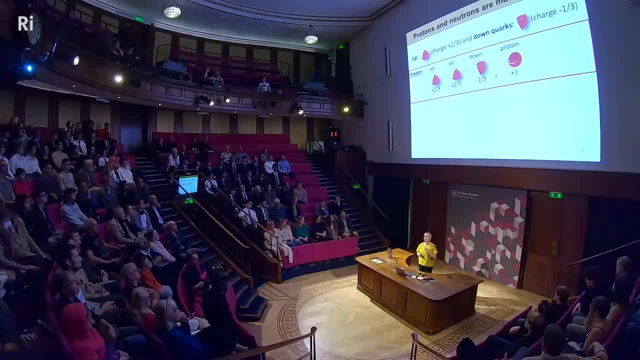 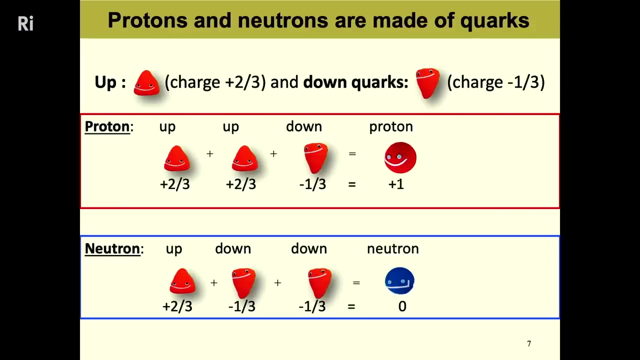 Yeah, Who said yes? Okay, so what do you do? Voila, Two down quarks and one up quark. So that's what a neutron is made of. Okay, very simple, And you know that The whole periodic table, the only difference from one element to the next. 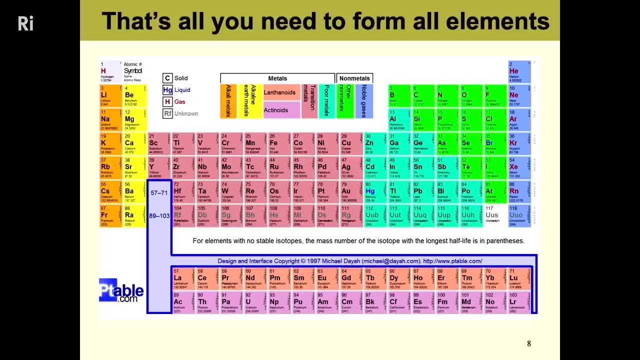 like the lightest one is up here, the hydrogen. it has only one proton in its nucleus and one electron around. The next one is helium. All you do to change an electric element, you just add one proton to the nucleus. So helium has two protons, two neutrons for stability. 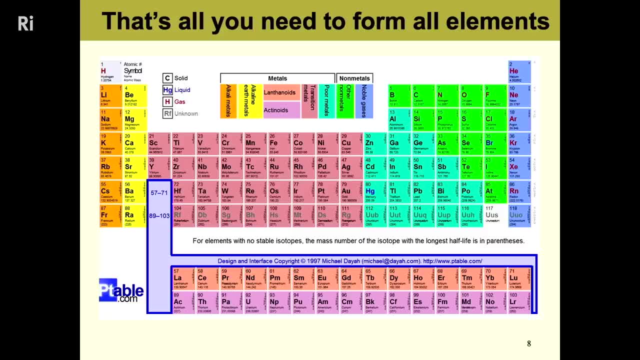 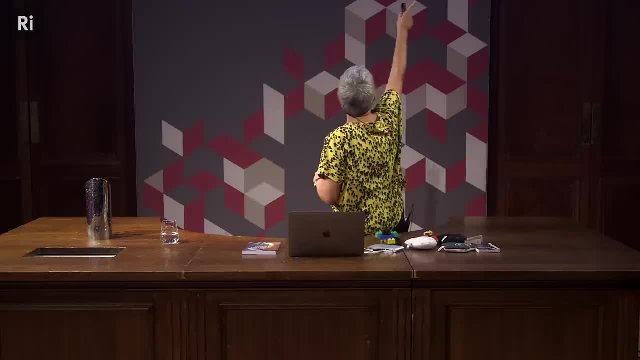 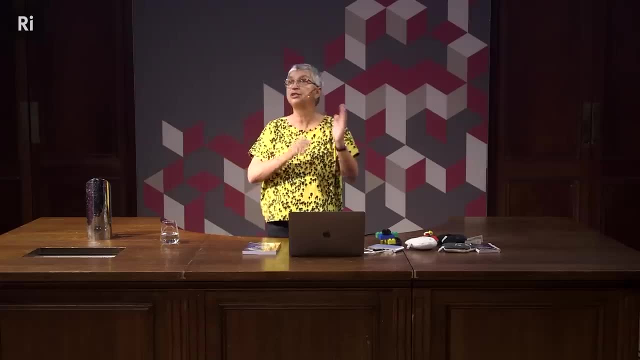 and two electrons around. The third one is lithium, and there you have three protons and so on and so forth. So you see, you can build all the 119 of those elements just by putting more protons in the nucleus. And that's the difference between the different elements. 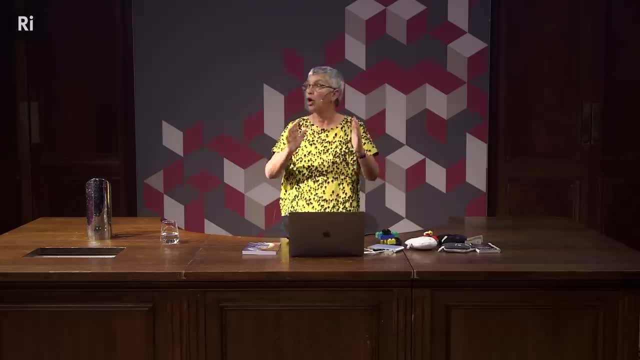 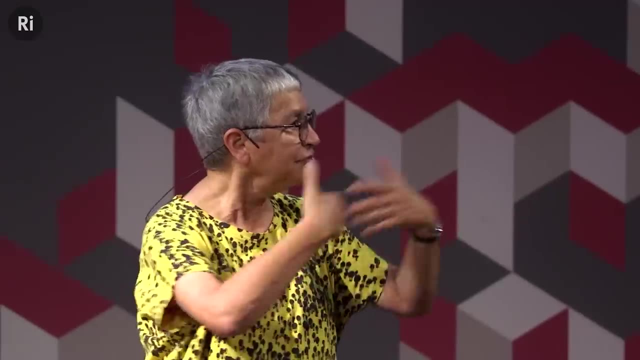 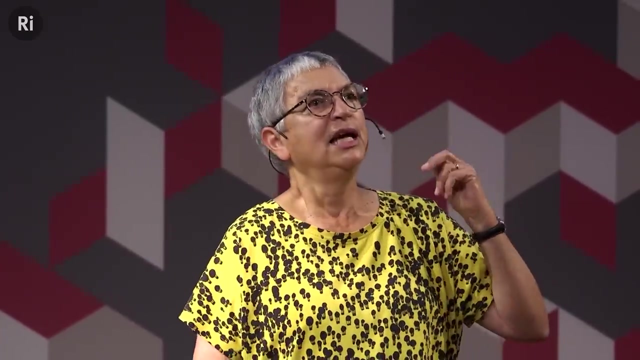 that we find in the periodic table. So that's it. With up quarks, down quarks, you put all type of chemical elements and you know that everything that we have on Earth is made of those elements. It was my dream when I was about 14, in 1969. when they went on the. It was which one Apollo 9 mission that went on the moon? 11? Apollo, Apollo 11, and they went on the moon and I was hoping they would find new elements. They found the same chemical elements that were here. 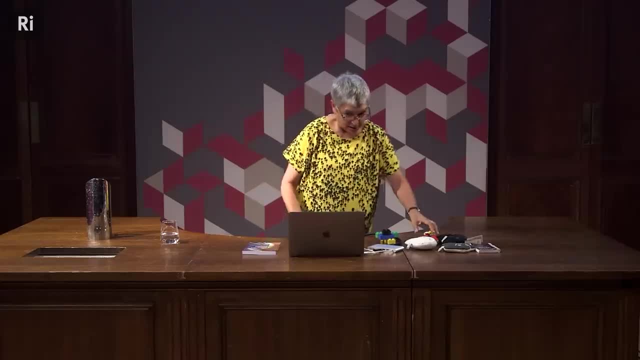 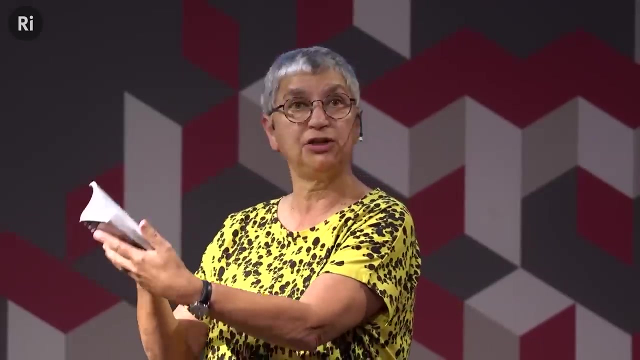 And so. So in the 60s it was really difficult because we had hundreds of different particles. Today, there are more than 230 different particles that are listed in this little booklet with all their properties, and now we know that it's not so common. 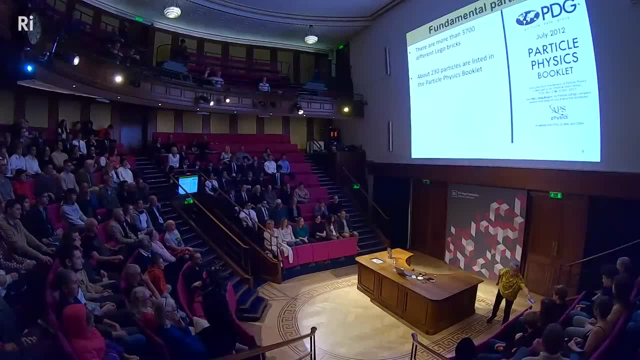 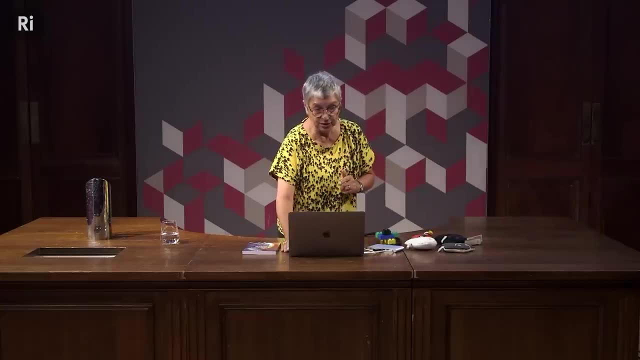 It's so complex At first. you can have a look at that, You can pass it around. At first, people didn't understand why there were so many, And it's far from being like the Lego bricks, with more than 3,700 different pieces. 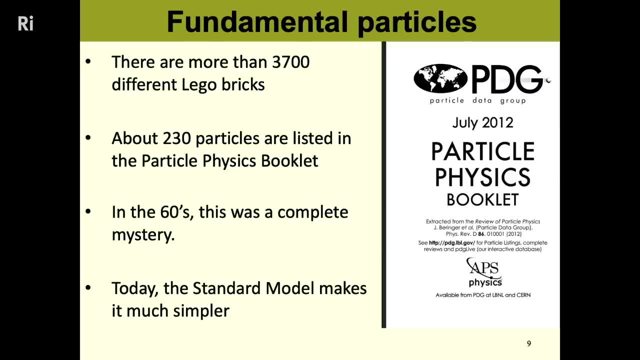 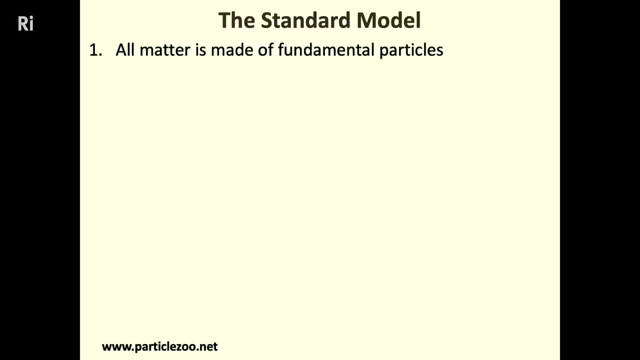 Today we know that it's very simple, and it's so simple that we can make it even simpler than the periodic table, and that's what we call the standard model. The standard model is just a theoretical model to help us classify the particles. 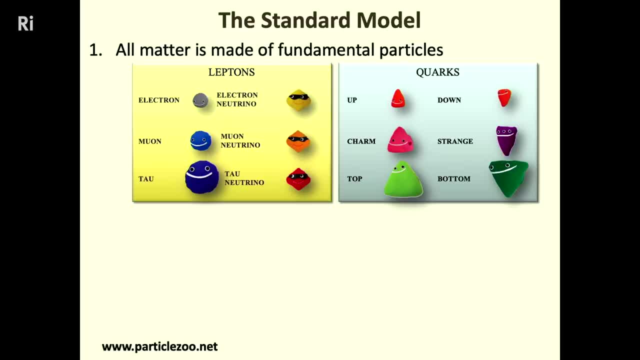 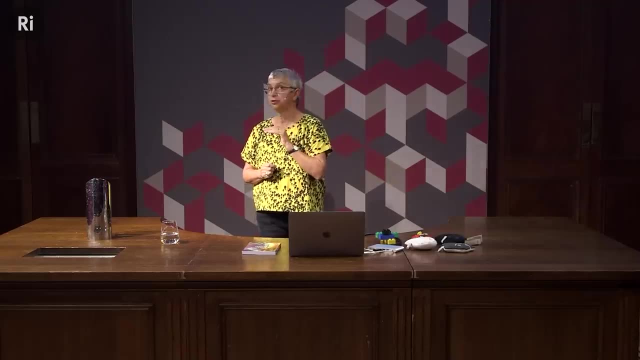 And it tells us it has two principles. The first principle is that all matter is made of particles. All matter can be broken down into the elementary particles, And it tells us that there are in fact 12 different particles. These particles come in two families. 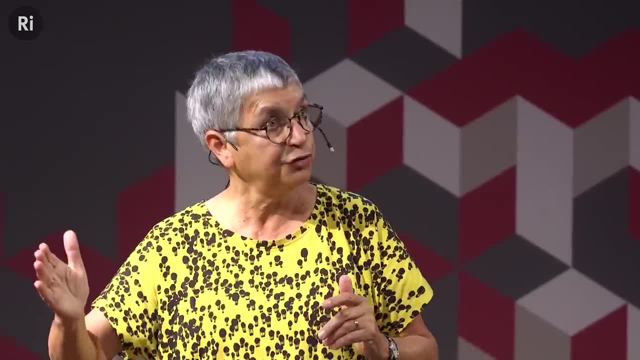 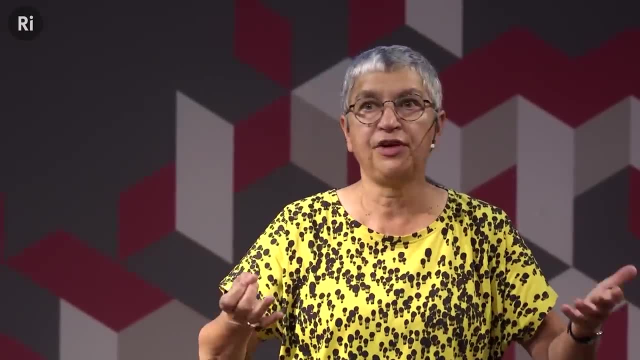 the family of leptons and the family of hadrons. the ones that are built out of quarks, like protons and neutrons, are in the family of hadrons. I'm a Gagnon, they are hadrons, Just a family name. 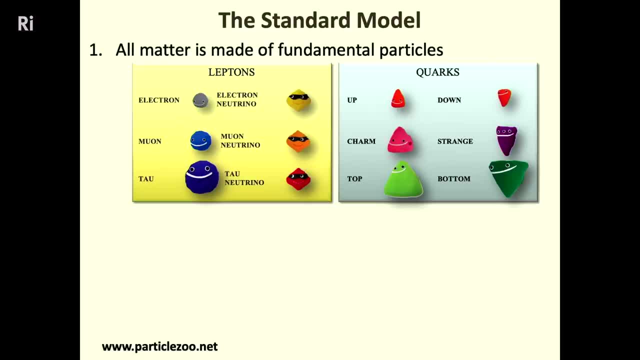 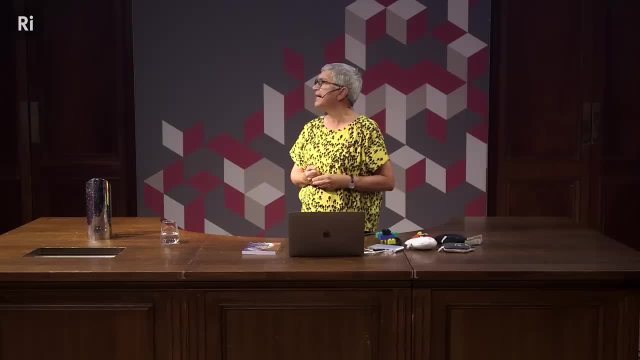 So I already introduced the up and down quarks. for the quarks Those are the lightest ones. And then there is the charm and the strange quarks. Strange quark got its name because all the particles that contain that quark were having a very strange lifetime. which was much longer than all the other particles that we knew before. So it was called the strange quark. The next one came. that was a discovered next quark. Then people said, why not The charm quark? This one had charm. 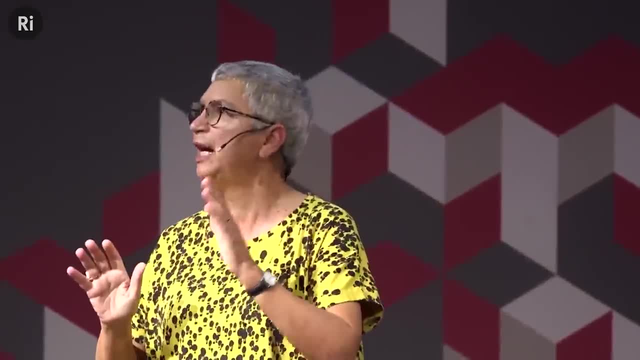 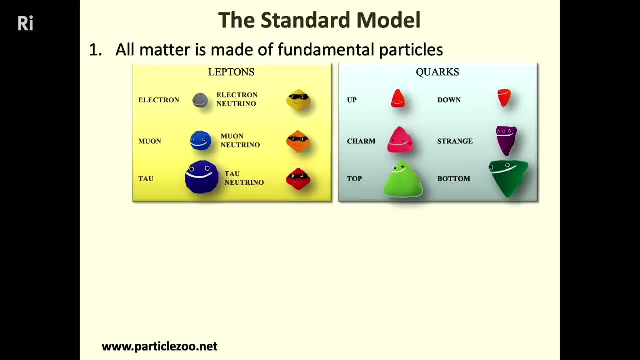 And then they went for truth and beauty. but then we said, OK, enough of that, And we kept the true T for top and beauty, B for bottom quarks. So now we have the top and bottom quarks. So the top quark is the heaviest of all the particles. 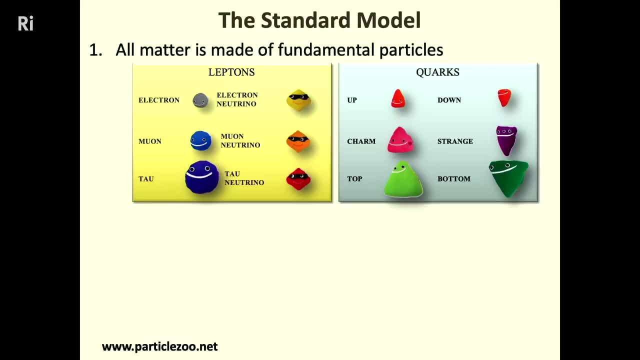 and it's quite heavy. So that's the family of quarks, hadrons and the family of leptons. You know the electron. The electron also comes with a muon, sorry, with a neutrino, When we create electrons in the laboratory. 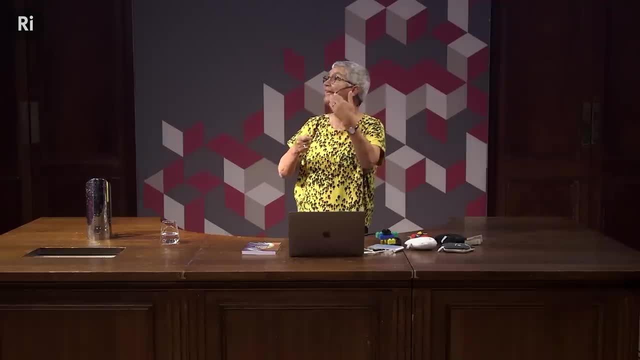 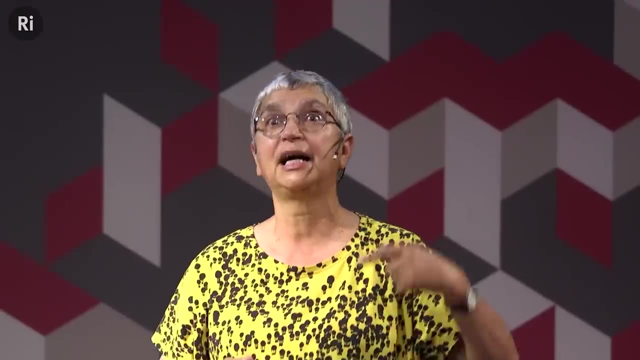 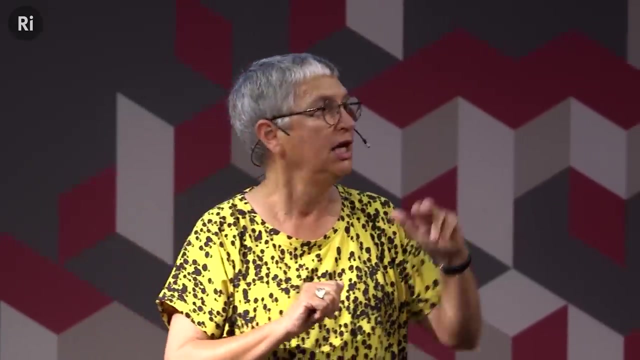 it's always produced either with an anti-electron or a neutrino. All these particles that you see here also have their antimatter. So particles that are antimatter. they are identical, except that all their quantum charges are inverted, Like their spin will be inverted. 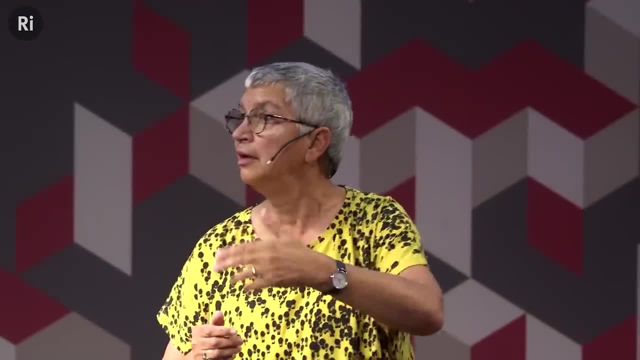 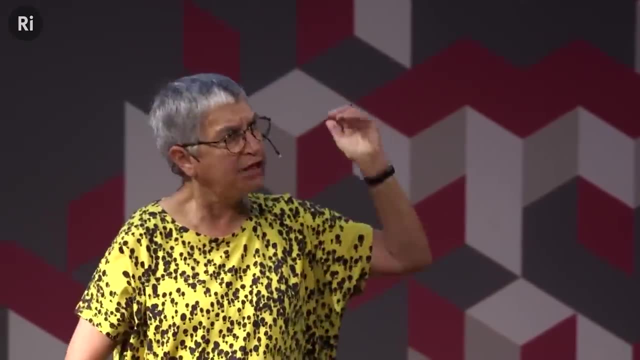 They will spin in the other direction. Their electric charge will be positive for a positron instead of the electron, which is negative. OK, so in the family of leptons we have the electron, then the muon, which is 200 times heavier. 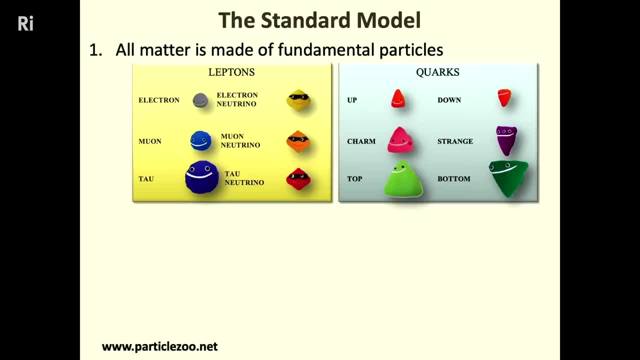 but similar to an electron, And it also comes with its neutrino. And finally, the tau particle, which is 4,000 times heavier than the electron, and it also comes with a neutrino, And I brought one here. and those are the. 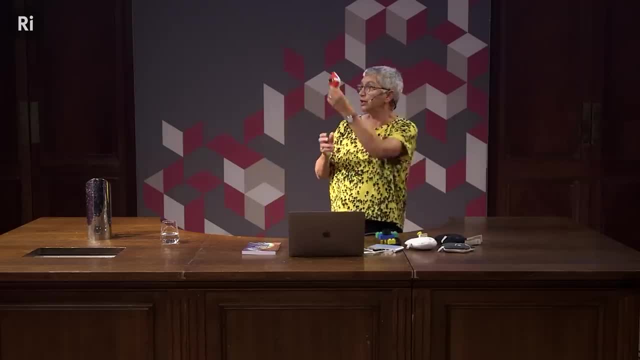 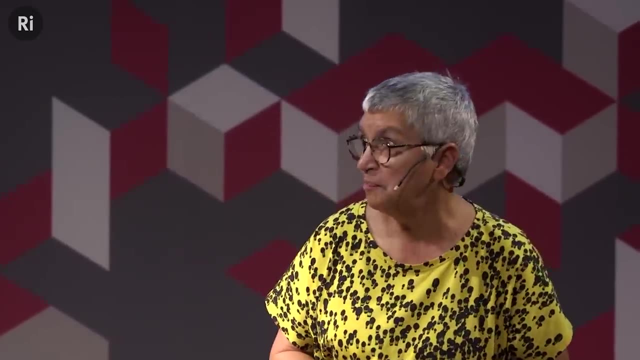 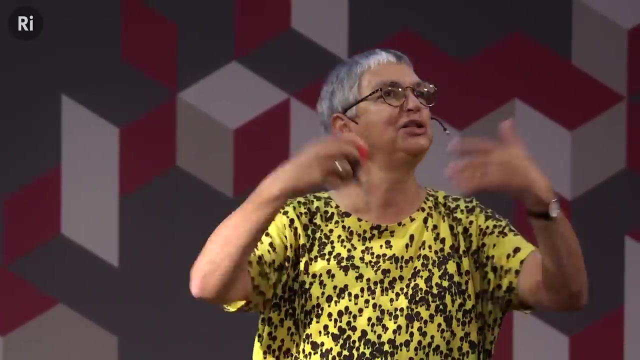 So now you know that it's real, And so this series of little characters come from the particle zoo, And it's a young woman, Julie Paisley, from California, who attended a lecture like this one day, and then she thought it was cute. 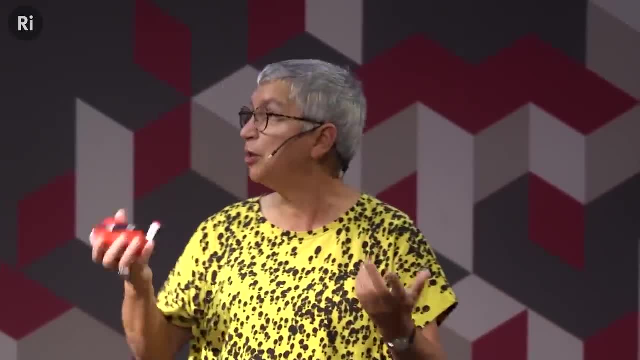 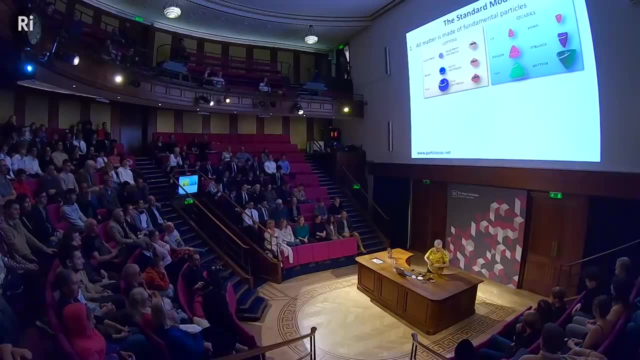 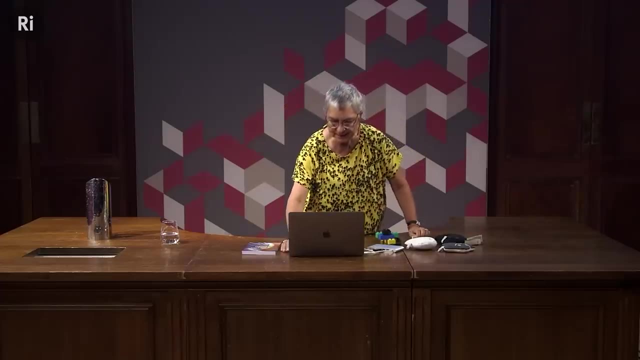 and she was a seamstress so she started producing the particle zoo And you can order them on the web So I can pass the tau neutrino And what is really weird, it's like you know we have a construction set. 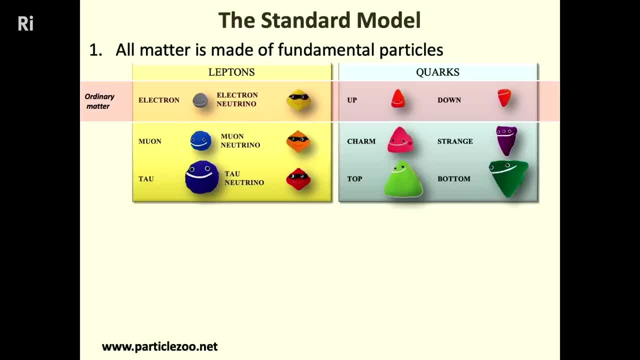 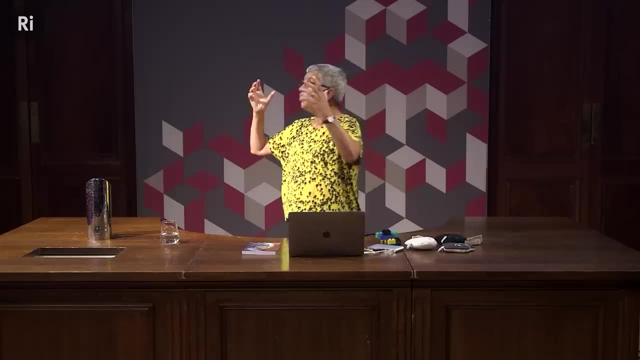 but the only particles that we need to build everything that we see on Earth and in the universe is the first generation of particles: Up quarks, down quarks, electrons. It's like I'm giving you a very nice construction set at Christmas time. 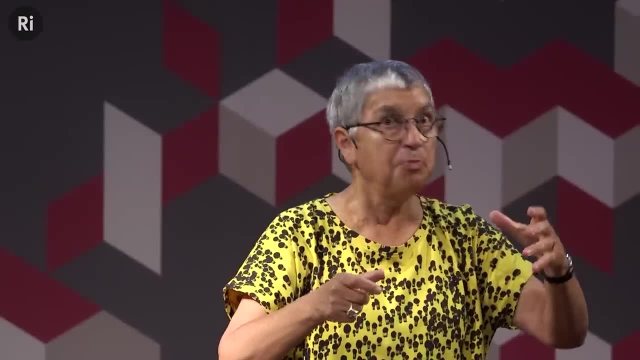 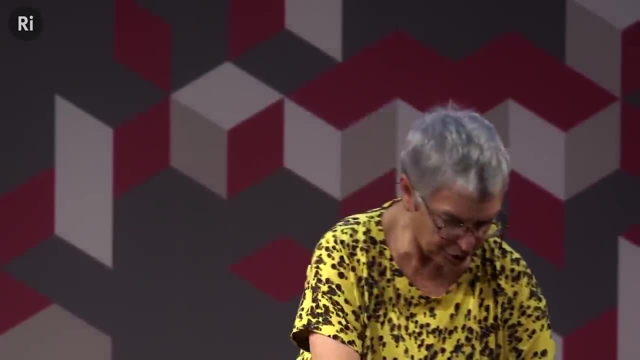 and it has all sorts of models that you can build, but in all those things you never use the second and third generation. It's like you have the basic particles, up and down quarks, and then the other ones. they don't fit. 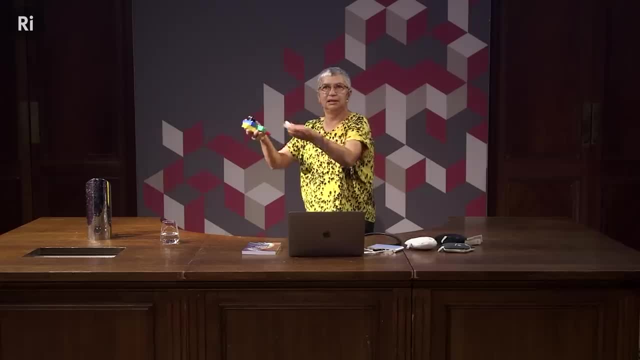 They're duplos, They're not Lego And that It doesn't fit together. So it's a funny construction set, because the tau muon, the tau lepton, is 4,000 times bigger than the electrons, So it's a very weird construction set. 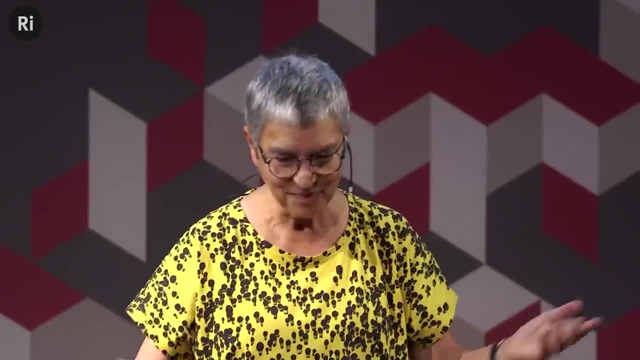 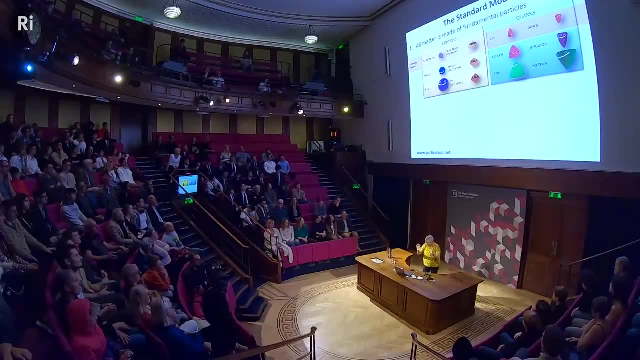 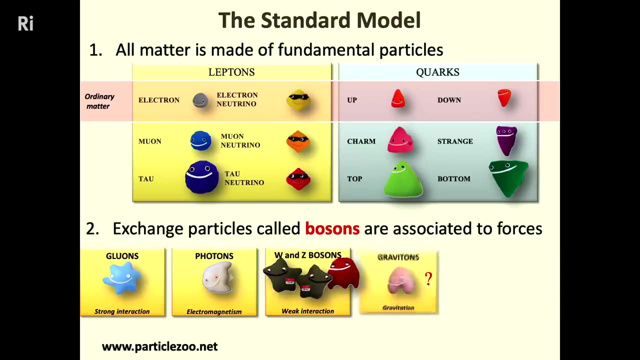 and you never use it. So it's strange. That's one thing that we don't understand. But we know now that there are these 12 basic particles and their antimatter, their antiparticle. The second principle of the Standard Model says that matter is made of fundamental particles. 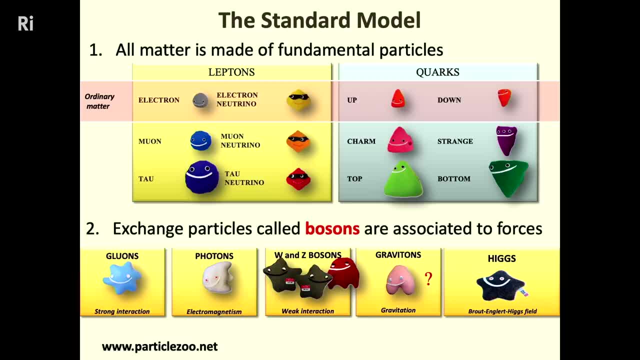 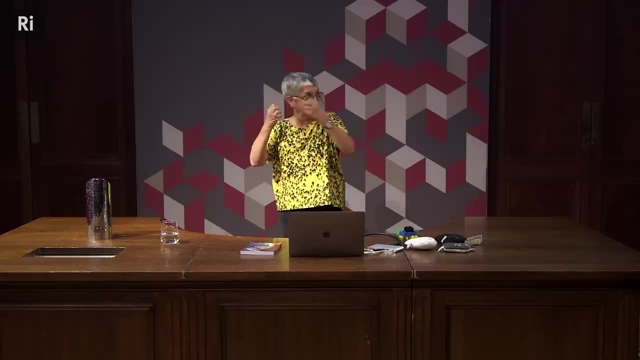 and they interact with each other by exchanging other particles that we call bosons, and those particles mediate the forces between those particles And the first one that is there is the gluon. That's what you find, that will glue, hence the name. 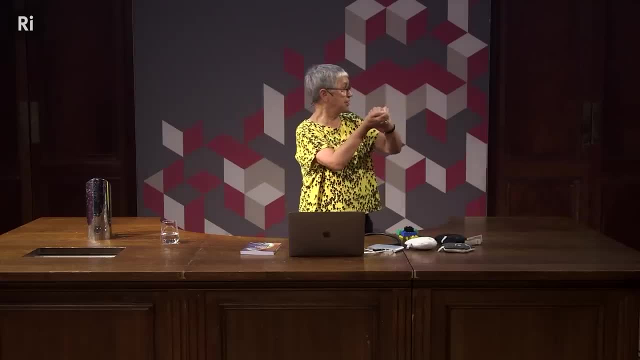 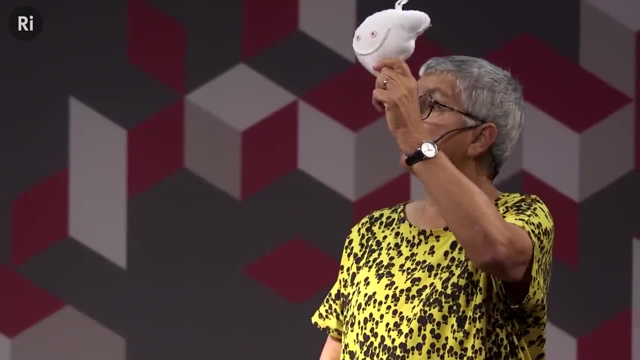 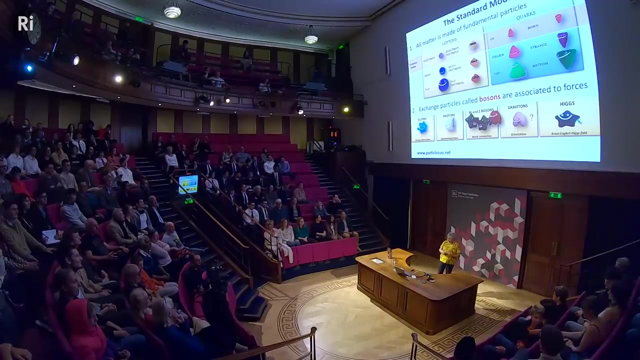 that will glue the quarks together to form protons and neutrons, for example. Those are gluons. Then you have the photon, which is associated with the electromagnetic force. So here is a photon And you have which is massless. 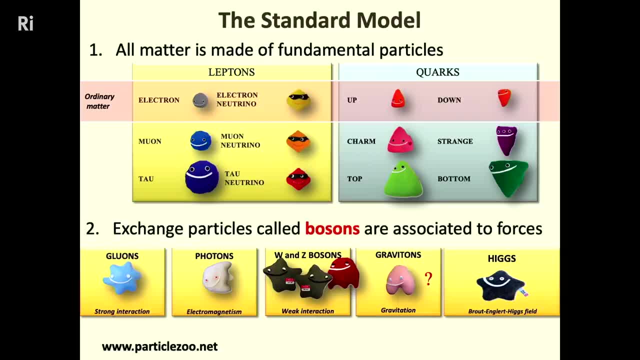 Then you have the W and Z bosons, which are the mediators of the weak nuclear force, which is way stronger than a bit, weaker than the strong interaction between quarks and gluons, And that's the process that takes place on the sun, in the sun. 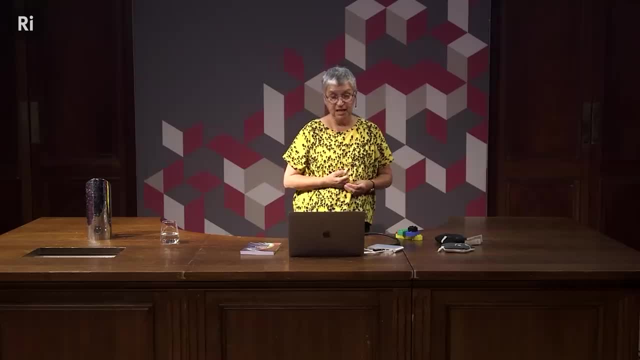 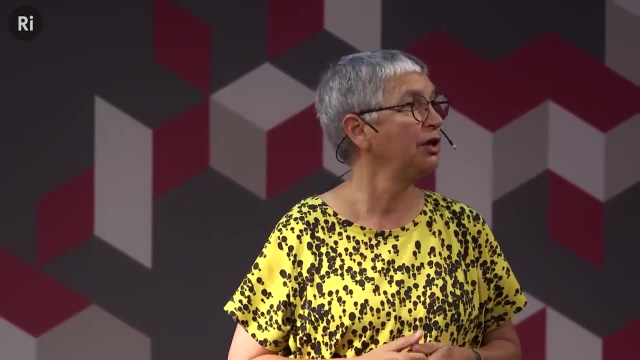 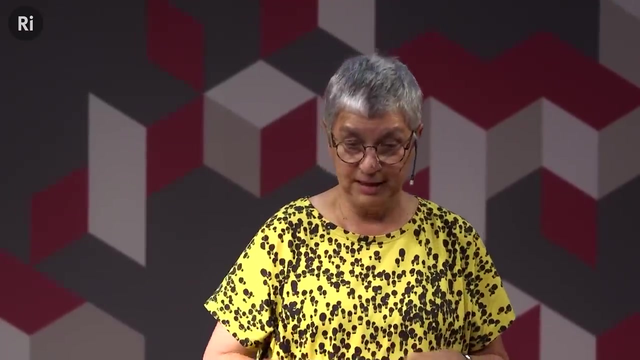 and how the sun burns its energy. Graviton: we haven't found it yet, But we have found. about 10 years ago we found the first gravitational waves, So we think that they will probably come with a graviton. And finally the Higgs boson. 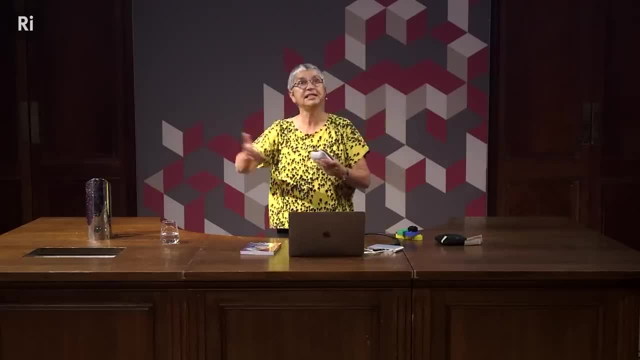 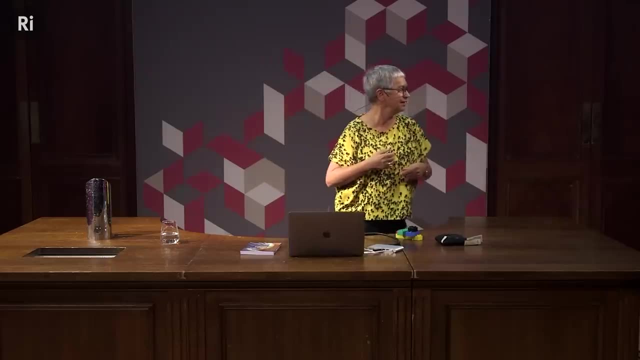 Ta-da, The Higgs boson which recently got discovered 10 years ago at CERN, and we'll talk more about that. Here's the Higgs boson and you notice the difference: This one has mass. What is this business of exchanging particles? 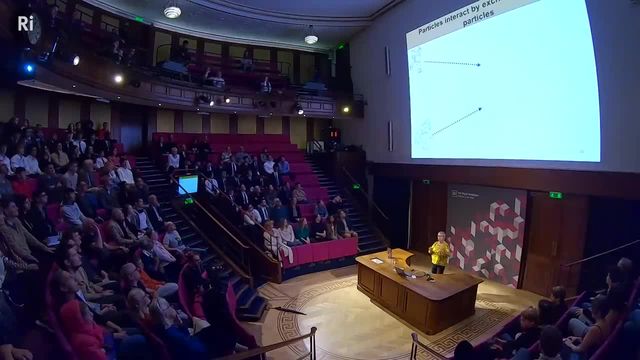 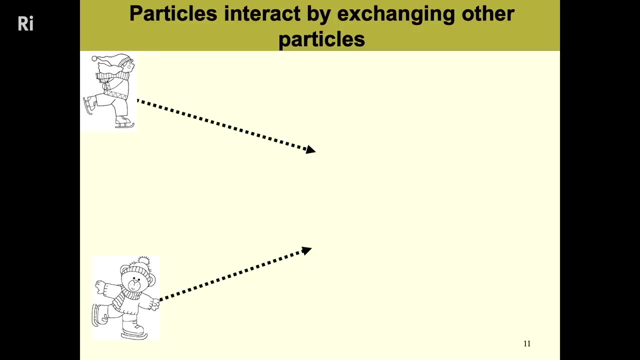 those bosons. It works like this, Like: imagine two particles, like two skaters that are evolving- you know, skating on the ice- and they ignore each other. They don't know that the other one is there. They do their own business. 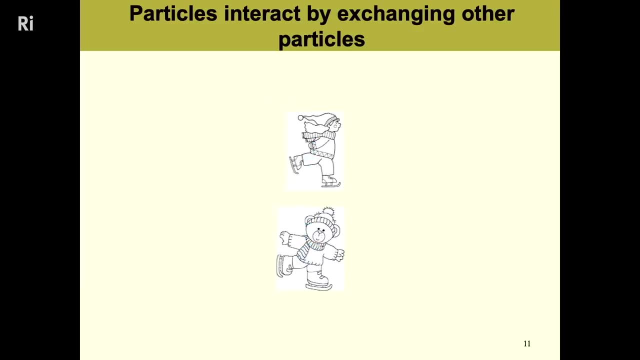 And they would go on a straight line. but the first one, Nasty, tosses a heavy ball at the second one and makes him deviate And she himself will recoil. So both of them are recoiling. So instead of continuing like this, 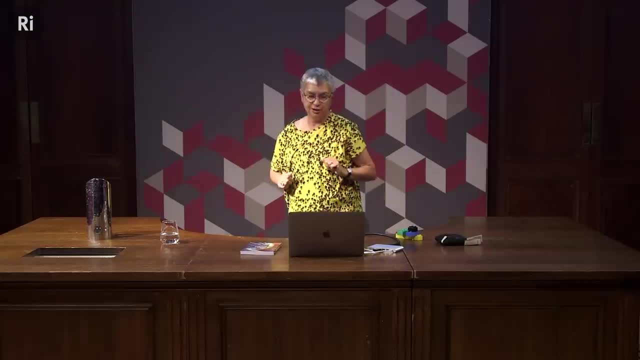 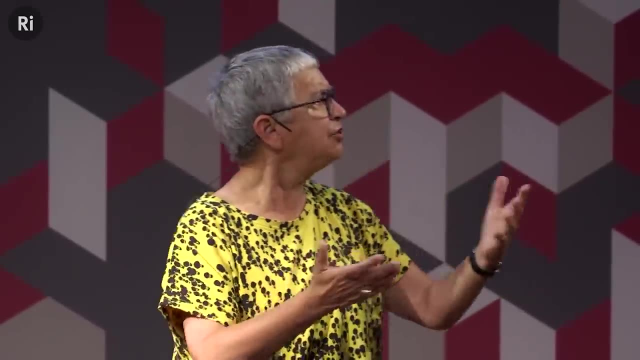 they will recoil and then they change their trajectory. So if I was to look at that from far away, I would say: look at that. there is a strange interaction at a distance that took place. No, no, no, that's not. 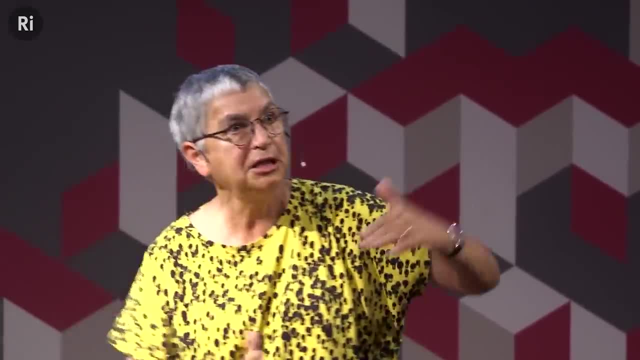 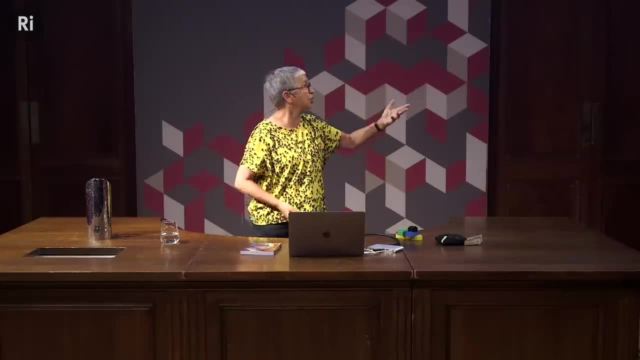 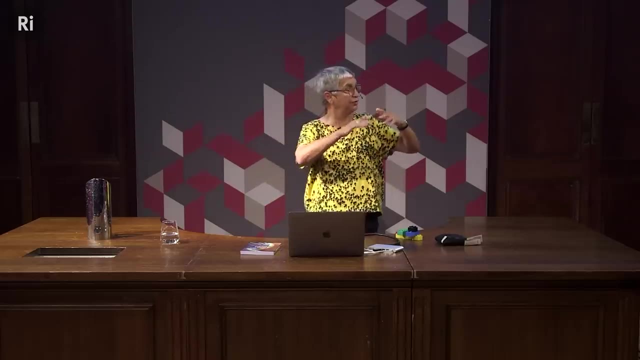 They simply exchanged a heavy boson and it made them recoil. So that's how particles interact with each other. It's by exchanging the various bosons associated with forces. So that's all there is to the standard model in terms of principles. 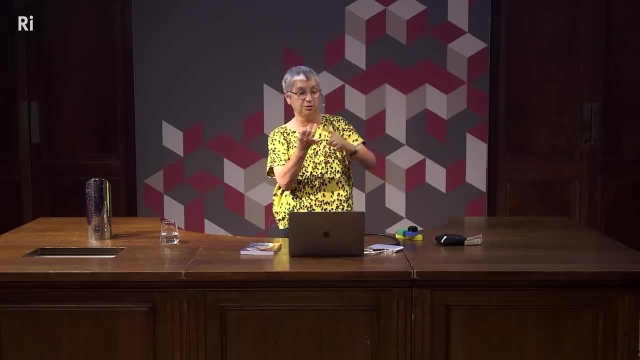 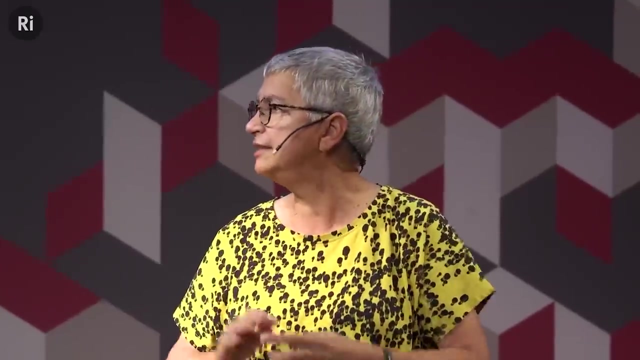 Everything is made of particles, All matter is made of particles, And those particles exchange, interact with each other by exchanging bosons. Okay, so the situation was much clearer than having those 230 different particles that we didn't know what they were made of and all that. 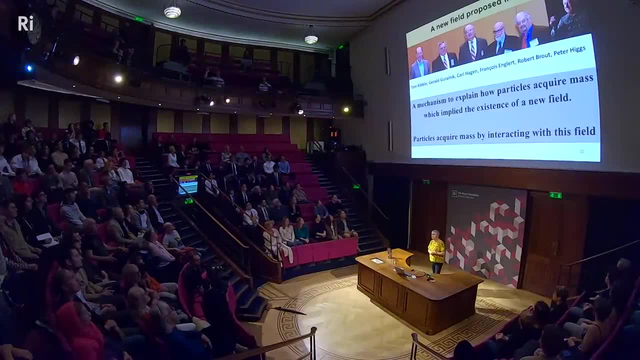 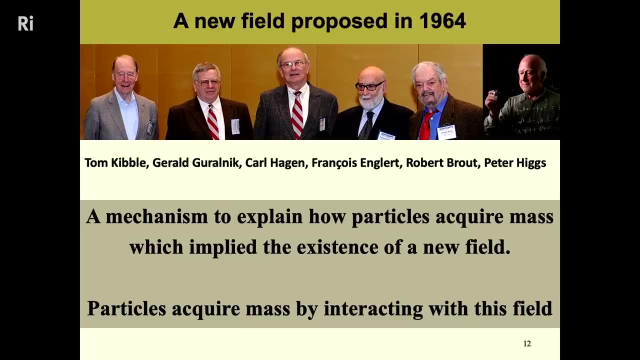 But in the 60s there was a major problem is that all the equations that come with the standard model predicted particles that were massive, But all of them in the equations were coming out with massless particles. All the particles were massless. 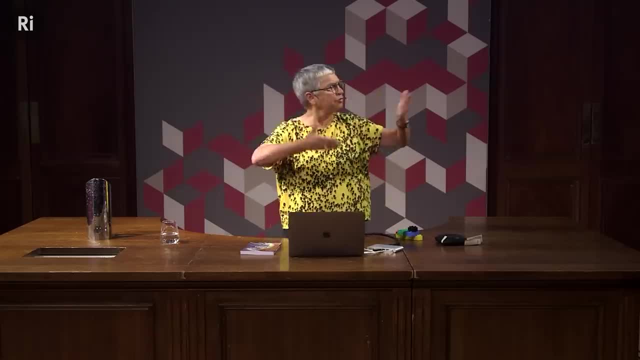 So the model was describing things properly. but all those particles in these equations were massless And we knew we had measured that in the laboratory. we knew that they had a mass. So it was difficult to understand. So a bunch of theorists. 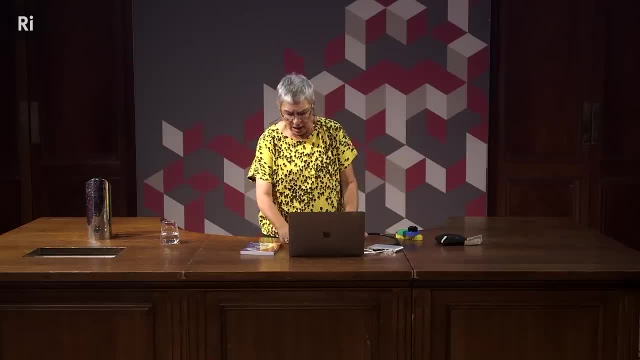 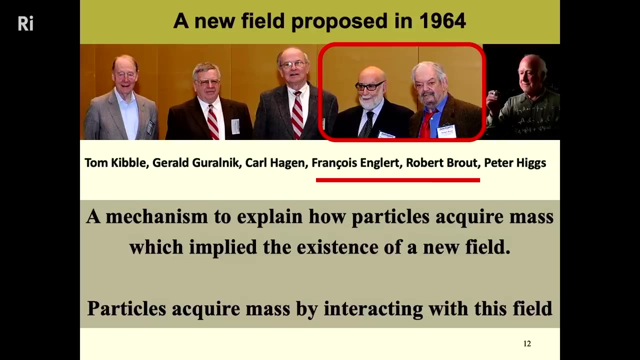 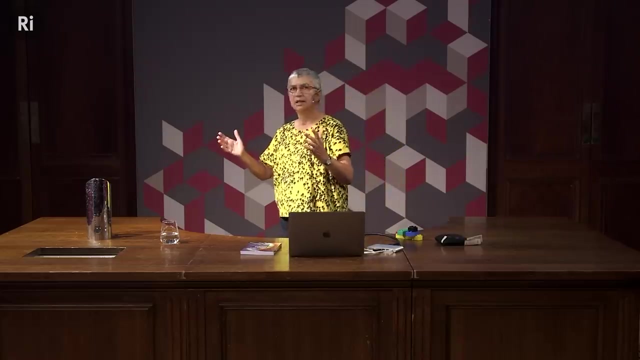 were all working independently, and these two were together, Francois Englert and Robert Braut, two Belgian physicists, and they were the first ones to propose a new field. They said that our universe was permeated by this field. that was, and through this field. 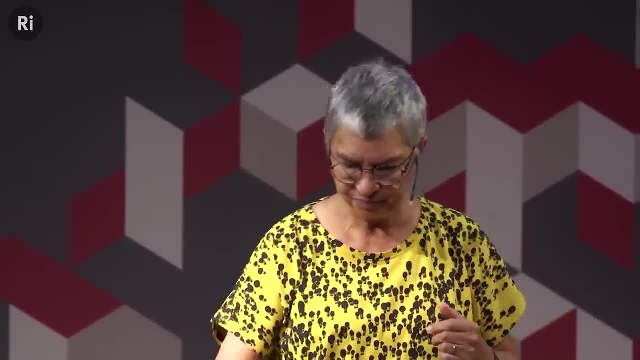 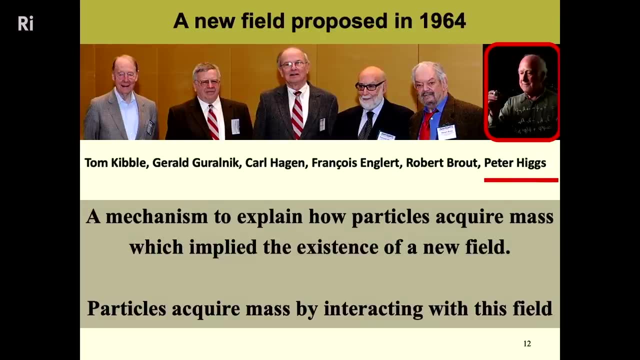 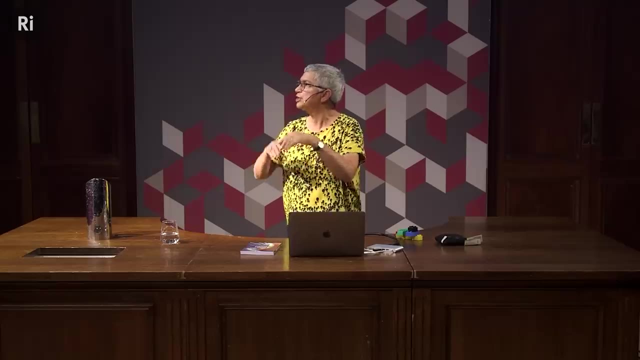 particles could acquire mass. Okay, Strangely enough, those names were until recently not very well known, but everybody has heard now the name of Peter Higgs. Why is he well known? Because he was the second one to publish similar ideas. 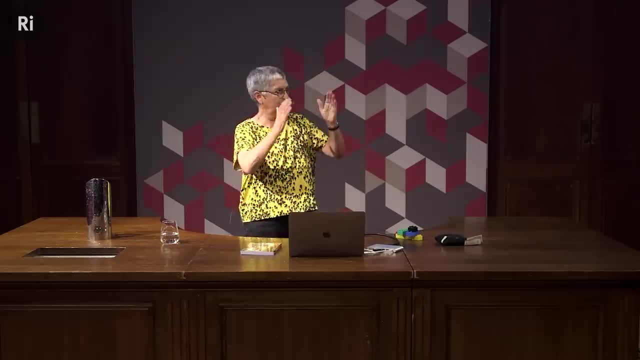 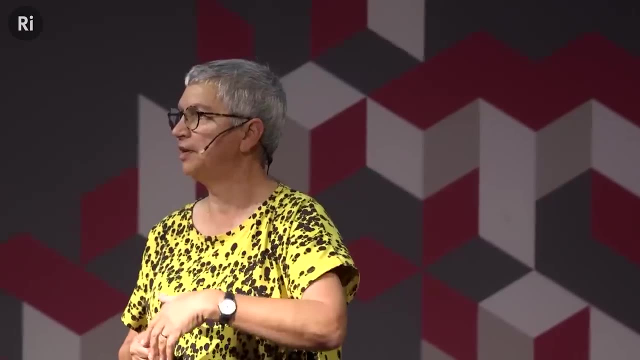 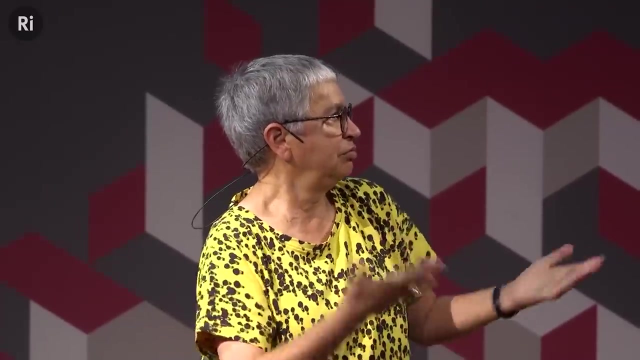 and he sent his paper to a news, to a journal, a physics journal, and the editor rejected his paper saying: useless theory. You don't make any practical prediction with your theory. So useless Higgs was bummed out. 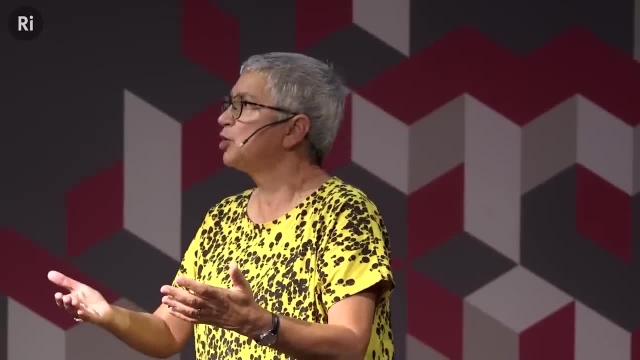 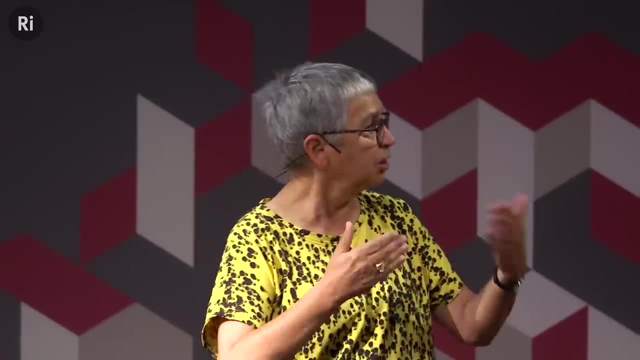 So he said, oui, mais it comes with a new boson. And so he modified his paper a little bit and submitted it to another journal, and then it got published and he was the first one to mention that this new field would come. 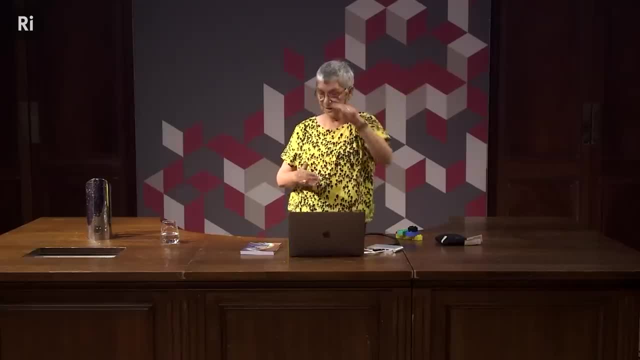 associated with a new boson, like the little Higgs boson that is going around right now. So with this. so that's why the the name stuck being the boson Higgs boson And what they proposed in their theory. 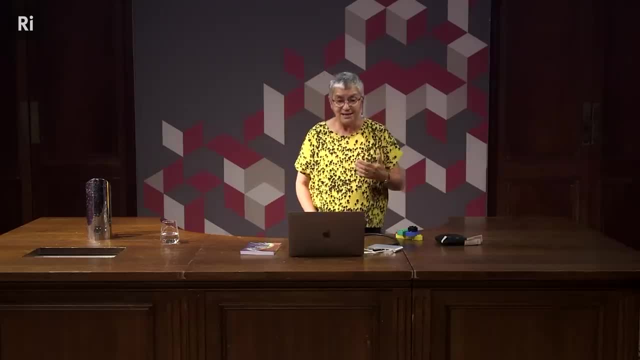 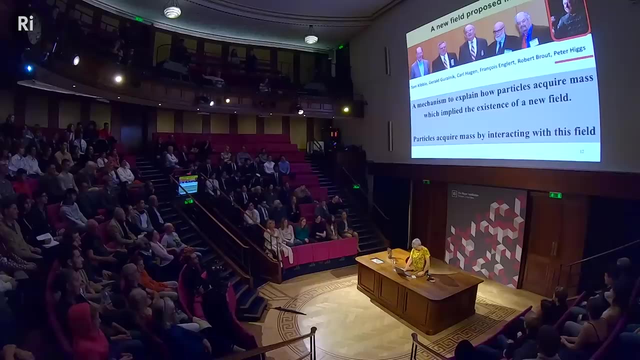 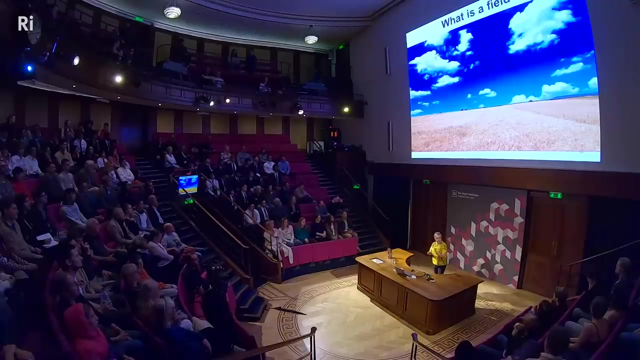 was a mechanism to explain how particles would acquire mass, and, but this required that we would introduce a new field and that particles would acquire mass by interacting with this field. Okay, Now let's try to look at those concepts, one after the other. 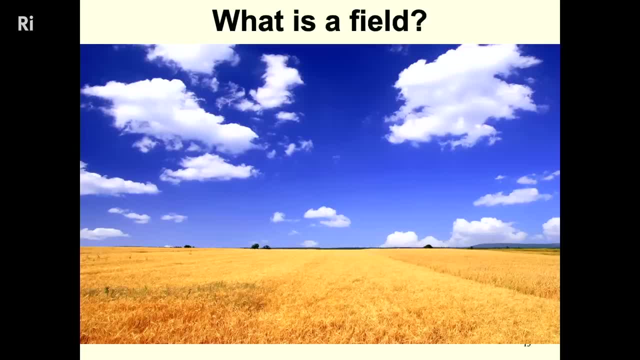 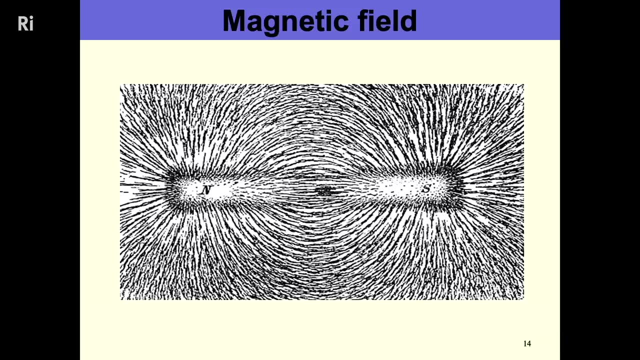 and get somewhere. What is a magnetic field? Well, in physics it has nothing to do with that kind of a weird field. It's more like a magnetic field. You know, if you put a magnet somewhere, it will simply change the properties. 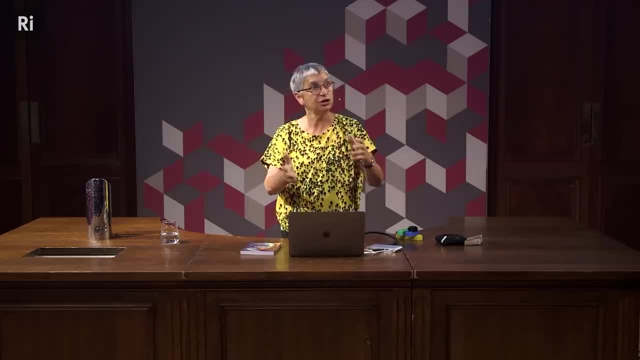 of the space around it such that any, any, any thing that is easily that is reacting to the magnetic force will behave differently. If I have a magnet here and I put a a piece of plastic and then I with a salt shaker, 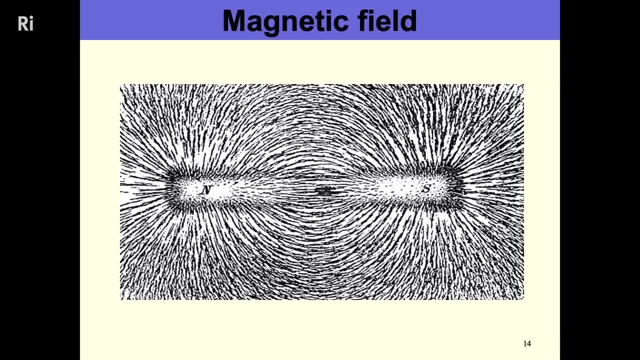 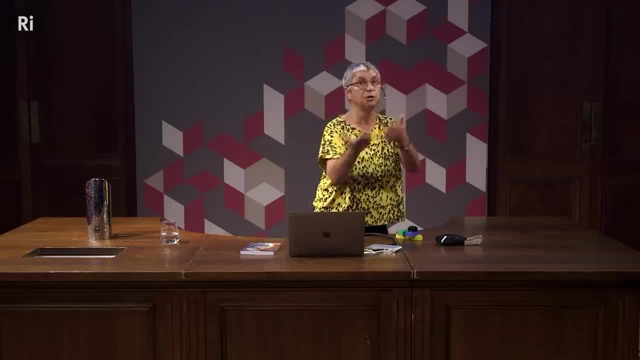 I put some iron filing on it, all the little pieces of iron filing will align themselves around in the direction of the magnetic field line, around the magnet. So those iron filings grains will all behave differently in the presence of a magnetic field. When there is a gravitational field, 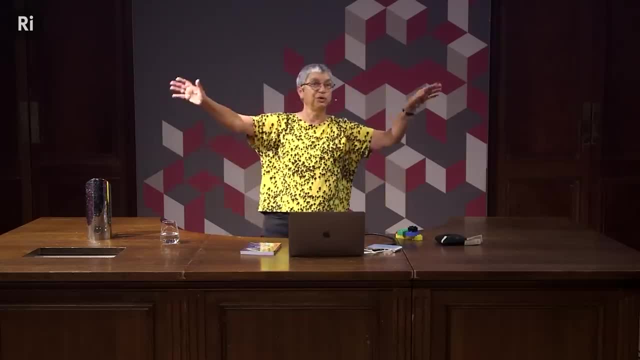 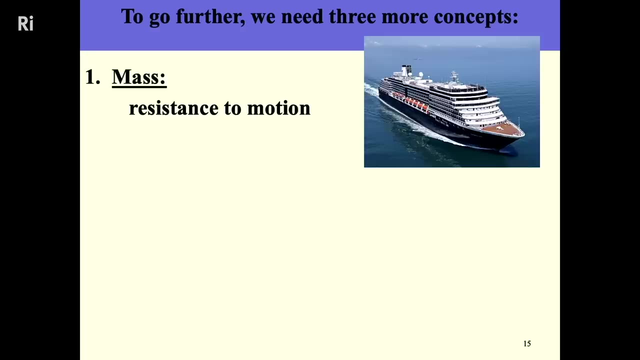 we stick to the ground. You know we don't float around, Okay, So keep that in mind. Now I will go and introduce three concepts that we use in physics: Mass- What is mass? Mass is the resistance to the change of your state of motion. 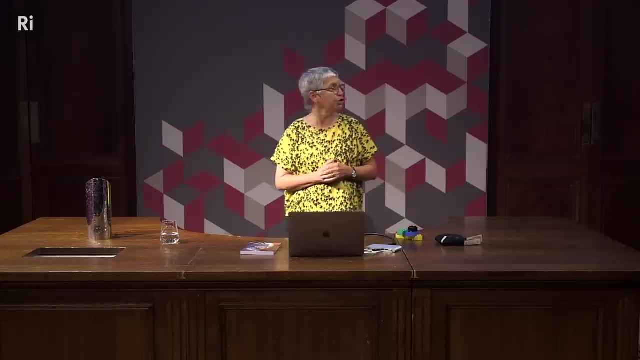 So say that you are a huge cruise ship like this and it's, it's in motion. If you want to stop it, it will take a lot of energy because it has a lot of mass. So to it will offer resistance. 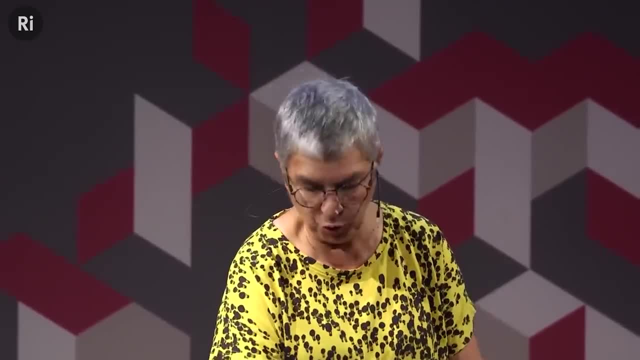 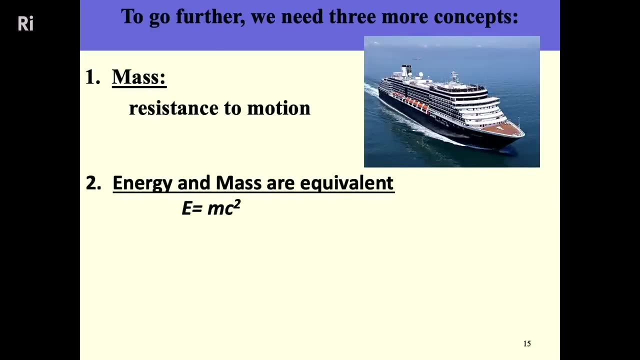 to the change of its state of motion. Likewise, when you want to put it in motion, And energy and mass are equivalent. The equivalence between energy and mass is well known with this equation is represented by this equation: E equals MC squared. 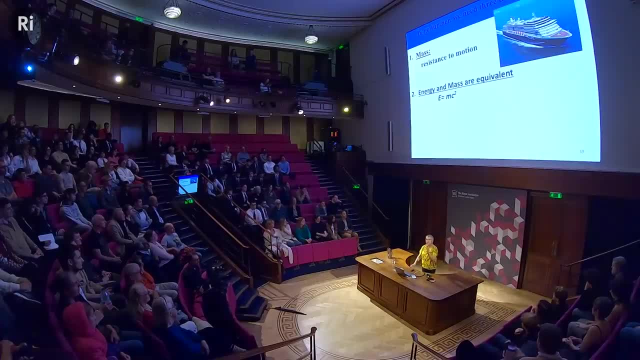 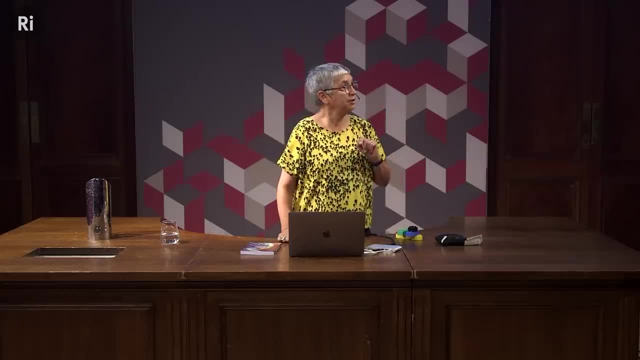 You've all heard that equation at some point. E represents the energy and M the mass. C squared is simply the square of the speed of light, And that's the conversion factor between energy and mass. This equation tells me that I can take energy. 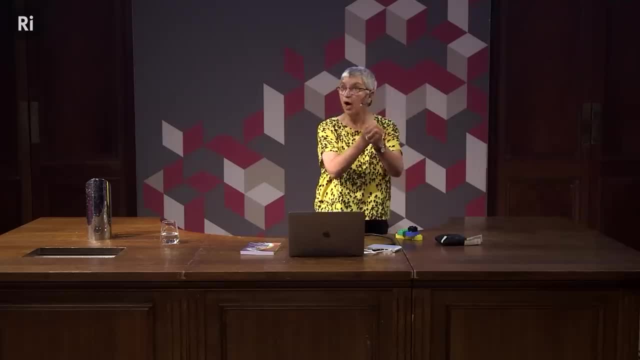 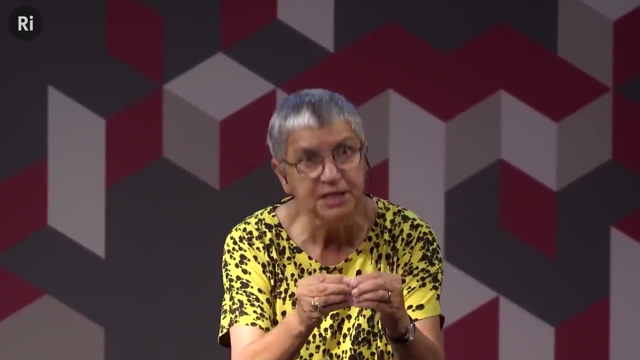 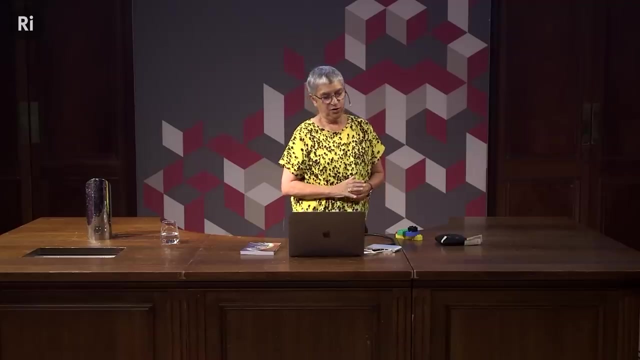 and produce matter mass out of it. That's what we do at CERN, when we concentrate a lot of energy with the accelerator in one tiny point And we make new particles appear there And you can take mass material and you can. 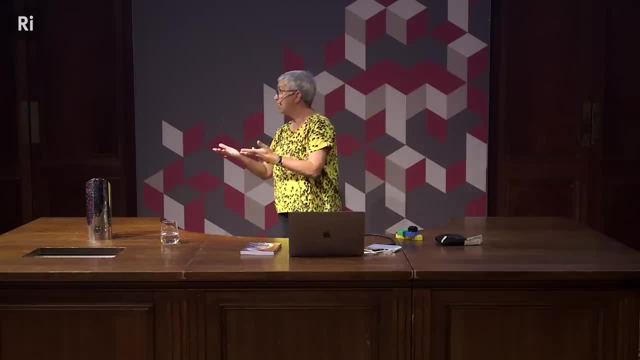 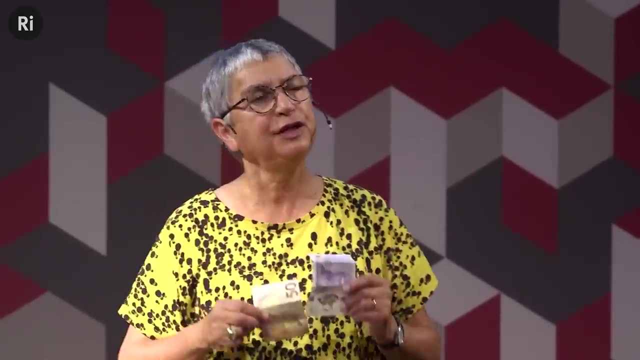 break it apart in a nuclear reactor and produce energy. So the two are equivalent. You can look at mass like being congealed energy. Okay, And mass and energy are just two different manifestations of the same essence, Like here, You know. 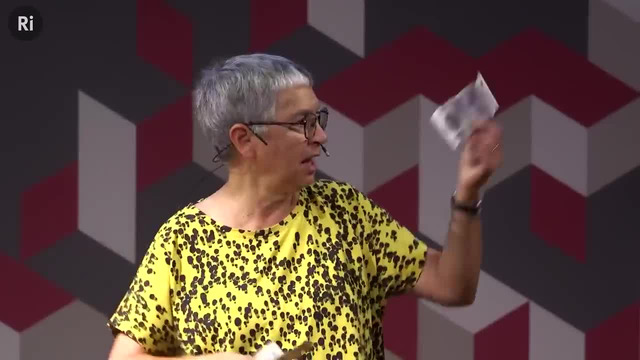 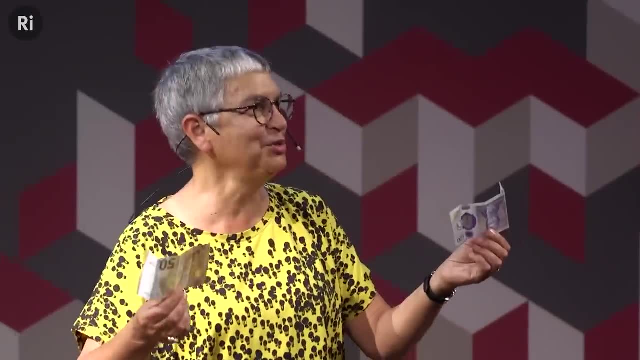 I live in Germany, so I have euros in my pocket. normally I'm here today so I have pounds, but I don't know why, because everybody only uses credit cards, so it's totally useless, But anyway. so I have pounds and euros. and there is a conversion factor. So it's not the same thing, but they represent the same essence, which is money, And there is a agreed upon exchange rate between the two. And that's the same between energy and matter and mass. 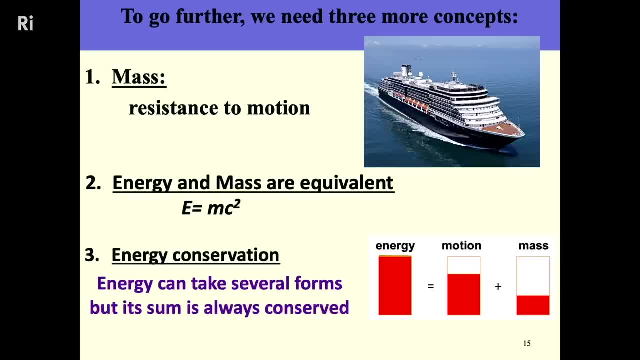 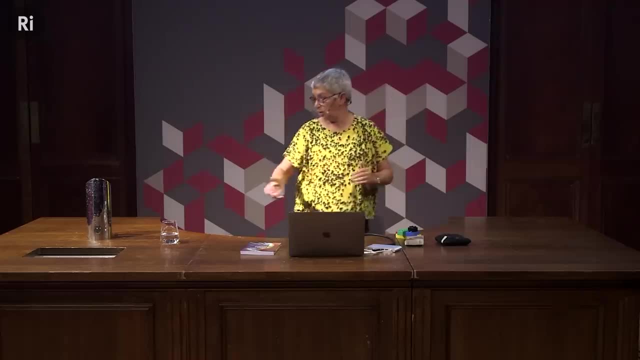 Third concept: energy conservation. Energy can take different forms, but must always be conserved. You cannot just lose energy like this. So if I represent energy with a fluid that I have in a bottle, I can then take my quantities of energy. 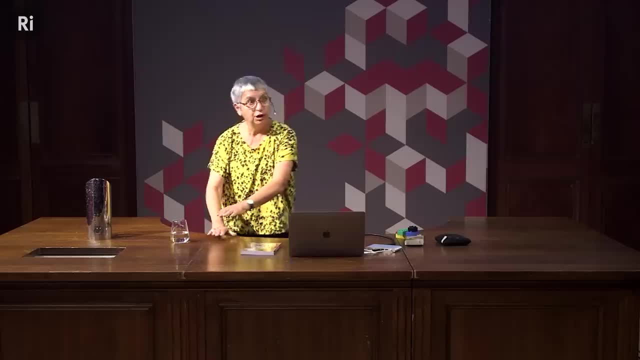 here and pour it in two different containers, but the total amount of fluid that I have at the beginning will always be the same. Just don't have to spill. It's okay. You're not allowed to spill. That's a thing For a fundamental. 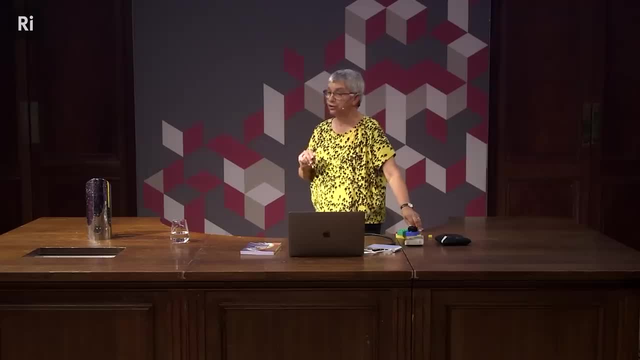 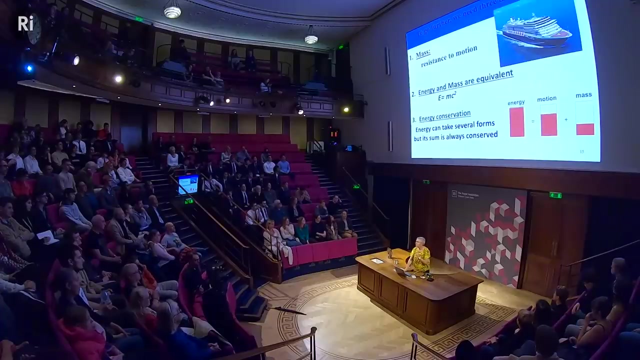 particle that is moving, there is only two ways that it has energy. It has energy due to its motion, kinetic energy- and it has energy- congealed energy, in its mass. Okay, Okay, Ready. Here is how the Brout-Endlert-Higgs field 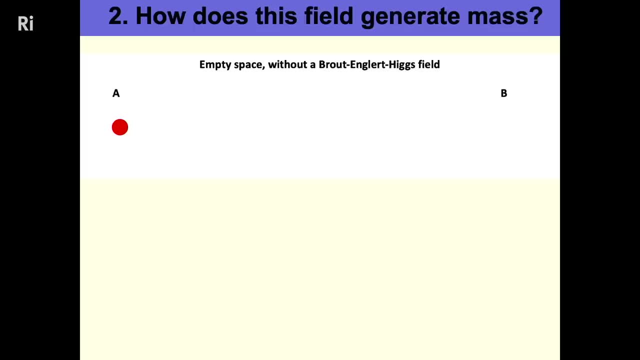 gives mass to fundamental particles. Let's go back a little bit back in time at the time just after the Big Bang, But we don't have much time. It lasted less than 10, to the minus 25, 30 seconds where there was. 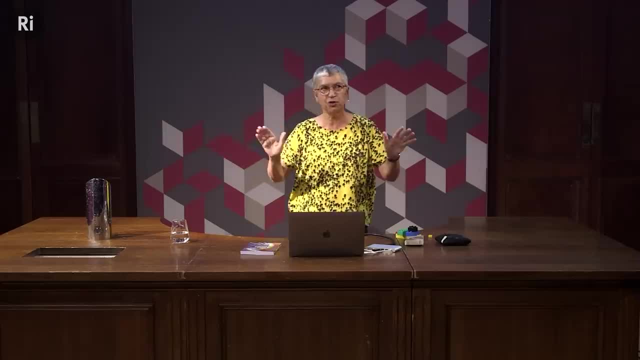 absolutely no Brout-Endlert-Higgs field. then There was no time. There was nothing before the Big Bang. I'm told I wasn't there. But so imagine that a particle wants to go from point A to point B. 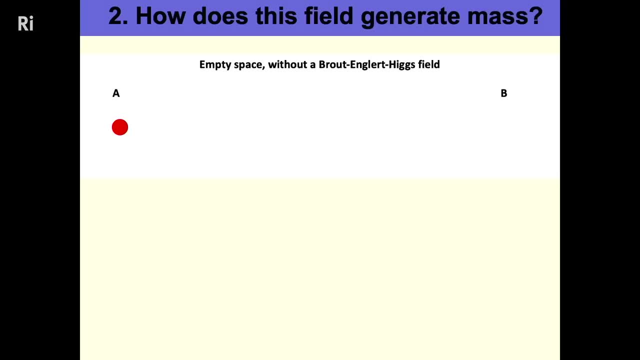 There is no Brout-Endlert-Higgs field, and then the space is empty and the particle can go from A to B on a straight line at the speed of light, because it's massless. Huh, So only massless particles can travel. 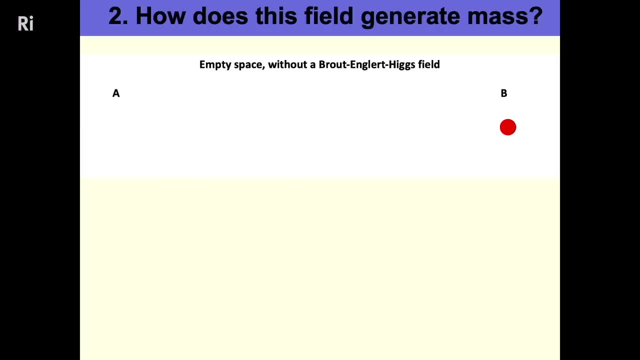 at the speed of light. Do it slower so you can see It's going on a straight line. So for this particle, which is massless, all its energy is in the form of motion, kinetic energy. It has no mass. So the mass 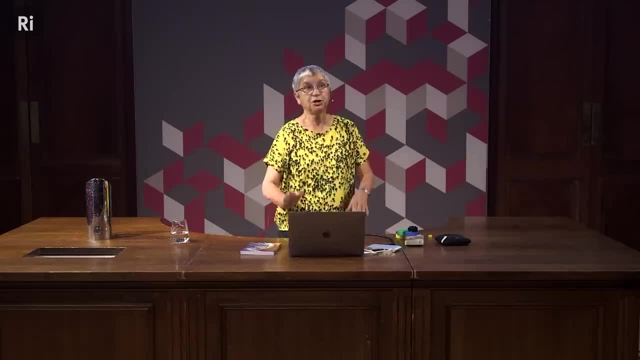 container is empty, But something like- sorry, I forgot it was 10 to the minus 32 seconds. shortly after the Big Bang, someone or something turned on the Brout-Endlert-Higgs field. And now the space, the properties. 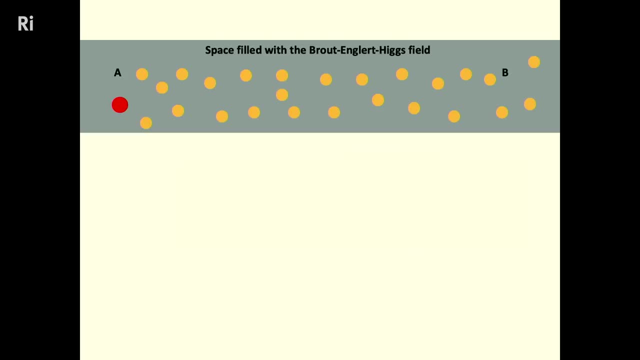 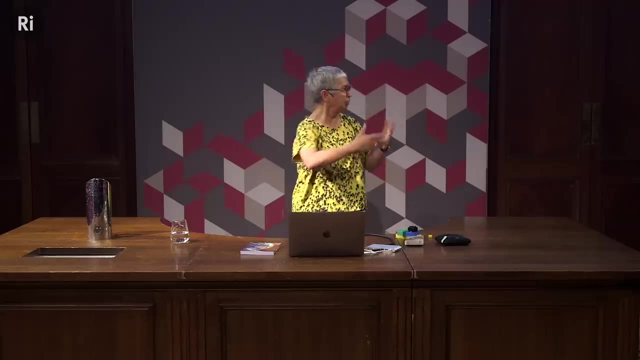 of the space were modified And it made it like it's like in the previous case. it's like a kid wants to go across the schoolyard and when the schoolyard is empty, the kid can easily run at full speed on a straight line. 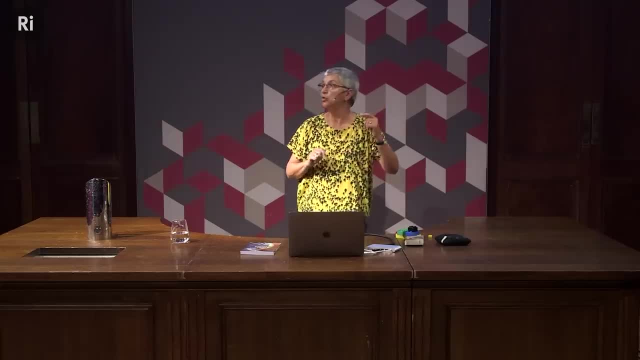 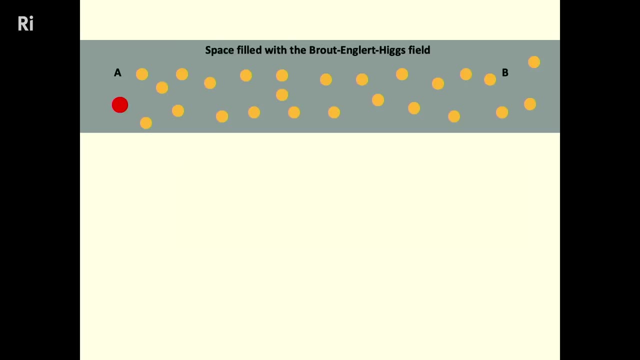 But if that kid is trying to cross the schoolyard when all the kids are out at recess, then it will start interacting, you know, saying hello to the friends and bumping into each other, And it no longer goes on a straight line. 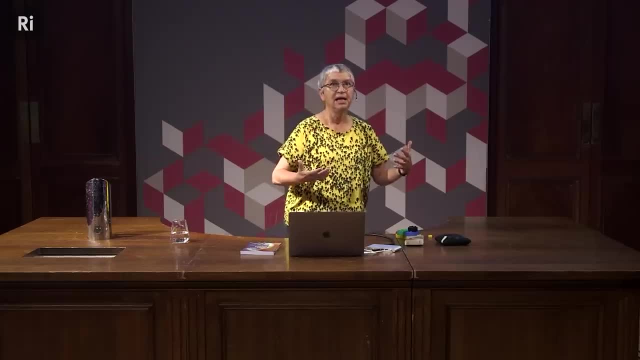 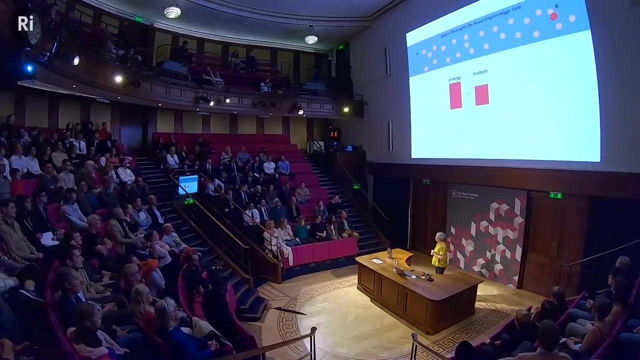 It interacts with the space around it. It starts getting its feet caught in the carpet, in the flowers of the carpet, like my grandmother would say. So you've noticed this particle is not going as fast as it was before, So it has less kinetic energy. 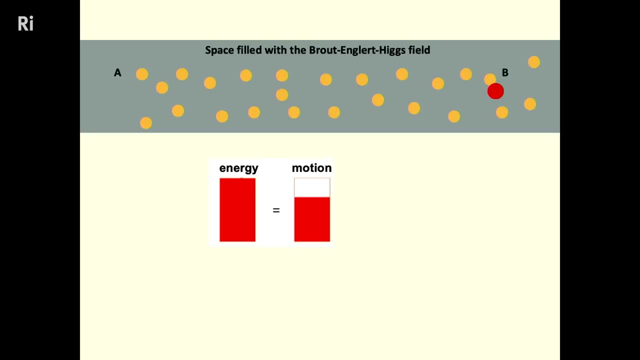 You all agree with me. Where did the missing energy go? Yes, that's it. So this particle acquired mass by interacting with the Brout and Laird Higgs field. Ta-da, That's how it works, And it's only this way. 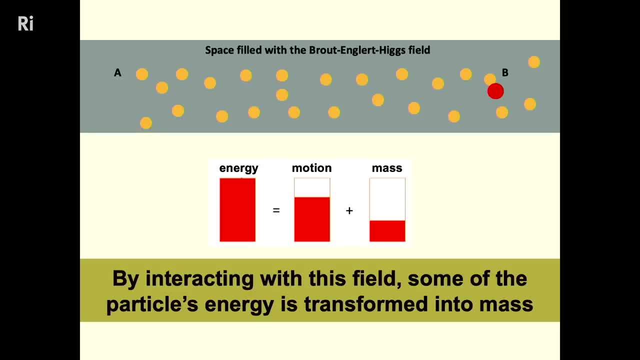 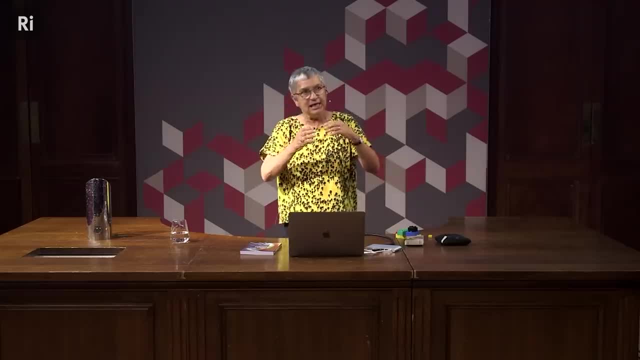 that the particle would transform some of its energy into mass. Then you will have congealed energy in the form of mass. Sometimes an image that is given is that it's like the space becomes viscous and the particle cannot move so easily. It's good. 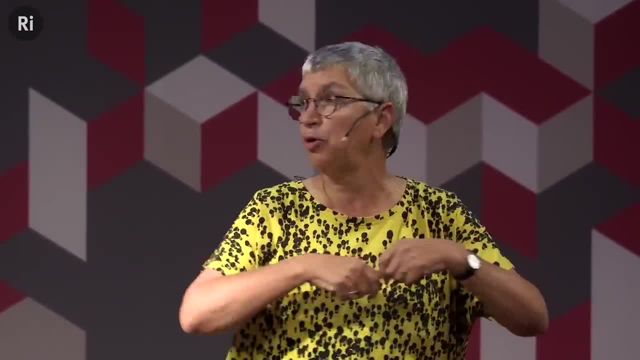 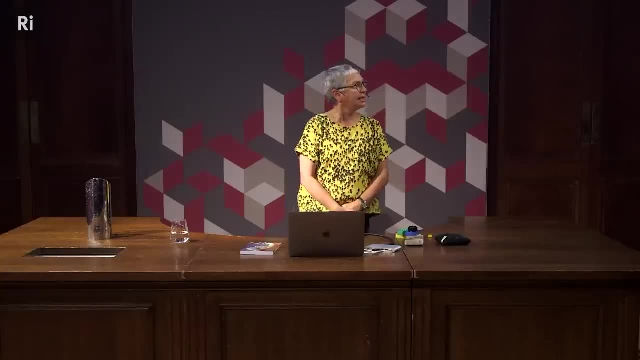 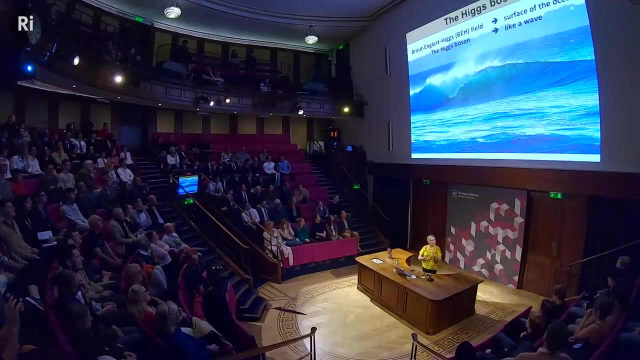 for an analogy. but then viscosity is something that is dispersive of energy by friction, and that's not the case here. Did you notice that I haven't said a word yet about the Higgs boson in that whole story? So Brout and Laird. 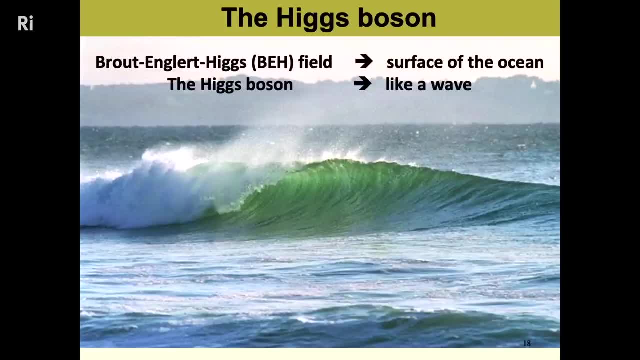 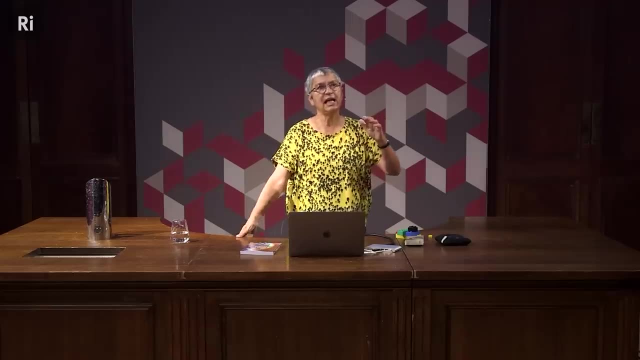 and Higgs independently, all came up with the same idea and the three other guys who were in the picture that I forgot to mention that there was this field and I would say that the Brout and Laird Higgs field. we could make an analogy with the surface. 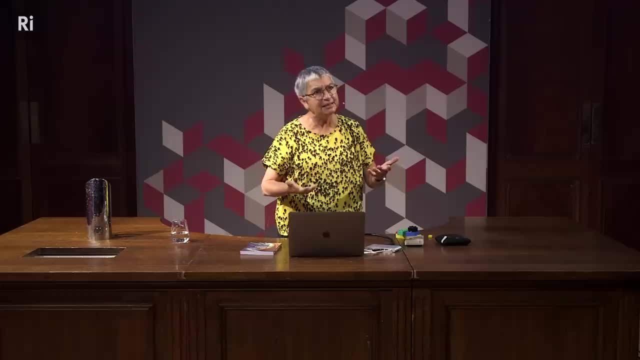 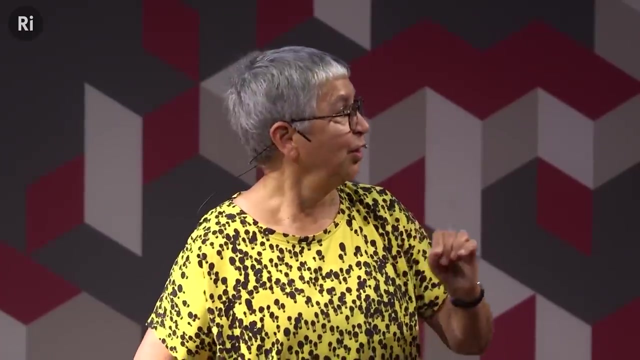 of the ocean and you know that we can excite the surface of the ocean either with the wind or an earthquake, a tsunami, and then you can produce waves. So the Higgs boson is like that: It's just a wave at the surface of the 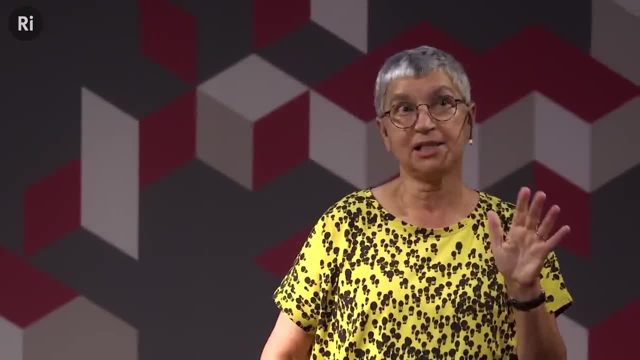 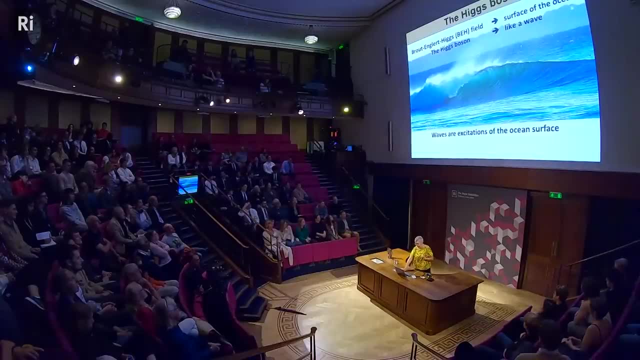 Brout and Laird Higgs field. Now you can all ask me: where did I get my drugs? It's pretty good to come up with those things. It's pretty far off, but that's the way it is. Waves are excitations of the ocean. 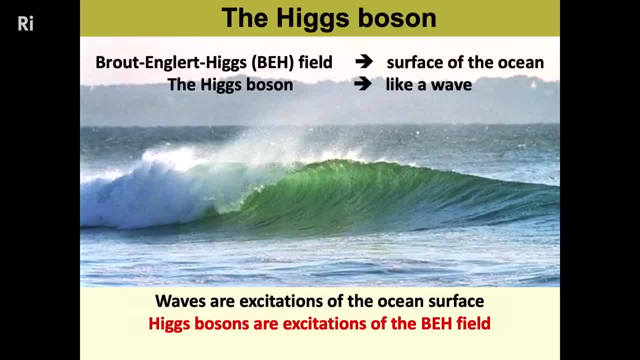 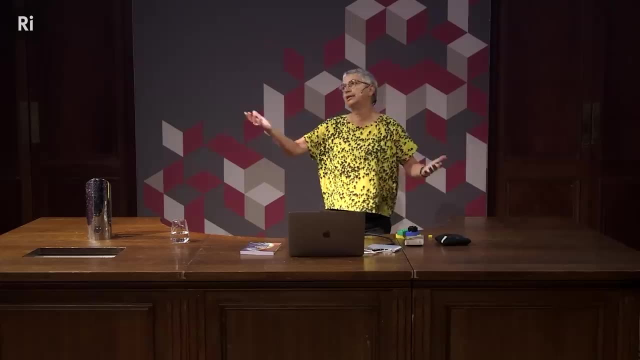 surface and the Higgs bosons are excitations of the Brout and Laird Higgs field. We can create Higgs bosons by exciting the Brout and Laird Higgs field. Of course I'll say: come on, now she's full. 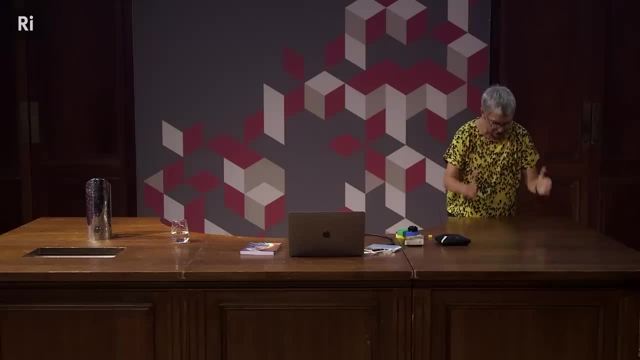 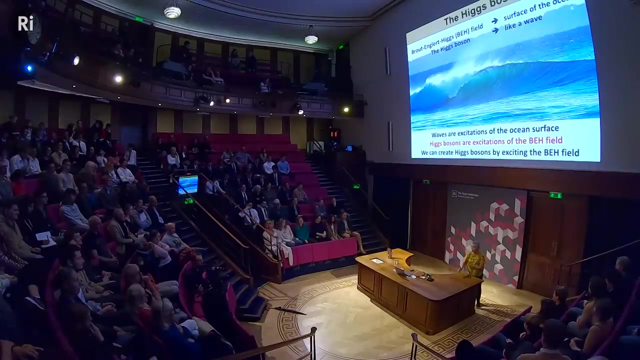 of it. What is this? And so to prove it to you, it's like imagine that I have an aquarium here and I tell you the aquarium is full of water. Can you see the water? No, Okay, so to convince him and all of you, 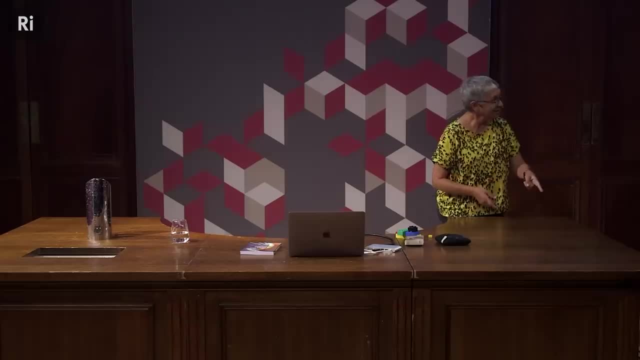 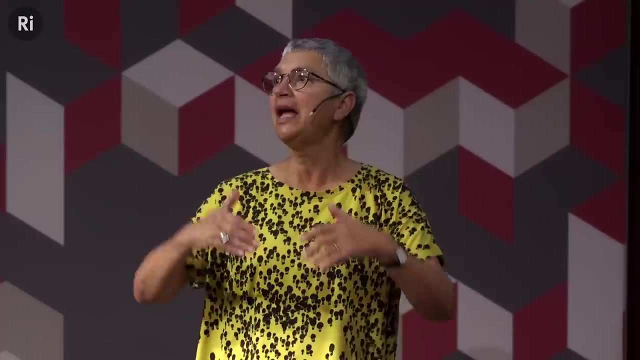 what I can do is easy. Huh, Did you see it? Okay, No good drugs for you, So okay. So all that we had to do, us particle physicists, experimentalists at CERN, was to go and excite the canvas of the universe to make Higgs boson. 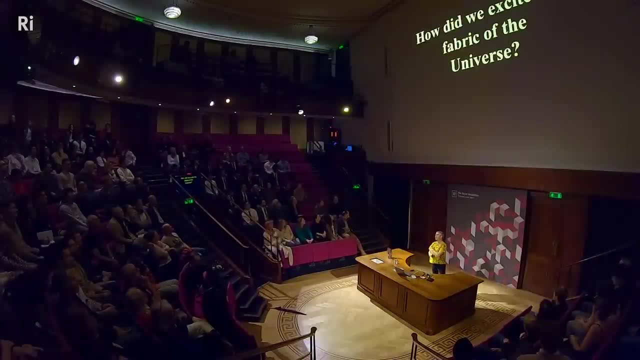 And that's what we did. But how did we excite the fabric of the universe? You know that's the job we were given. Okay, go and excite the fabric of the universe. Sure, What time would you like that? 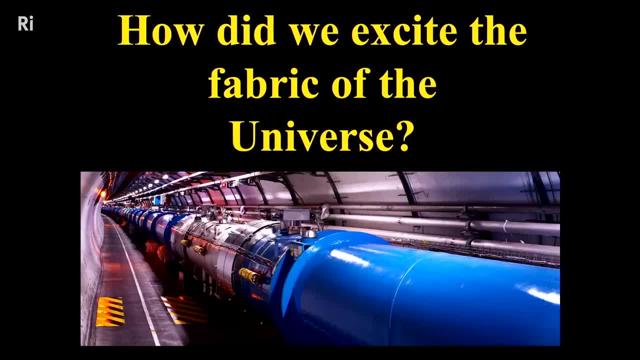 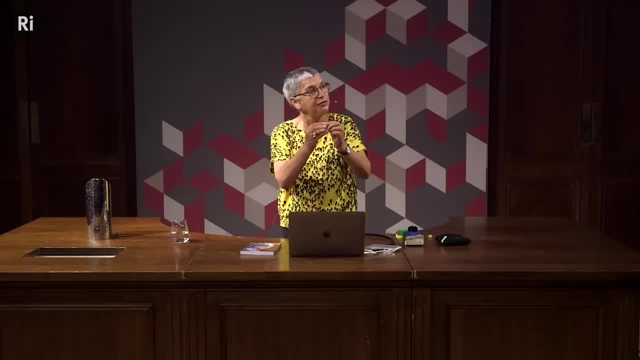 And so what we did was to do it with the Large Hadron Collider, And this is a very energetic machine that can put a lot of energy in one tiny point in space, And this energy can resonate with the fabric of the universe And then, when you just give it the right energy, like a string of guitar. 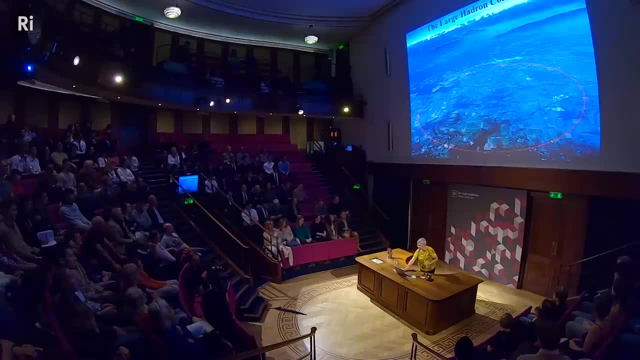 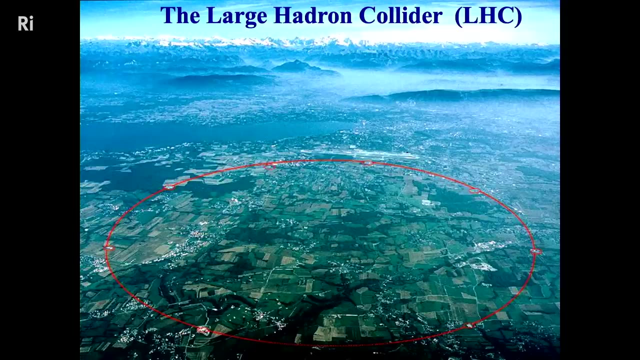 it will start to vibrate. That's exactly what we did. That's exactly what happened. So the Large Hadron Collider is built at CERN. CERN is the largest particle physics laboratory in the world. It's near Geneva, in Switzerland. 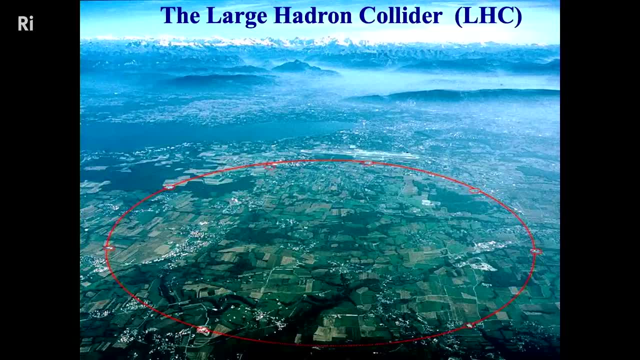 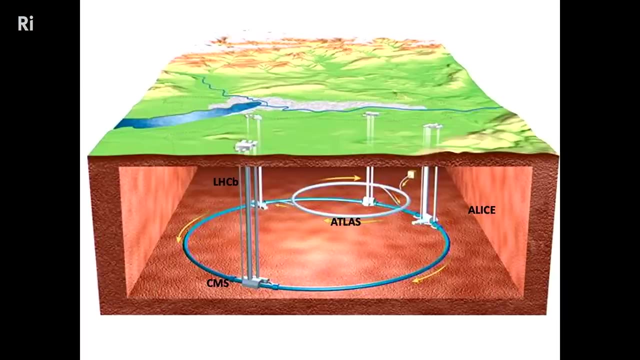 And it's very large. It's 17 miles in circumference, 27 kilometers around, And you don't see anything. but the four experiments are built along this tunnel, but 100 meters, 100 meters underground, So 100 yards underground. 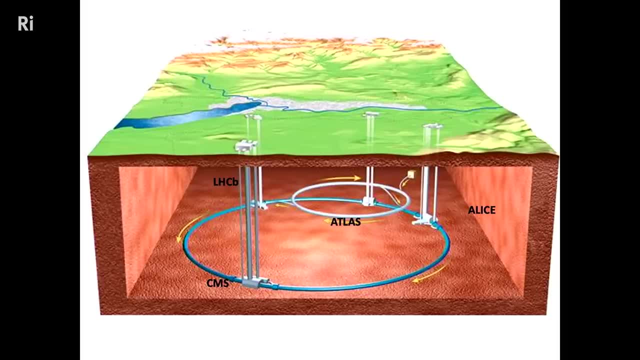 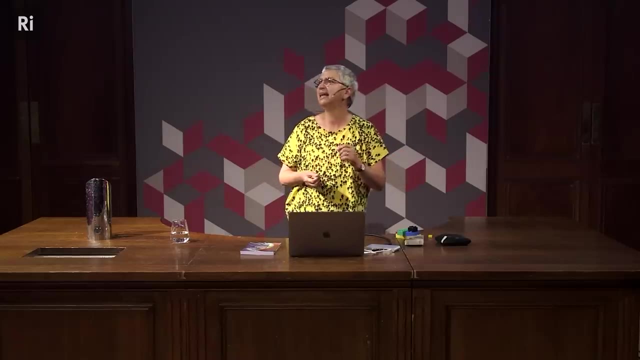 And there we have huge caverns that have been excavated and a tunnel that looks pretty much like a subway tunnel, in which we have a vacuum pipe and we have protons that are accelerated near the speed of light- It's at 99.99997% of the speed of light- and we have the particles, the protons, that circulate. 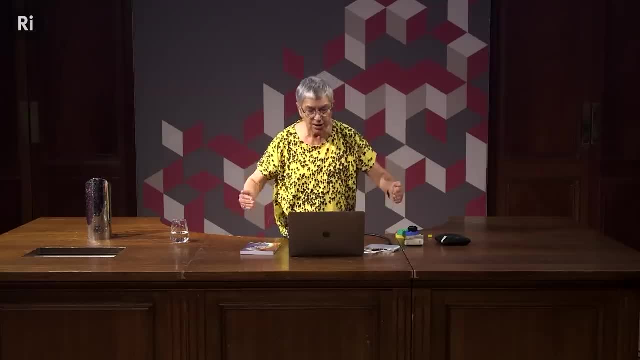 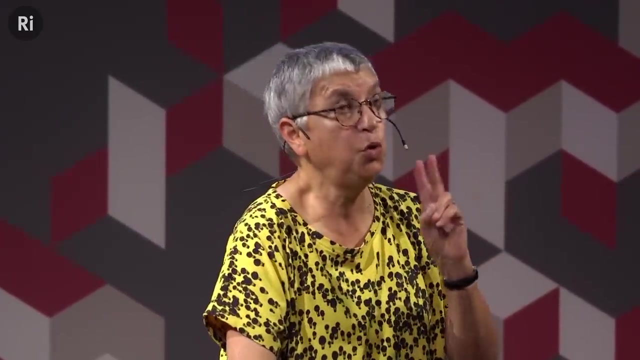 in the accelerator, like that, 27 kilometers, And then they come and they collide. We bring them into collisions And then of this collision the energy materializes and produces new particles. So we have two types of tools to work at CERN. 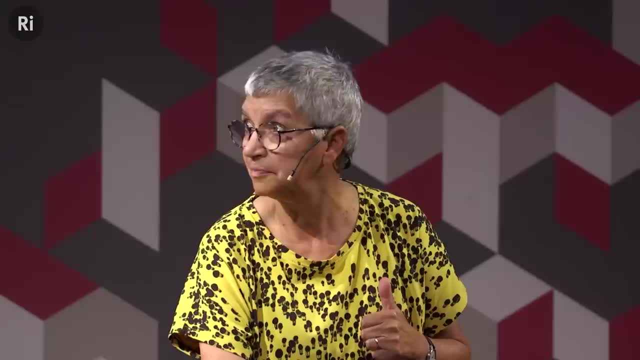 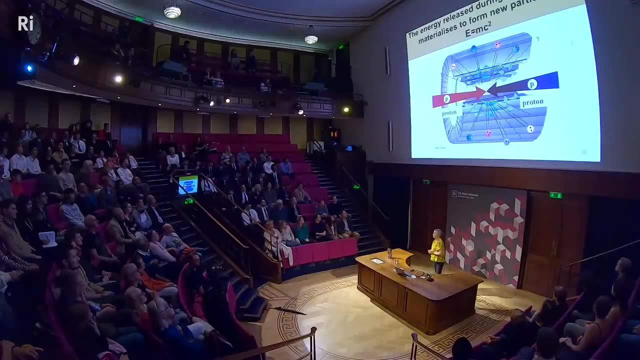 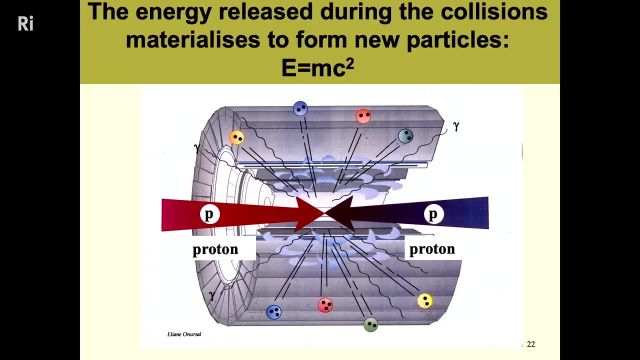 We have accelerators that accelerate particles and we have detectors. and guess what they do? They detect the particles that come out. So we produce those collisions. new particles form right there, but they're very unstable. they break apart and they create like mini-fireworks and all the fragments fly apart and they go. 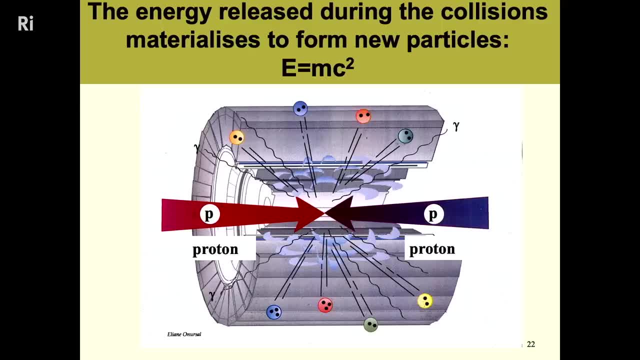 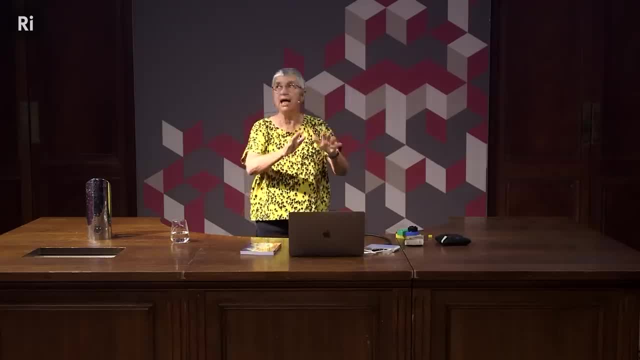 through the different layers of our detector, which are huge cylinders with end caps, And it goes through all the layers and leaving signals everywhere, and then we can tell that, yes, we saw something. It looks like a mini-firework and we're trying to catch all the fragments that come. 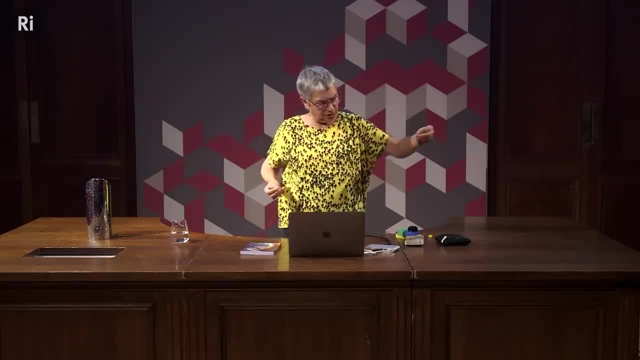 out, and then we can reconstruct what was created at the first to start with, and then analyze what kind of particles can be produced and how do they decay, and all that, and from that we infer the various laws of the universe. So that's what we're trying to do. 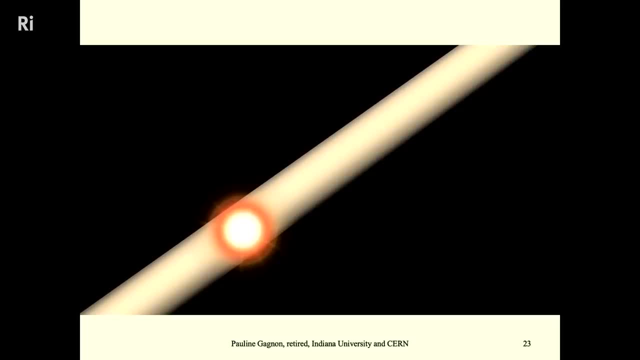 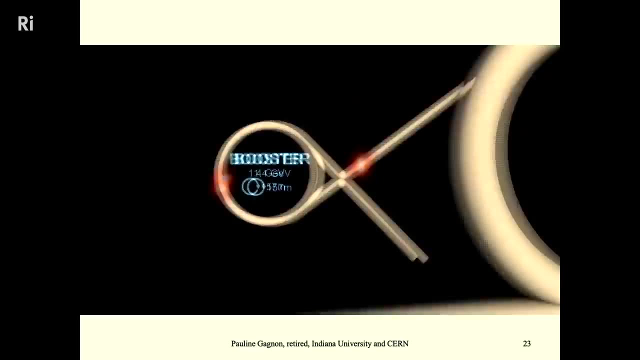 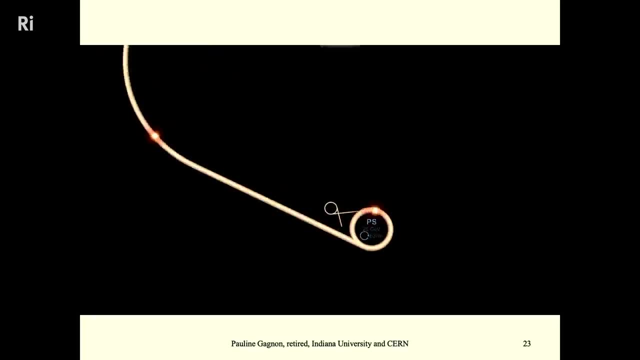 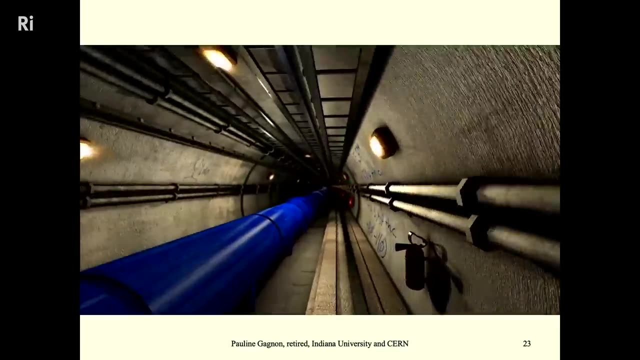 They gain enough energy, They go to the next stage, which is about 630 yards around, And then they go in a larger one that is about 5 miles around, and they gain more energy at each step until they get in the LHC- 27 kilometers or 17 miles. 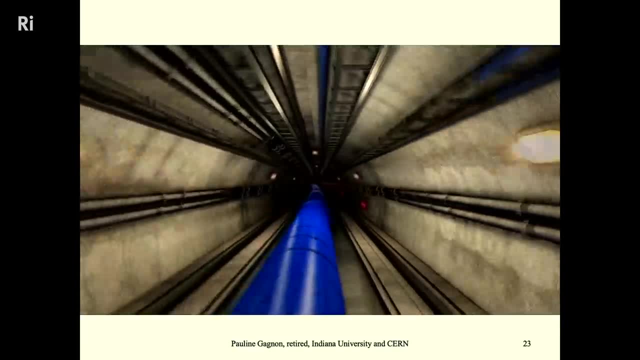 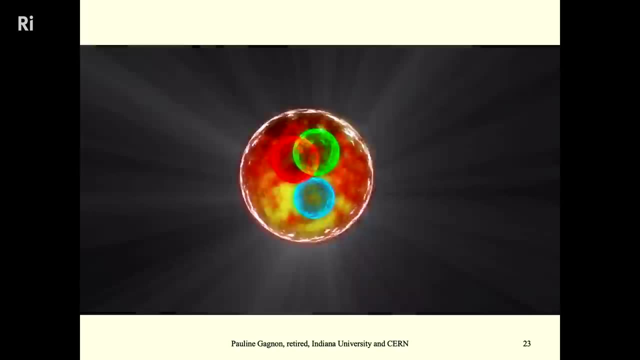 And they go and circulate. They go through this vacuum pipe accelerated by electric fields, and we have huge magnets that will bend them around to keep them on the circular orbit. You see the three little quarks are a bit excited. before action: 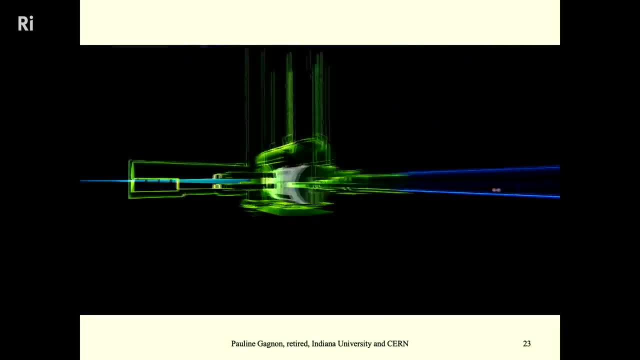 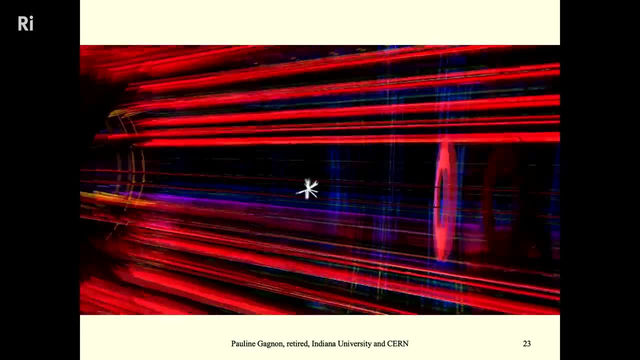 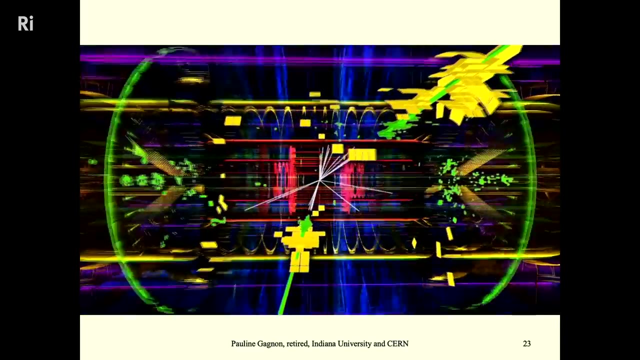 And then they come from both ends. we send them in two directions and then they come smack in the middle of where we put the detectors, and then they collide. energy materializes in the form of various particles and we try to catch all fragments to tell what happened. 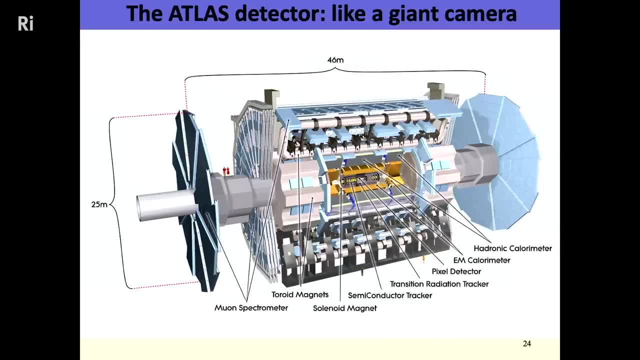 And so we do that happily. and our detector is built: it's like a giant camera, except that it's a pretty good one. We have collisions, And every 20 nanoseconds, 20 billionths of a second, we have collisions. 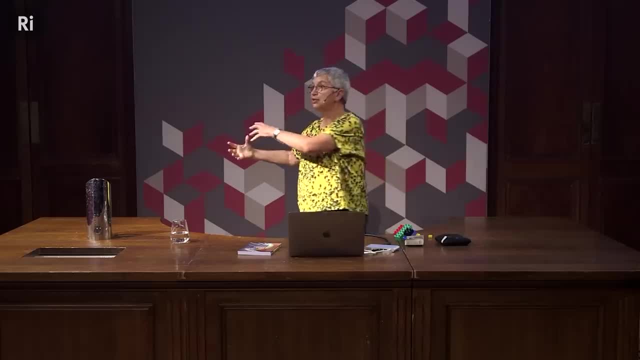 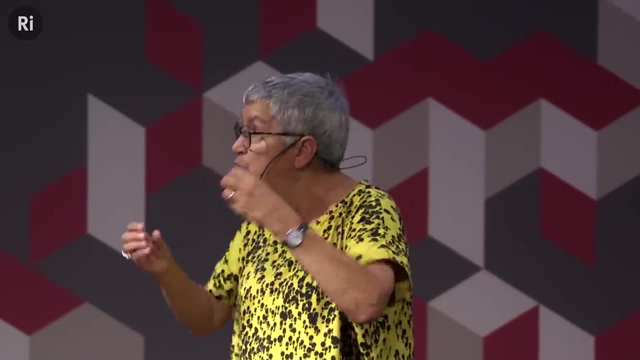 And it's not only one proton coming here and one there, but it's a huge bundle of protons in one side, same with billions of protons, like bee swarms, and they come and they collide, And sometimes there are more than one collision at the same time, and so it gets really difficult. 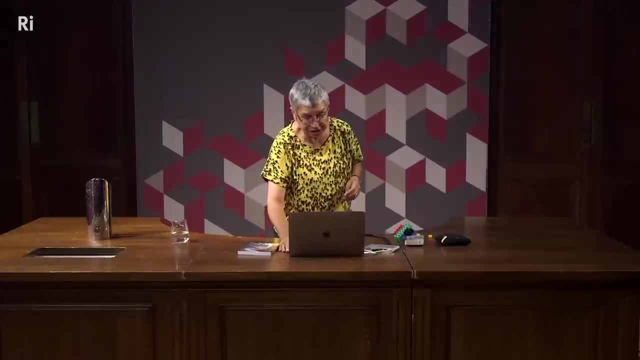 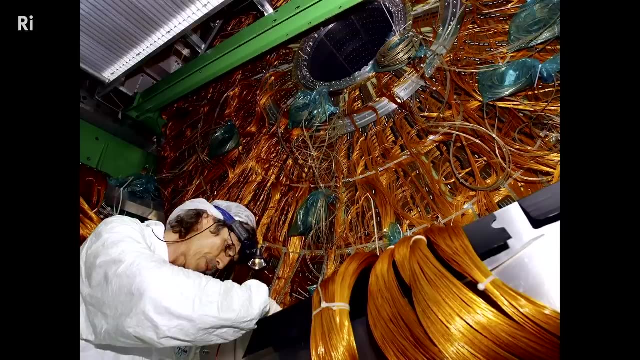 to disentangle all that. It's a huge machine with 4,000 kilometers of cables. Here, if we're looking at the calorimeter from Atlas A, calorimeter is a layer that is there to measure the energy that each fragment had. 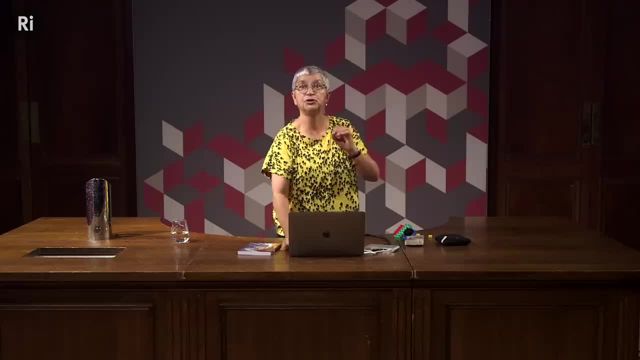 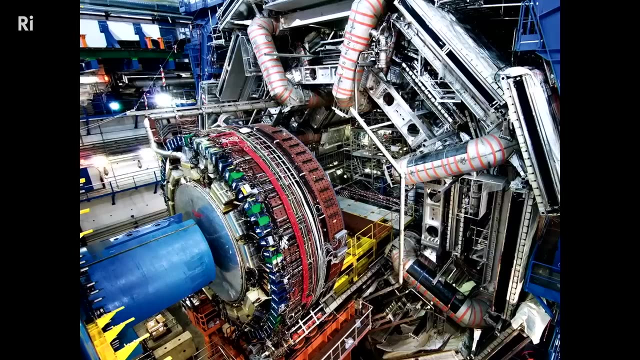 So we have 4,000 kilometers of cables and 4,000 kilometers of tubing with cooling fluids and various gases. The whole detector is few. It weighs 7,000 tons. That's the weight of the Eiffel Tower. 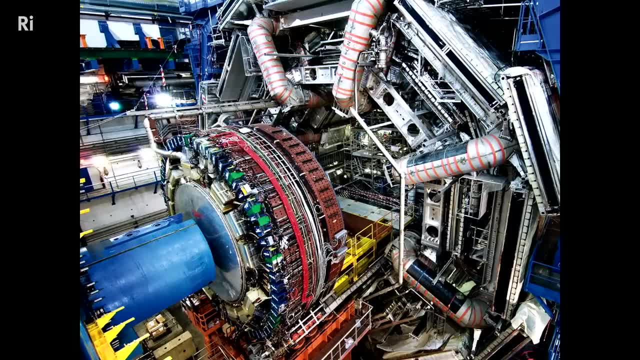 But the Eiffel Tower is just rusty steel, Whereas here, like my friend Monica Dunford said in the movie Particle Fever, it's like a Swiss watch on steroids. Everything is done with ultra-precise little detectors, all built by hand, assembled by hand, 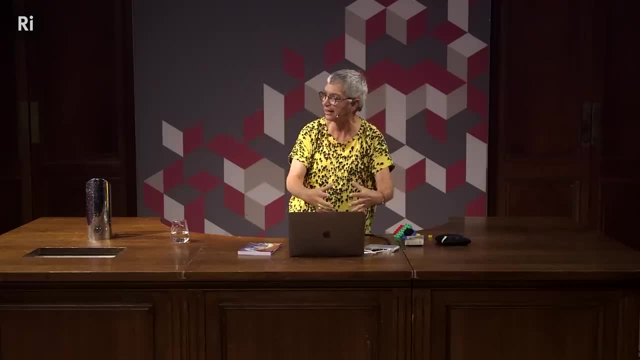 And for the Atlas detector, we built it in the cavern, like we build a ship in a bottle that cannot come out of the lair, And it's six stories high. So here is what we call the muon wheel. So it's a detector just to detect muons. 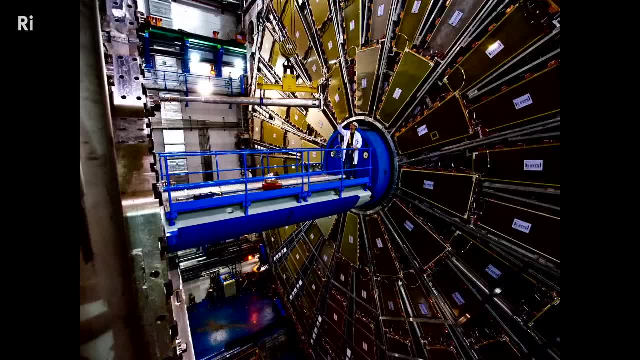 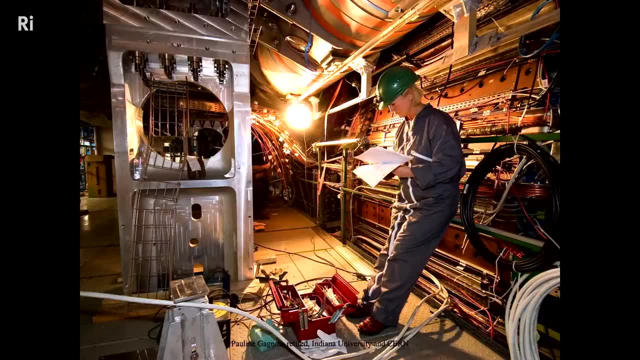 I'll show their role later, And it's a hell of a time to make a good selfie there. The big question is how we turned on the detectors and all that and it all worked. It was so amazing. The accelerator, the four detectors. 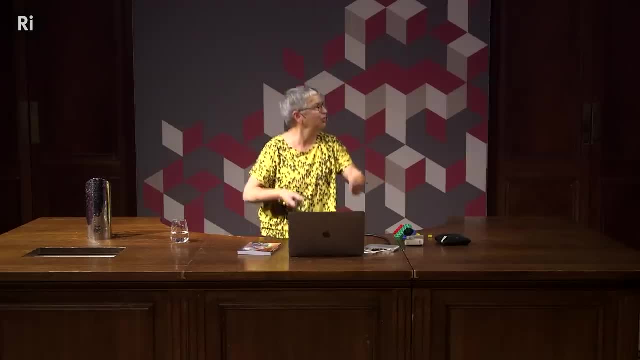 Of course, we had done some tests and all that, but the one day when we turned everything and it worked, it was amazing And it took about 20 years to build all that concept and all that. So how did we manage to make it all work? 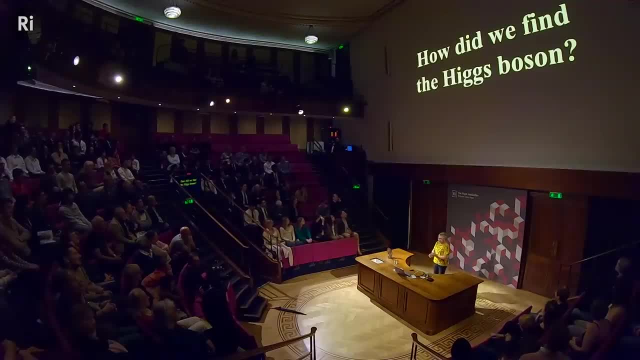 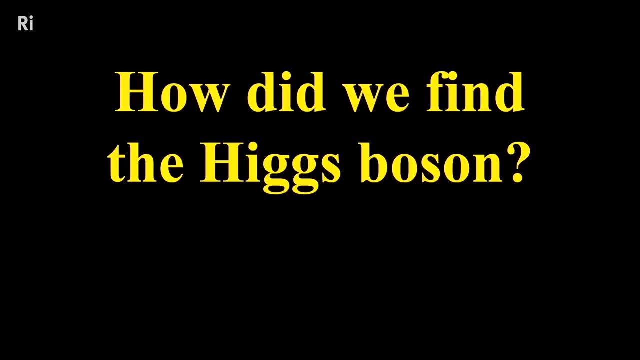 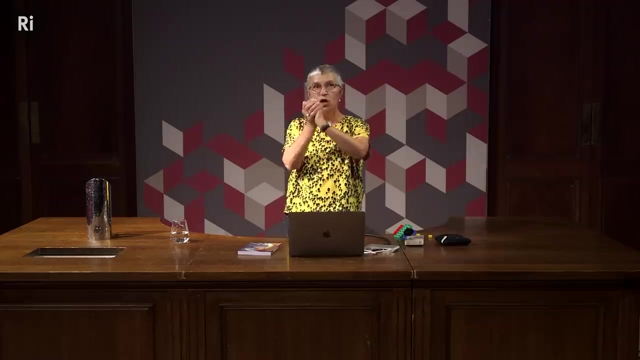 It's a mystery. But let's go back to our Higgs boson. How did we find the Higgs boson? So we excited the canvas of the universe, produced that very unstable particle which broke apart. But I was telling you earlier that those particles were fundamental particles. 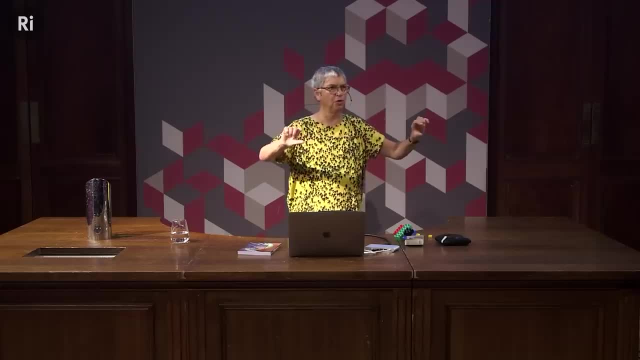 The leptons and the quarks and the bosons at the bottom. those are fundamental particles, So they don't contain other particles inside. It's not a composite object like this. It's like when I make when a particle decays. 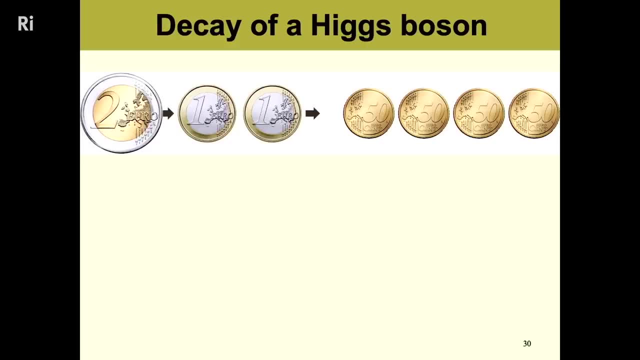 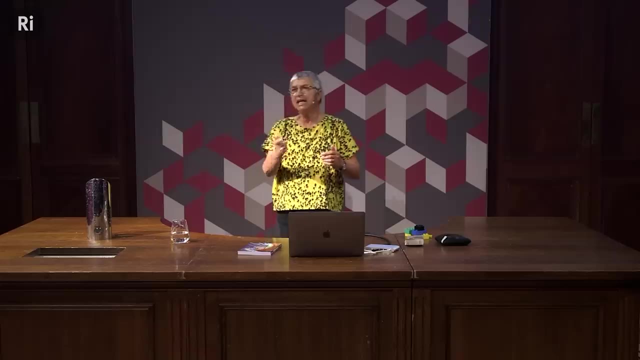 it's like when I make change for coins, If I put the two euro coins in a change machine and then I will receive two one euro coins or they can also break into four 50 cents. It's not that the four 50 cents were hidden inside the two euro coin. 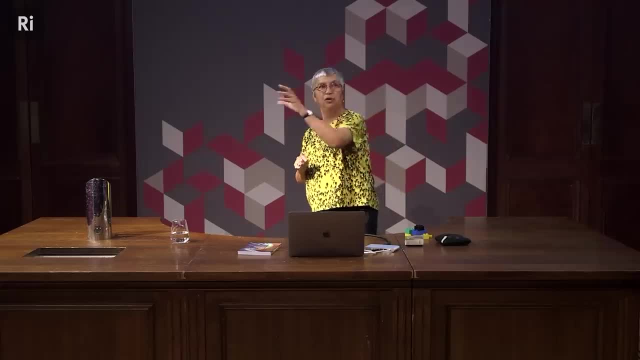 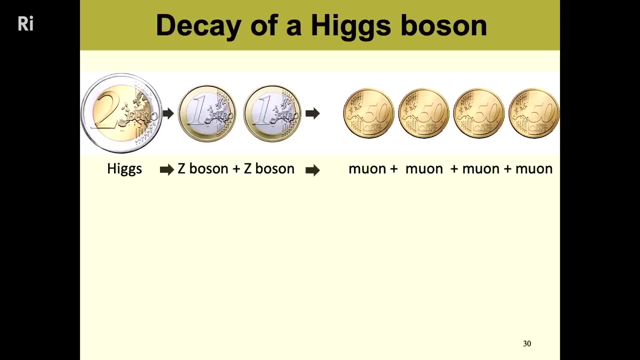 It's just that we exchanged the value of two, Two euro for two euros in the form of four, 50 cents, And so that's what happened with the Higgs boson. The Higgs boson will disappear, but it's equivalent in mass and energy will reappear in the form of two Z bosons. 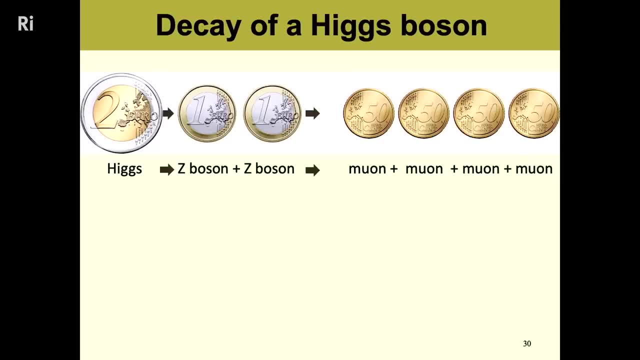 which bosons which are lighter. So the bosons will go fast, And then these two in turn will also break apart, And sometime they can produce four muons. So in the end we find four muons. But it could happen too that we had produced those four muons. 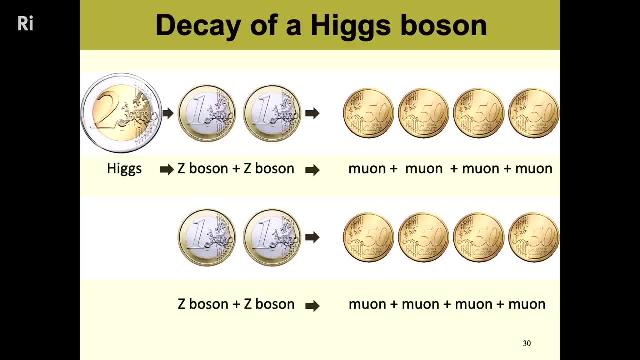 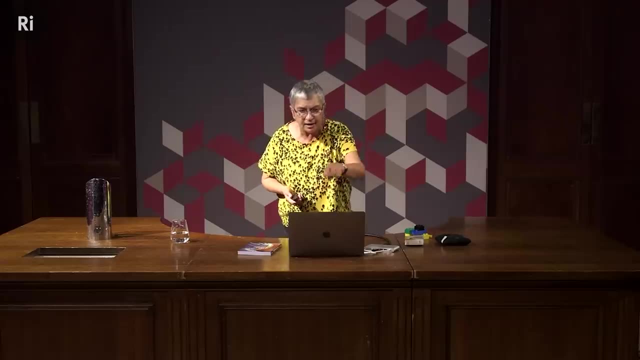 simply because we had produced two Z bosons, which is often, much more often than the Higgs boson. Producing a Higgs boson took a lot of energy, but two Z bosons was relatively easy. So when I find an event like this, 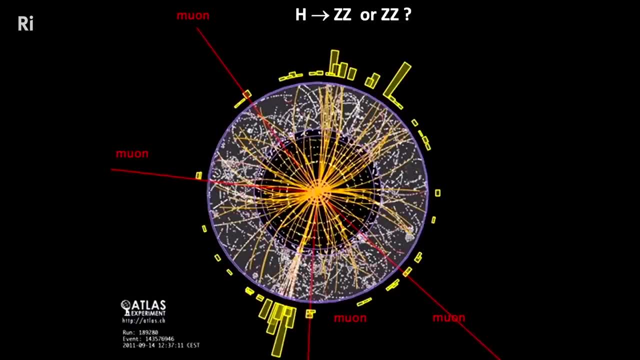 that I took with my detector, which is like a camera, and when I've done all the analysis I can tell: ah, I have four muons coming out real fast, The four lines that you see in red that went through our giant muon wheel. 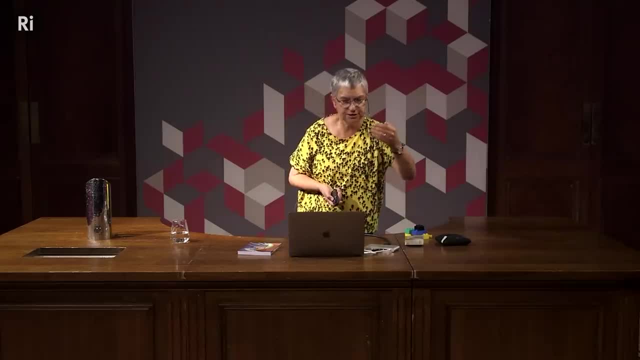 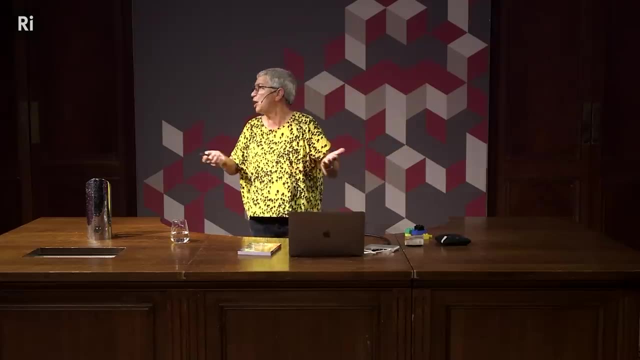 If I ask you is that, does that contain an event with a Higgs boson or two Z bosons that were created in the first place? Nobody knows. The only way to tell the difference is by looking at the Higgs boson. 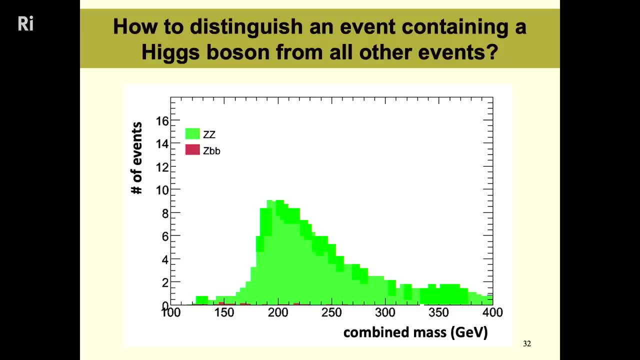 Okay, Okay statistics. If they were, only if the Higgs boson didn't exist and we were finding events with four muons we can count. on the vertical axis I'm putting the number of events that I am finding and on the horizontal axis it's the. 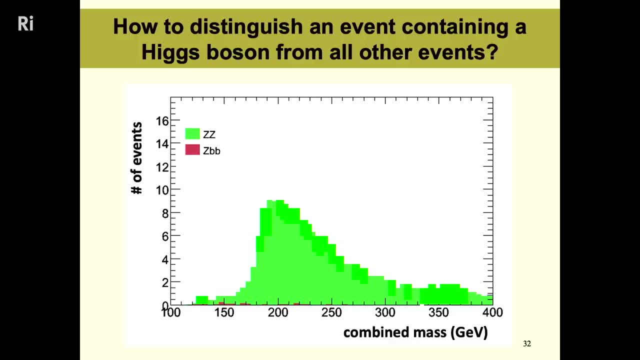 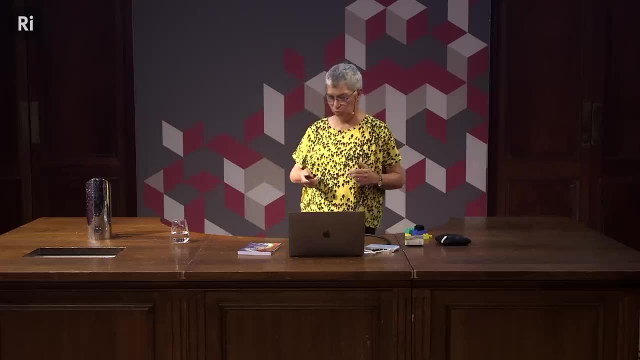 combined mass and energy of the four muons. And you can see, the theorist would tell us: oh, you should get a distribution that looks about like this: Okay, so this number, But if in addition to those two Z bosons, if in addition to that, 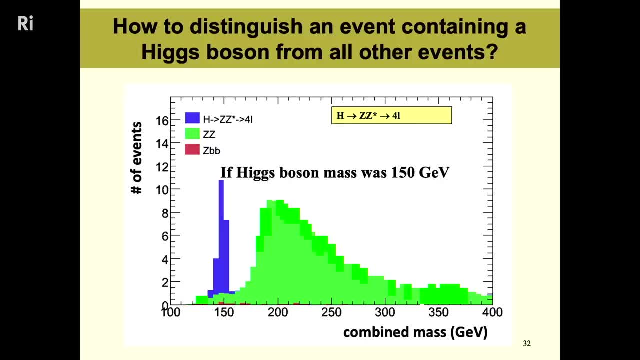 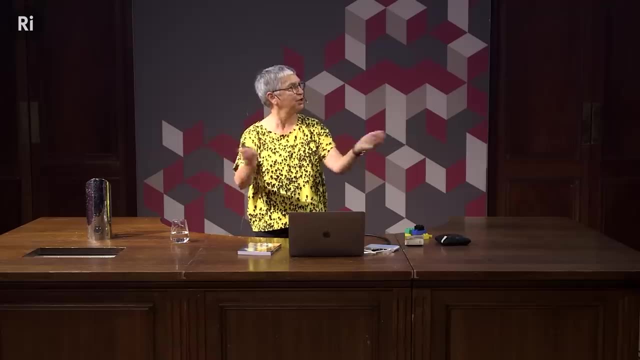 there is a Higgs boson, then we will see extra events appearing at the value that the Higgs boson mass has. We didn't know the mass of the Higgs boson to start with. Okay, fine, So we were shooting a lot of protons and exciting ourselves. 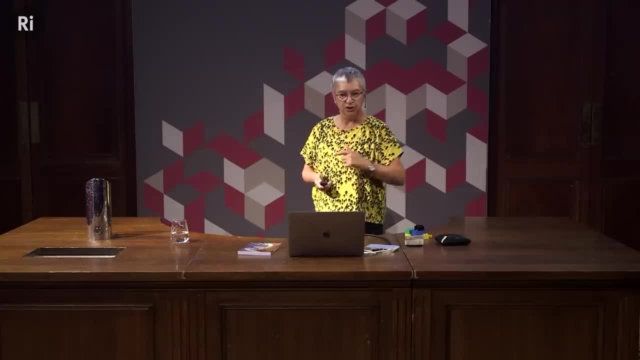 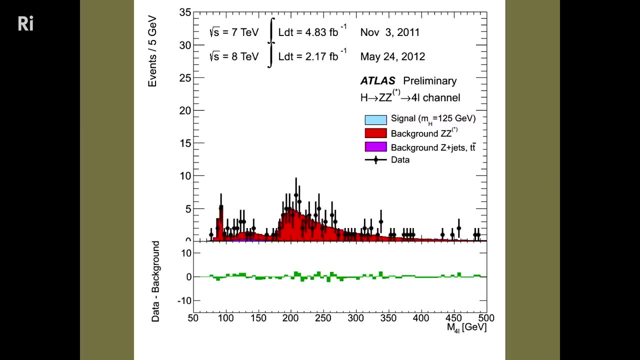 and the fabric of the universe. and then you know we started collecting events. So each black dot is an event that we collect in our detector And you see the number are growing with time. And at the beginning it pretty much reproduced just the red curve, but we see now that here in the 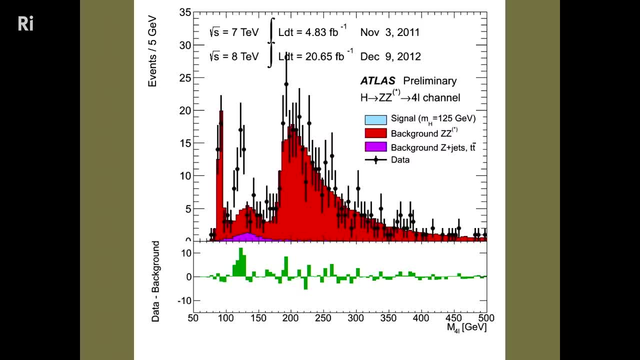 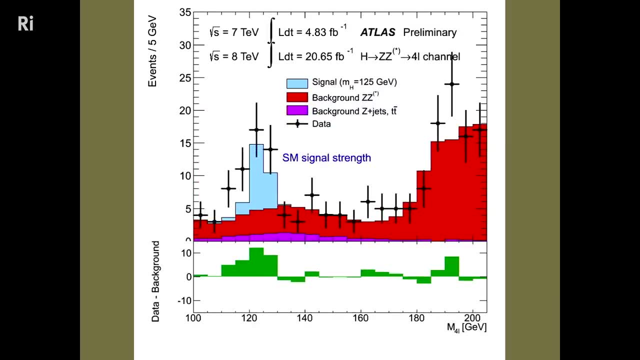 sorry, in this area, we start seeing an excess of events, And these corresponded to what theorists were saying, What theorists were predicting would happen if a Higgs boson had a mass of 125 GeV. So that's how we could tell, on the 4th of July 2012, that we had found the Higgs boson. 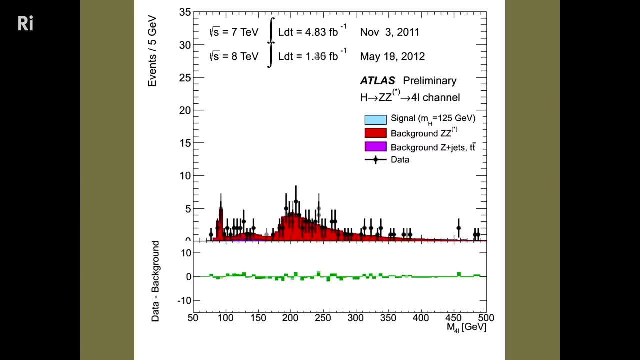 We started collecting data in 2011.. In 2012, we were at a higher energy of 80 GeV. so just to see it again, And so it takes time And you see a little excess that shows up here And that's how we could tell. 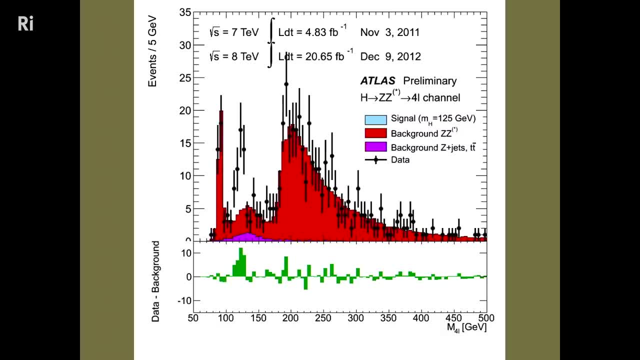 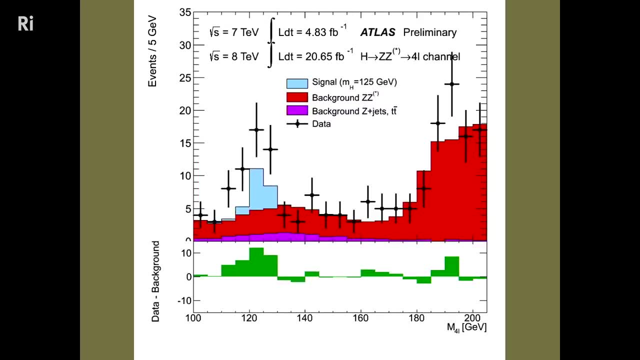 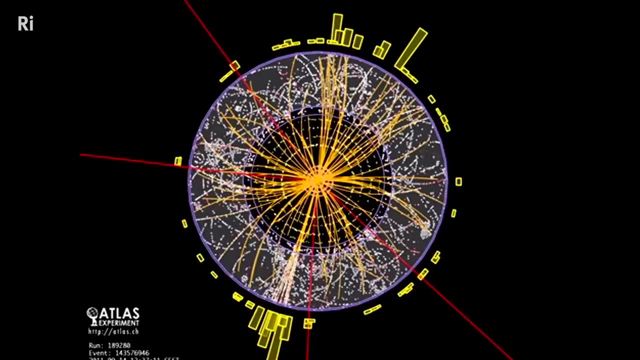 we had found one because there were more events than what was just predicted by random ZZ events. But still, when we look at an event like this, I cannot tell you. this is a Higgs boson decaying into 4 muons. I don't know, It's just the statistics that can tell the 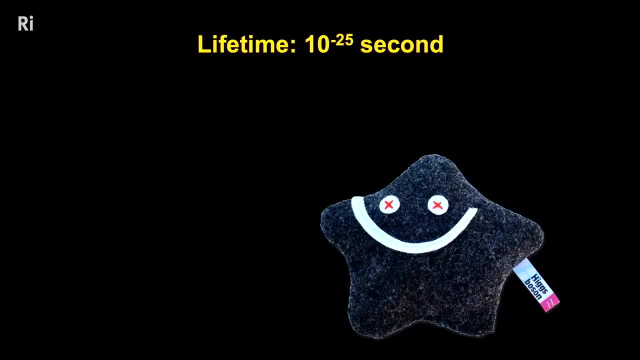 difference. So the lifetime of a Higgs boson is 10 to the minus 25 seconds. you have to get up pretty early to find something to do with that. So we will probably never find any practical application for the Higgs bosons. 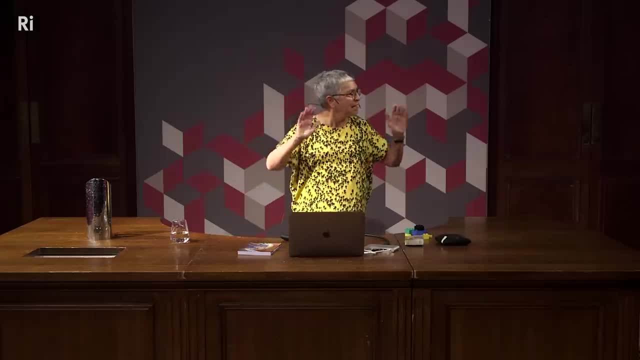 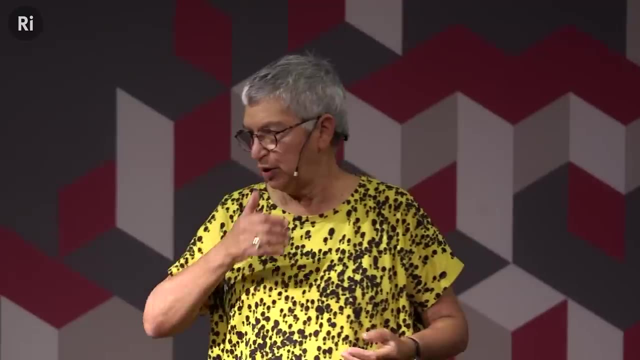 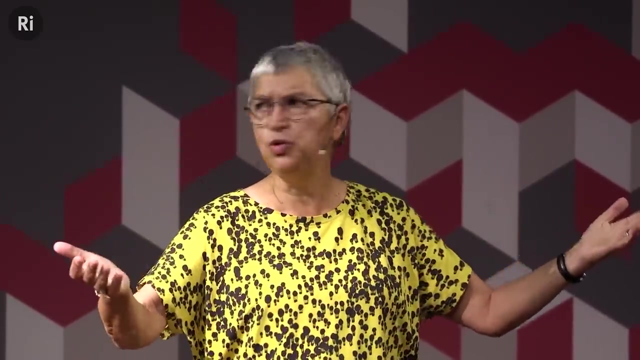 But around 1825, when Michael Faraday was working here on electromagnetic waves, the equivalent of the Minister of Finance came to visit him and he was asking him: what are you going to do with that? And Faraday said: no clue, but I'm sure you'll find a way to tax us on this. 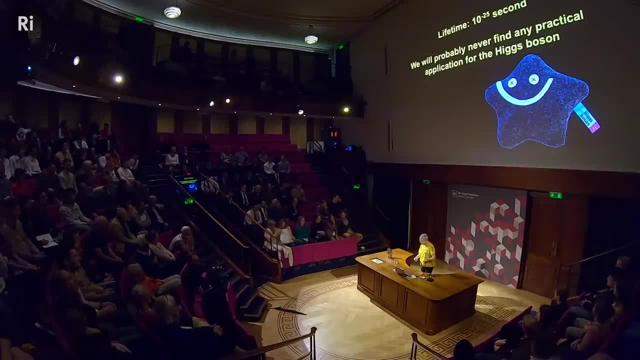 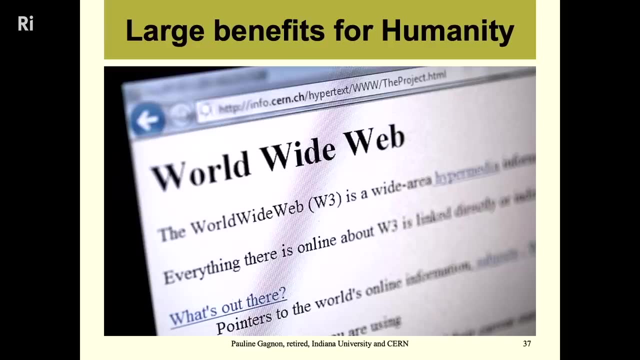 And Michael Faraday was done right and we pay for that now. So why do we bother to find those particles? We bother because when we do that, we develop new technologies. new techniques. For example, the largest benefit to humanity from CERN is not the Higgs boson. 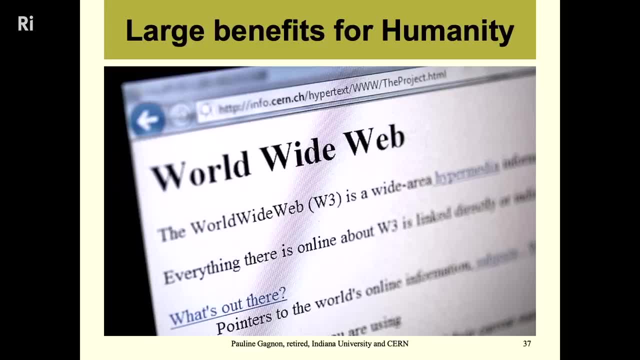 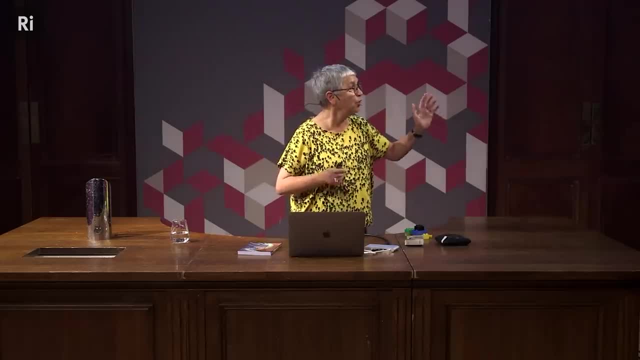 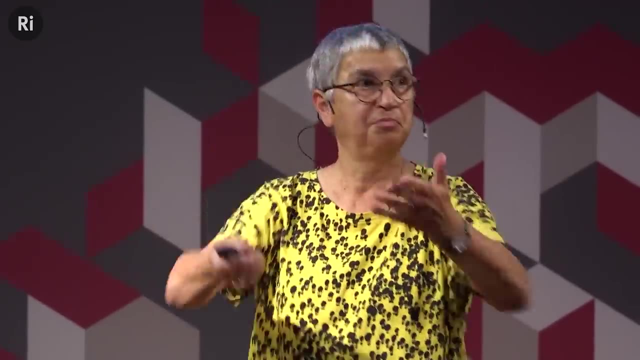 The Higgs boson is as useless as can be, But it's the World Wide Web. We were 13,000 physicists from 118 countries working at CERN, So of course we needed ways to communicate with each other, And that's how this need brought into play. 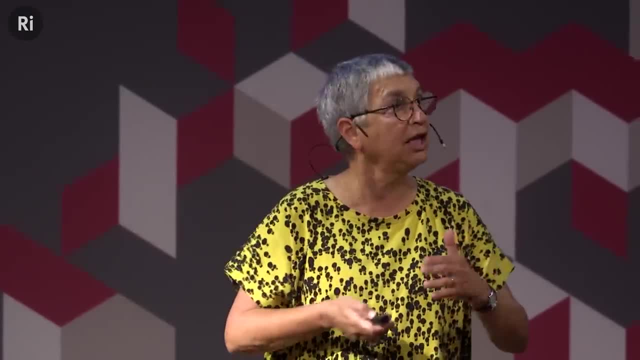 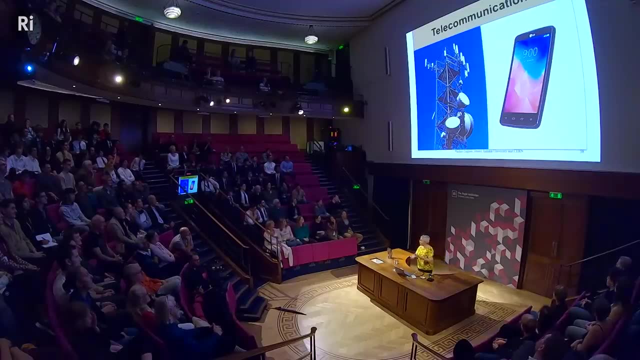 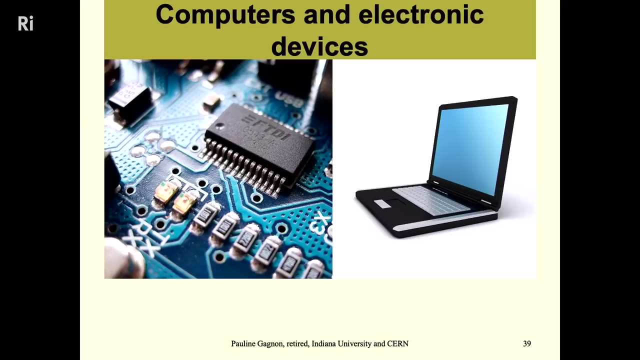 that we put efforts to communicate with each other, and that was the World Wide Web. And for telecommunications that's the same thing: All the work that Michael Faraday did on electromagnetic waves. now we put that to use, The work that physicists did on electrons. 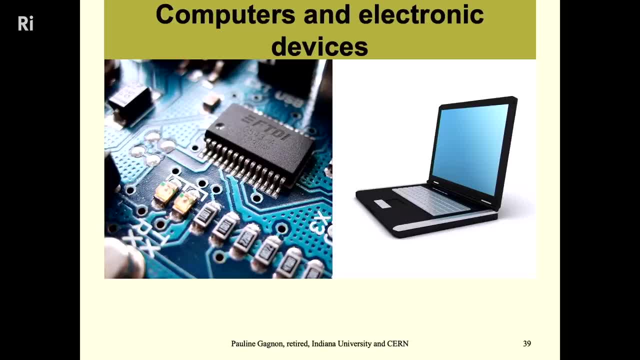 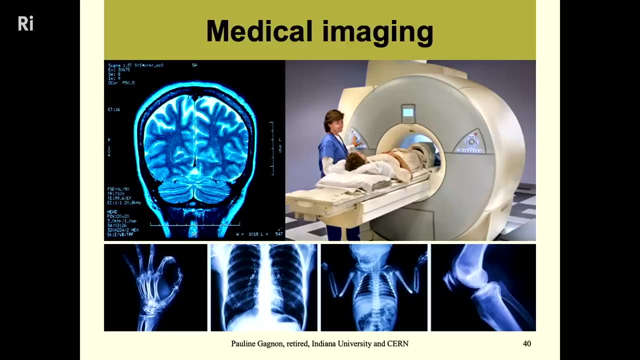 now we have all these electronic devices that end up in the garbage And so yeah. so computers and electronic devices. thanks to the creativity of countless engineers and technicians, we have that put into use. Medical imaging is probably the most direct byproduct of the research that we do at CERN. 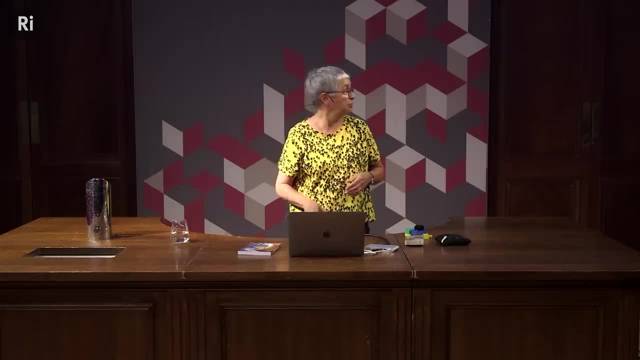 because that's the kind of techniques that we do at CERN, because that's the kind of techniques, because that's the kind of techniques we use to detect particles, And so X-rays and computer tomography with MRI- magnetic resonance imaging. 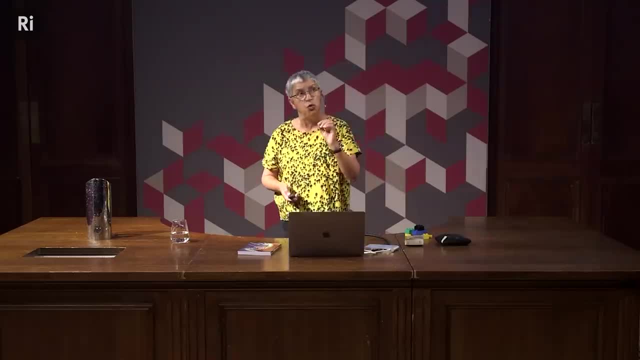 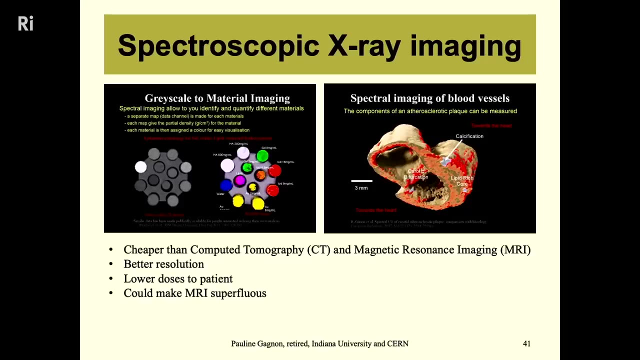 all those techniques come from particle physics. There is a new one that just got invented, and it was published at CERN a month ago, and it's called spectroscopic X-ray imaging. So instead of operating X-rays at just one frequency, now they use X-rays. 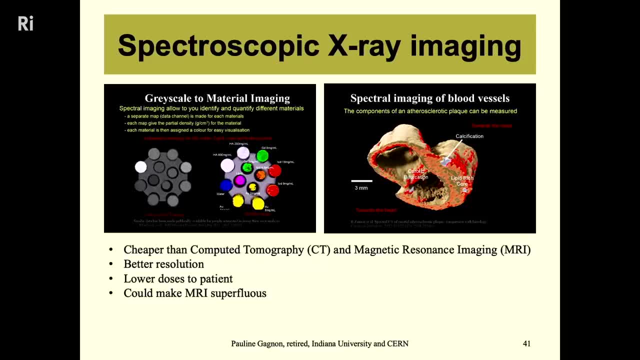 So instead of operating X-rays at just one frequency, now they use X-rays at just one frequency. now they use X-rays at just one frequency. they use many frequencies, so a large spectrum of X-ray values and they can do things in color. 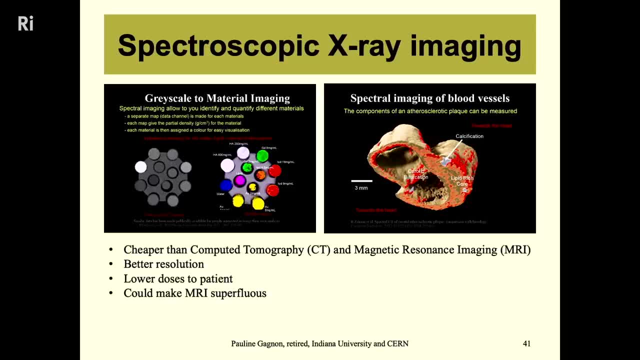 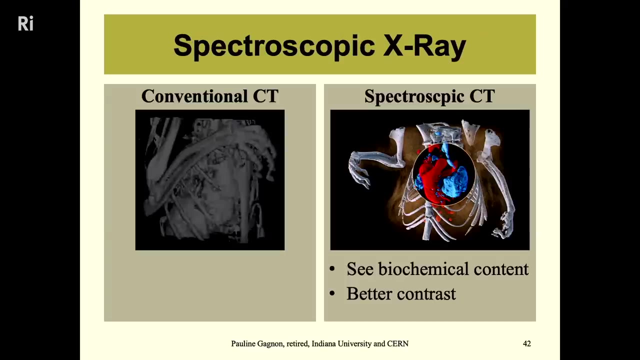 as if before it was just black and white. So they can now. it's cheaper than computed tomography and magnetic resonance imaging. It gives better resolution, lower doses of radiation to patients and it could make CT and MRI superfluous. These are two pictures with conventional X-ray. 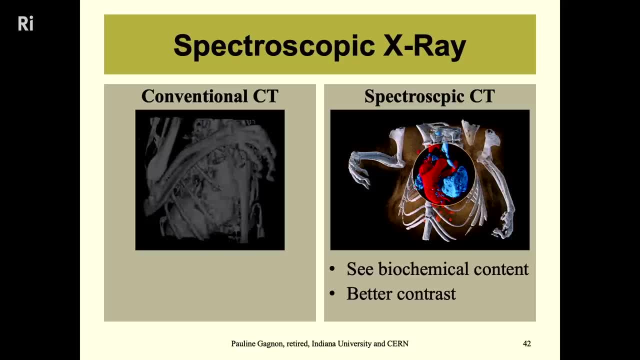 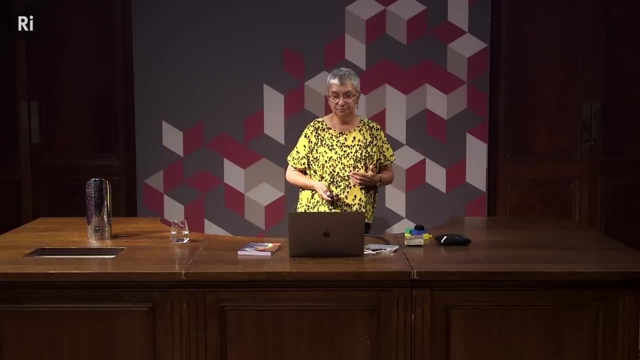 or computer tomography done on a small mouse and to the right with spectroscopic CT And you see, you can see the biochemical content and a better contrast. So the images are much better than we have before. So we'll have better medical diagnostic with that. 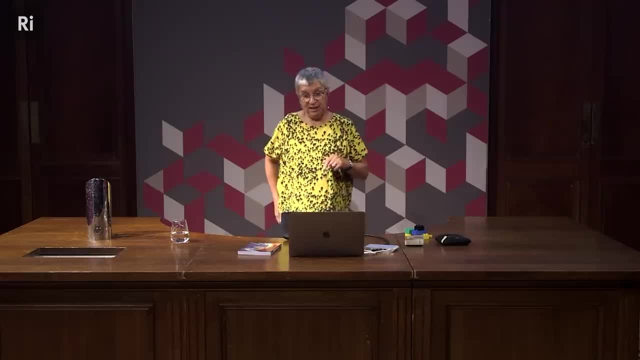 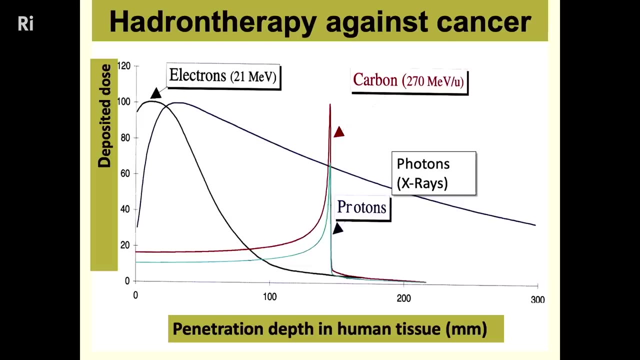 Another technique that was developed here at the Royal Institution by Bragg was this. you know this technique. we call this particles like made of hadrons, like protons, neutrons, no, mostly protons, carbon, with an electric charge as well. 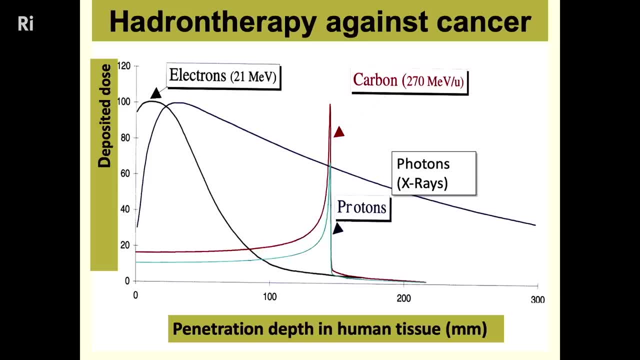 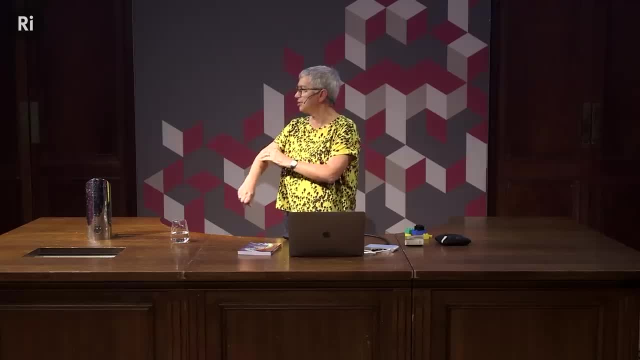 will deposit most of their, all their energy, or most of their energy at a specific depth. So if you have a tumorous cancer, something in your liver which is, I don't know, three, four inches inside your body that this tumour is, 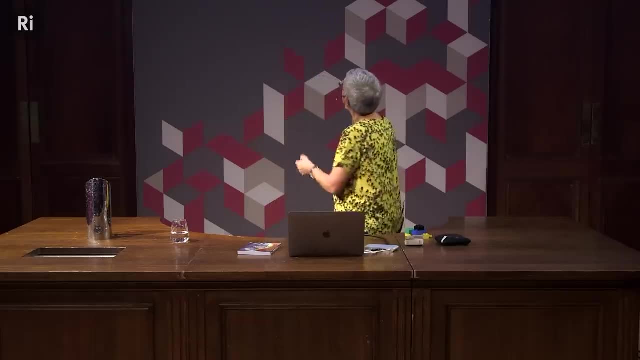 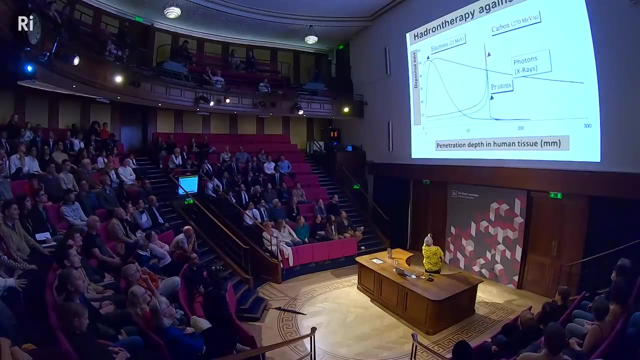 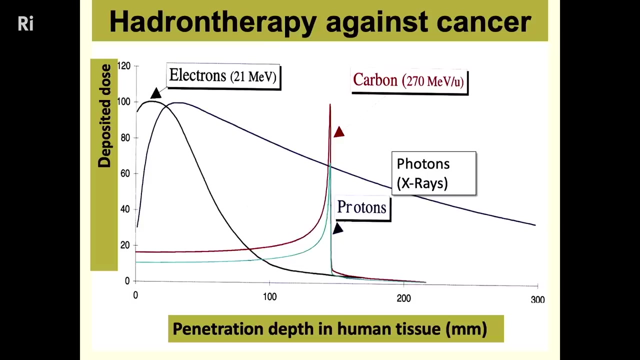 if you were to use X-rays. if we look at that here- X-rays are here, the black curve- you see that the X-rays will deposit energy all along the way, say that our tumour is here and so it will damage healthy tissues. 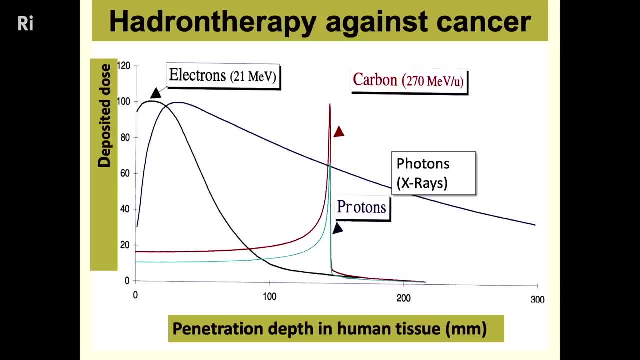 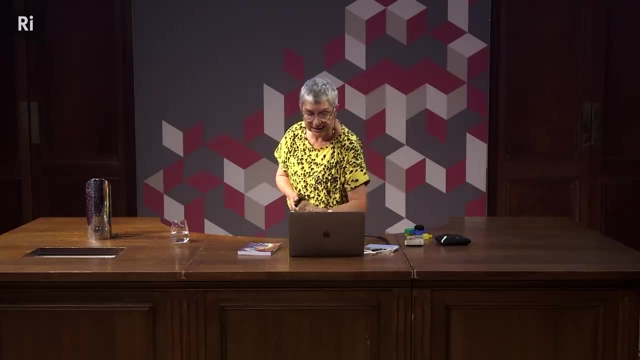 at the same time as zapping the tumorous cancer cells. But with protons they will deposit all their energy exactly at the same time And that's where we tell them to go. We can just tune where we want that. So it's a very powerful technique to fight cancer. 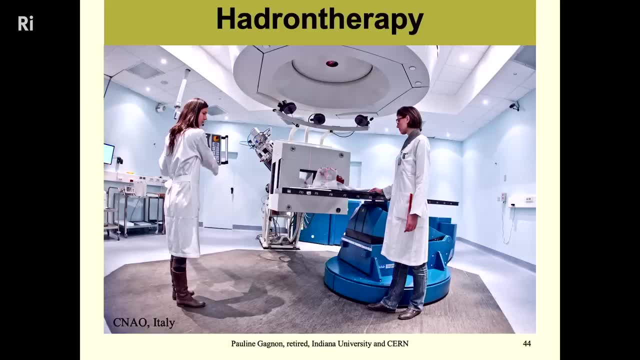 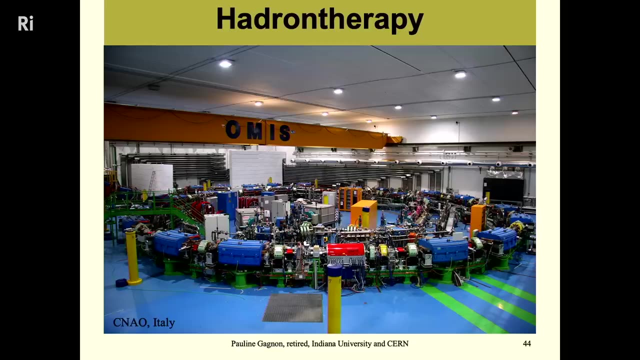 and it's called hadron therapy, And this is a centre that CERN contributed to building in Italy. That's what patients see when they go in for treatment And this is what is behind the door, the wall that nobody sees, And you can see the touch of CERN there. 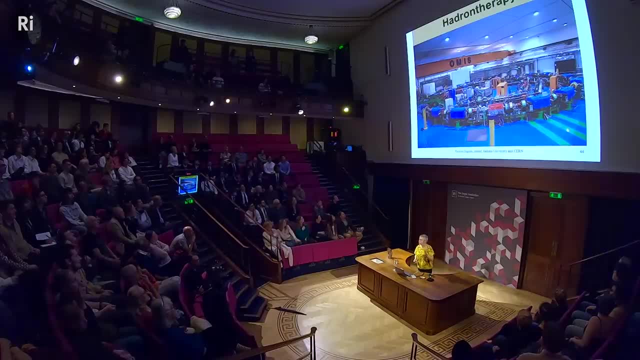 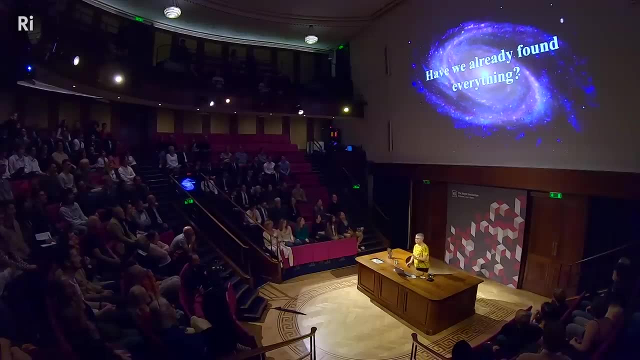 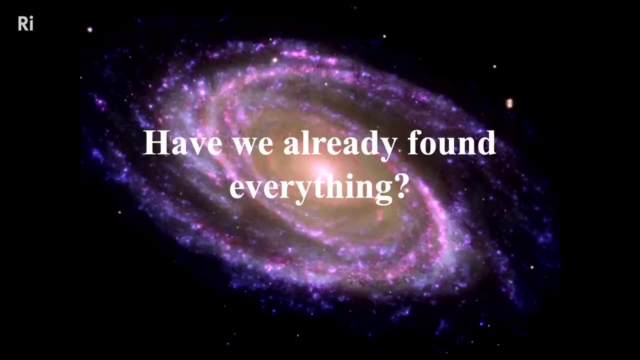 this particle accelerator. Just about all the best things we have today come from fundamental research. Okay, and I'm going to close this discussion. in the next 10 minutes or so on, have we already found everything. So especially for the young people here. 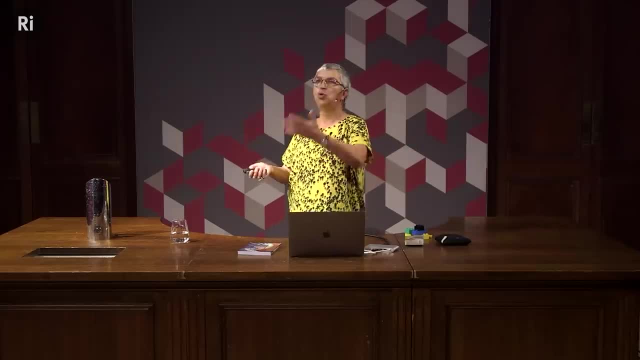 that's a big question because you know, if we've already done all the job, why would you bother to study in science? Well, please hang on In the content of the universe. we now have a good idea of what is inside the universe. 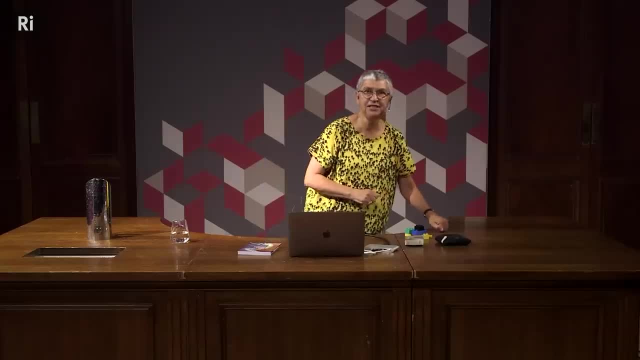 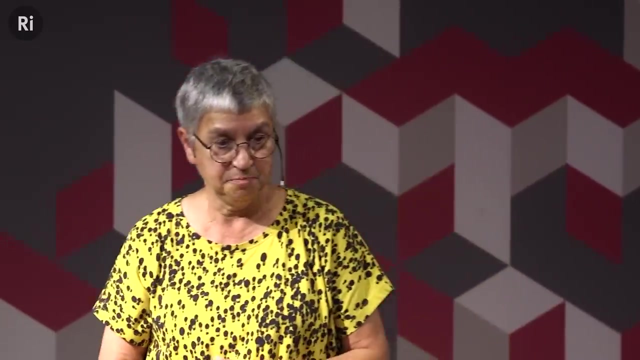 Everything that we know as matter, visible matter- made of quarks and emitting light when it's heated up, like stars and galaxies, we can see them. all that is made. we call it visible matter because it emits light when it's heated up. 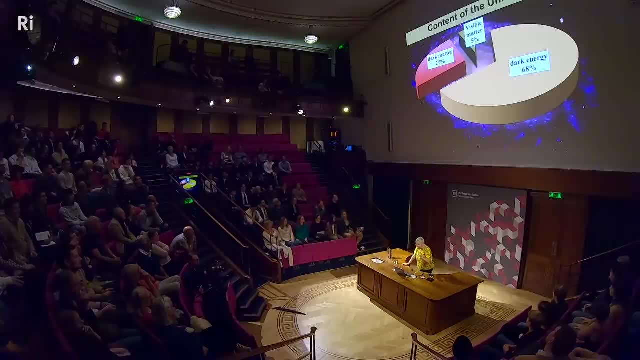 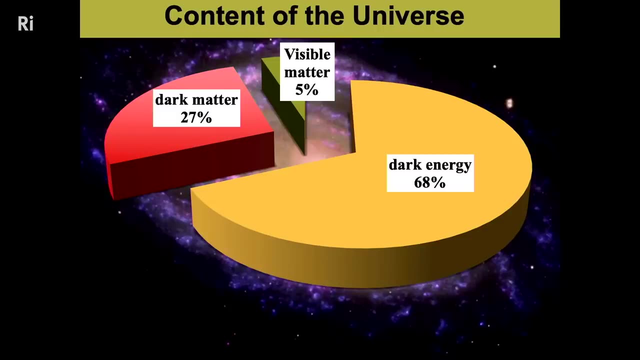 and we see it. So this visible matter only accounts for 5% of the content of the universe. So 100, 200 years of work by particle physicists and we have only understood 5% of what is there in the universe. 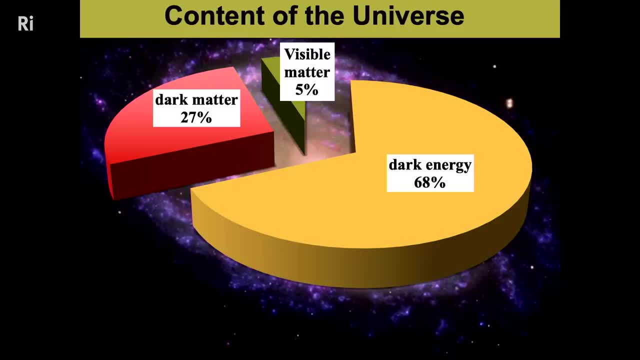 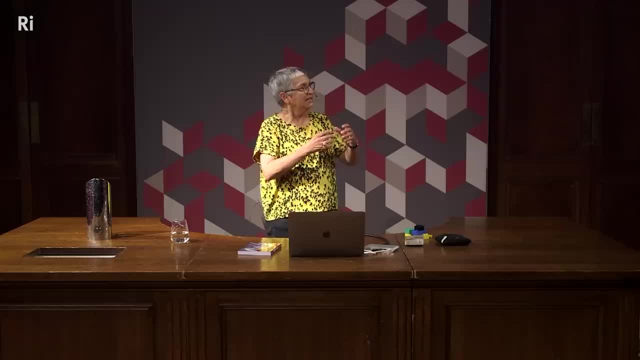 We now know that there is dark matter, a type of matter which is 5 times more prevalent than regular matter, visible matter. It's matter that reacts to gravitational waves. It's very, very common waves. It has mass, So we can see it with gravitational lenses. We can feel the effects. 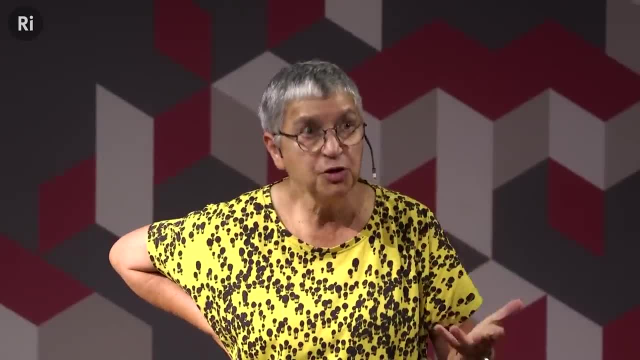 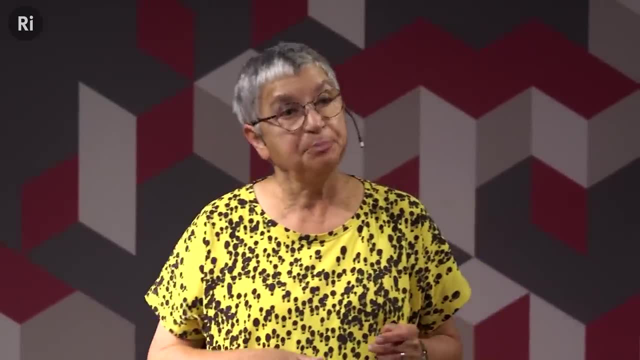 the presence of this mass, this matter, but we don't see it. It doesn't emit light, So we call it dark matter, And not only that, and that's 27% of the content of the universe. We have no clue. 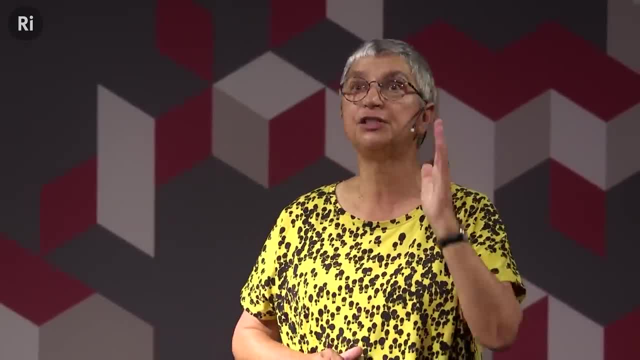 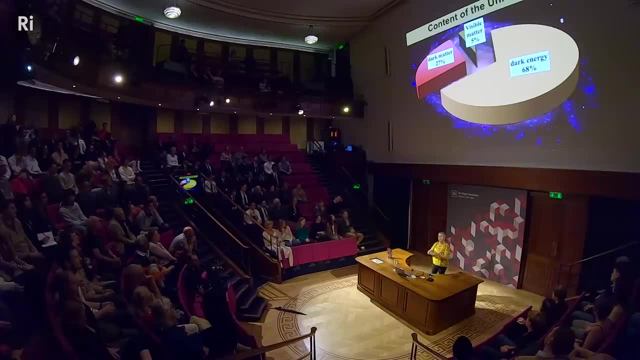 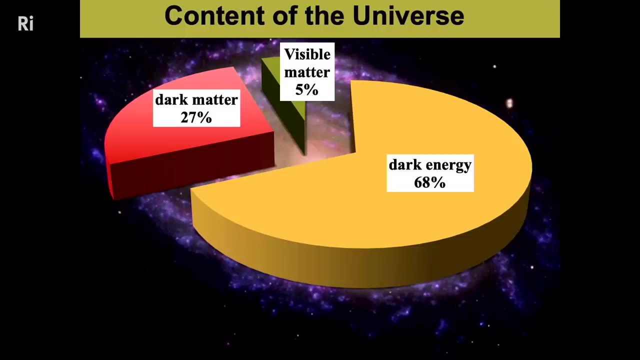 what it is, No clue, We just know it's there And we have lots of ways to know that it's there. I can talk about that later if some people are interested. And finally, 68%. it's embarrassing: 68% of the content of the universe is in the form of energy that we know nothing about, And it's 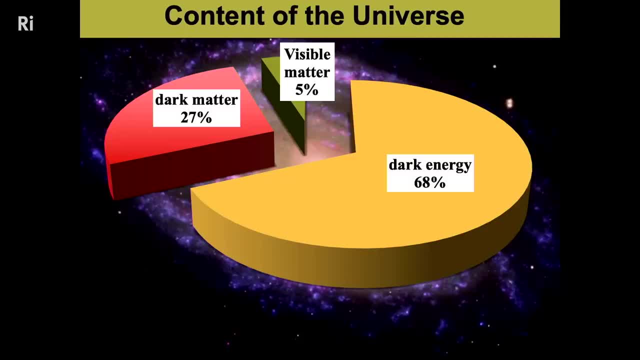 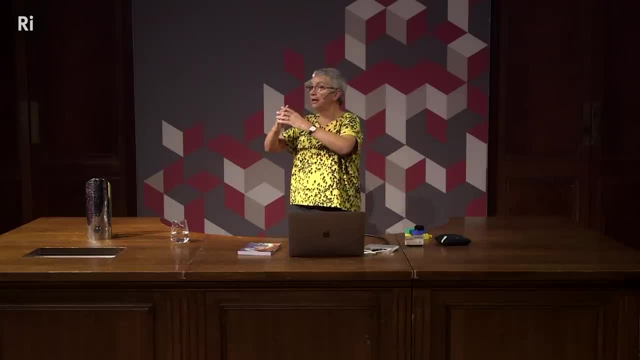 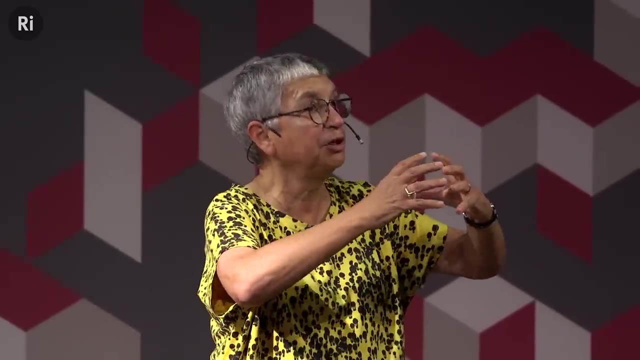 called dark energy. But we know it's there because about 20 years ago some astrophysicists realized that you know that since the Big Bang the universe is in expansion, But in fact they realized that not only is that in expansion, but this expansion grows. 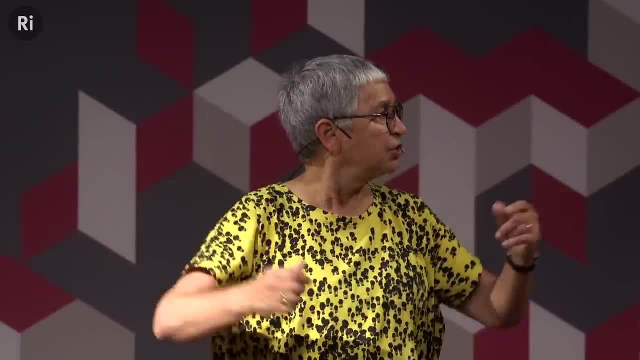 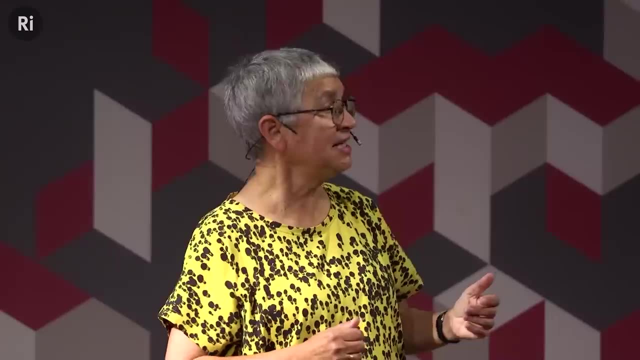 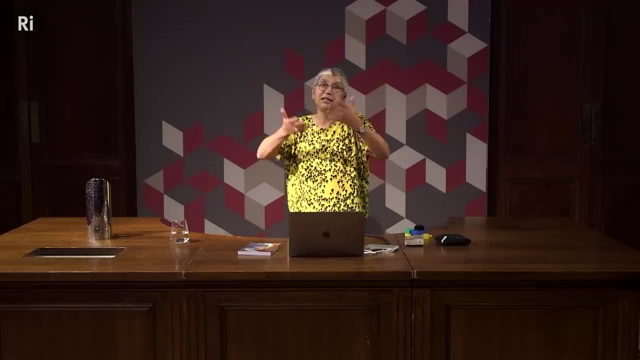 is always accelerating, So the expansion of the universe is going accelerating. You know that if you want to accelerate in your car or on your bicycle, you need to give energy. Where does this energy come from? No clue, But you can imagine that we need a lot of energy to accelerate. 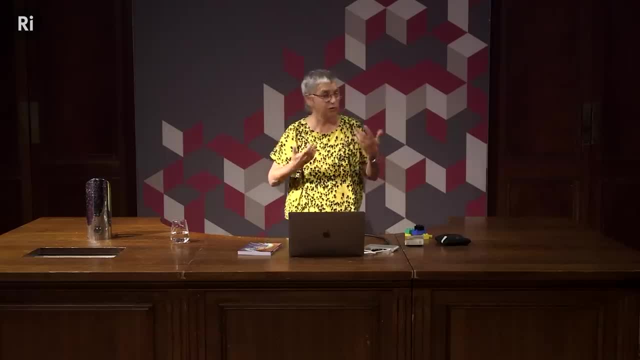 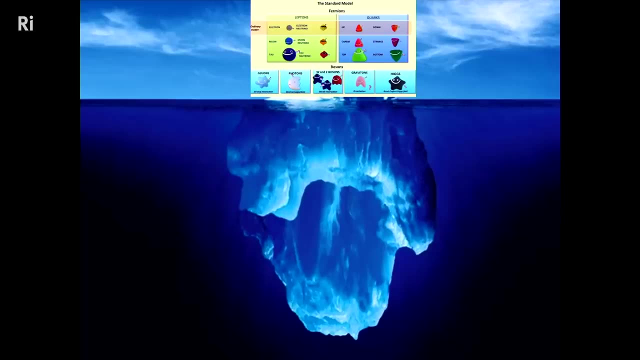 in the expansion of the universe, And that's why the dark energy accounts for so much. So all the particles that I described before are only describing the tip of the visible part of the iceberg, And the rest is completely unknown. So we know 5% of the content of the universe, And you 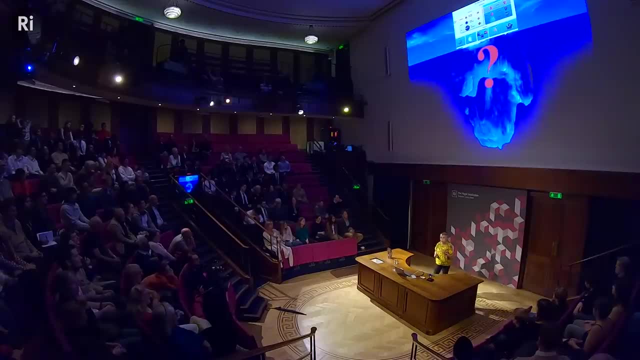 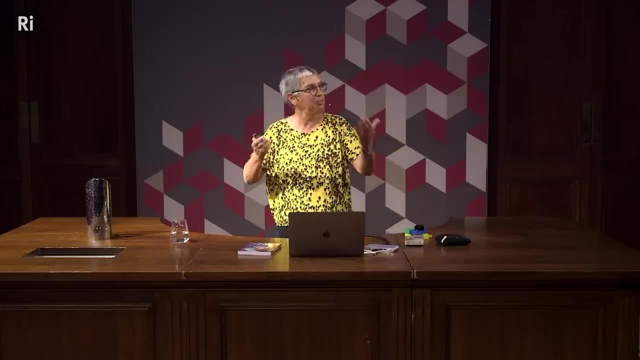 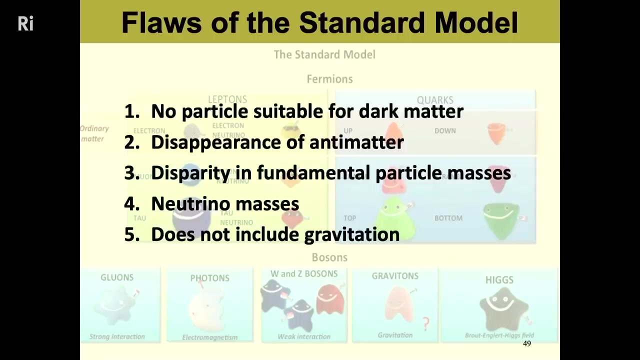 all the young people who came tonight. it will be your job to find what is this 95% that is missing. There are some good job opportunities ahead. There are several flaws in the standard model. There are no particles that we know of that is suitable for the dark matter. It doesn't predict anything. 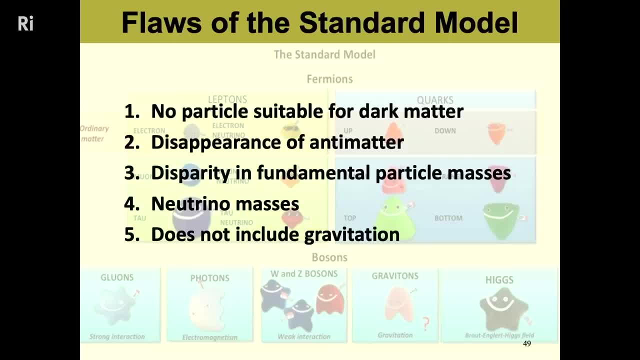 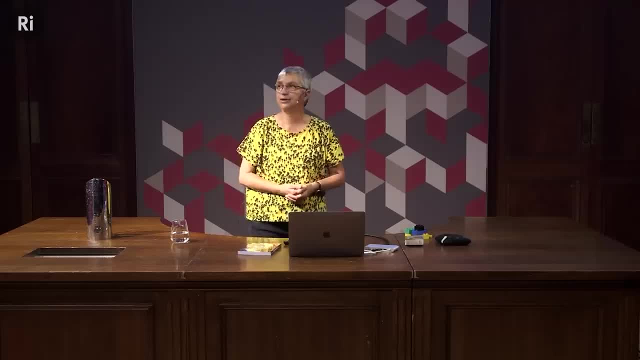 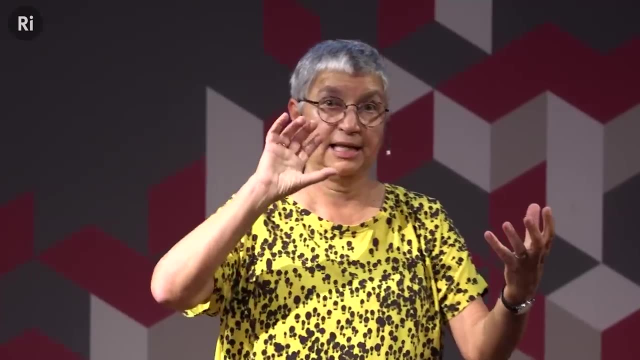 that we could use This appearance of antimatter. every time we produce matter in the laboratories, we always produce as much antimatter at the same time, But, and so we know that right at the Big Bang, just as much matter as antimatter was produced, but it has completely disappeared from here. 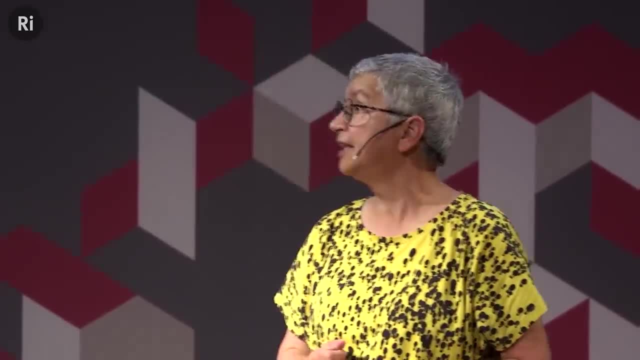 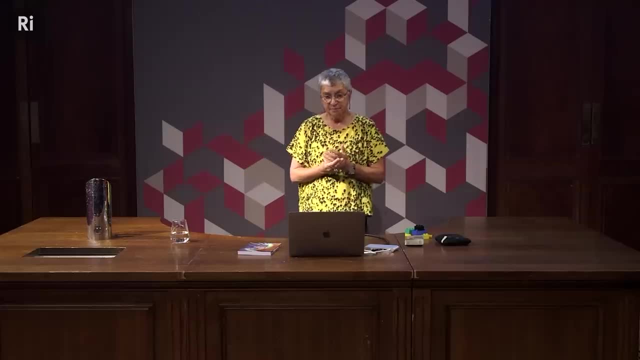 Many of you are saying, yes, they knew that. Maybe you have seen the talk that Tara Shears gave here a few years ago. It's available on the website from the RI, And so it's a big mystery. We don't know what happened. 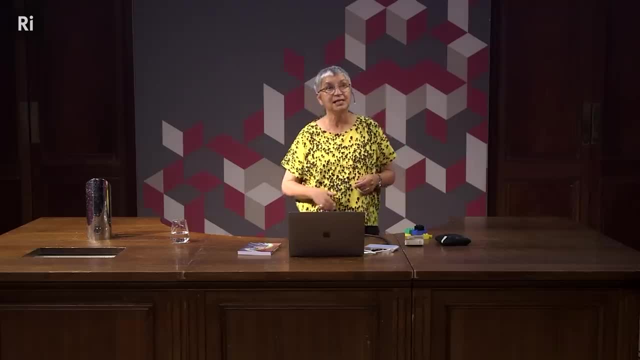 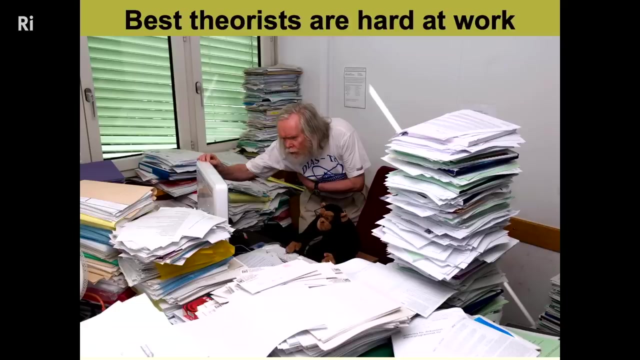 There is disparity in the masses of the fundamental particles. What I was telling you before- three generations of particles with completely different masses- makes no sense. The worst construction set you find on the market, And it does not include gravitation. So the best theorists are hard at work, Like here John Ellis, very famous physicist from CERN. 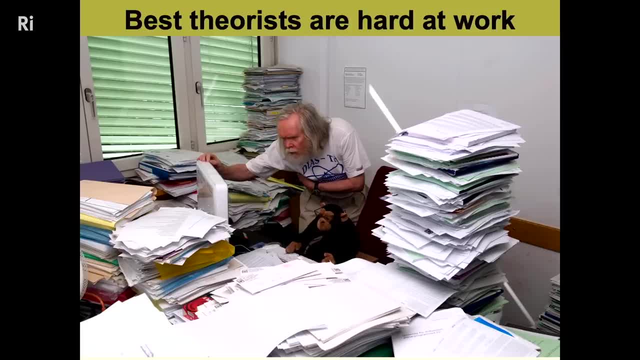 a theorist who works also here at King's College, and his assistant, Mademoiselle Mumu, And they're just now trying to to figure out what, what could it be What? what theory would be better or could be? 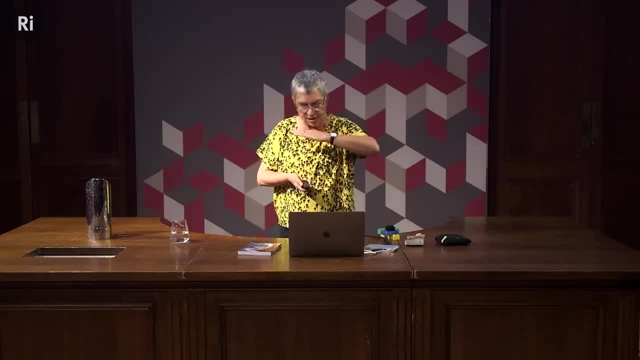 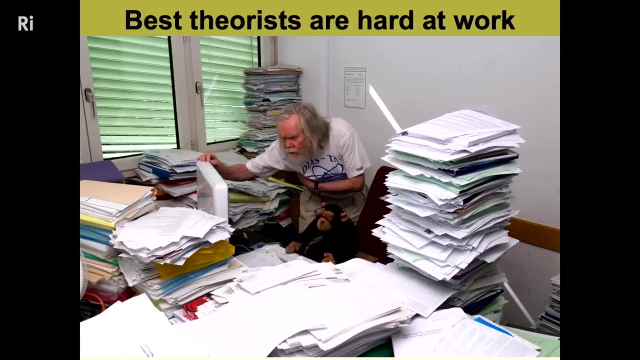 what could we build on top of the standard model to go a bit further and answer those unanswered questions? And so he has these piles of papers in his office. So when I was there taking the picture, I said: but John, have you read those papers? He said I read your paper. 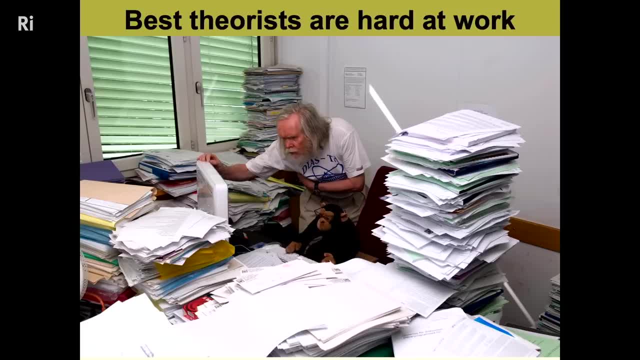 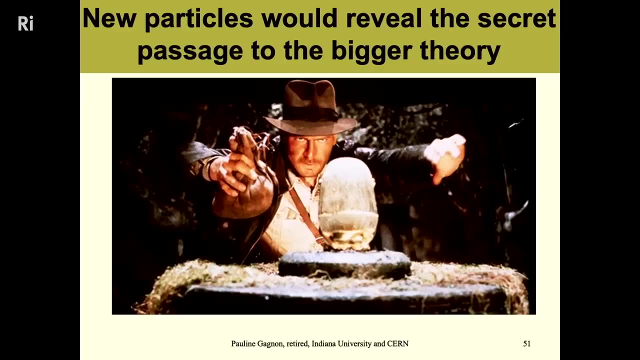 I said yes, okay. And then I said, do you know where it is? He said: don't push your luck, Anyway. so theorists are really stuck. They come up with all sorts of theories, but we don't know if any of those theories are good. 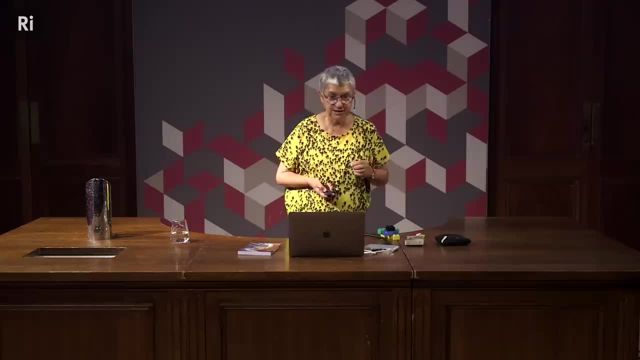 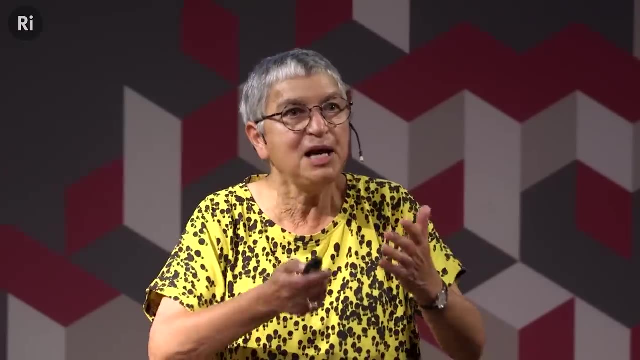 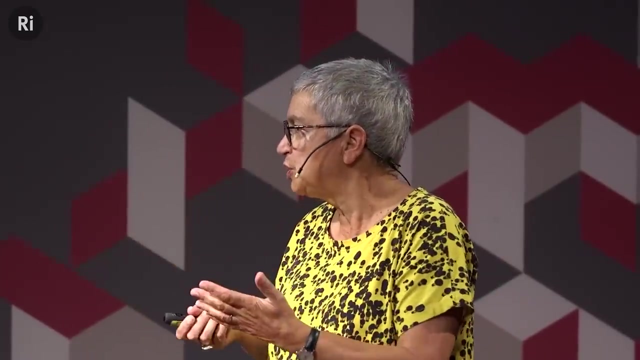 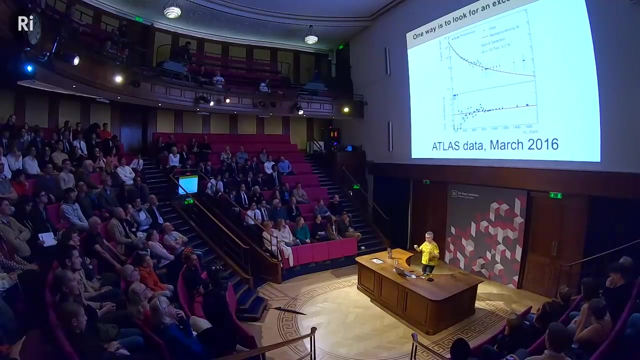 It's only when we will find new particles that we will be able to tell which one of those theories was valid. Now we have no clue. The theories are producing tons of new ideas, But no one knows which one is true. Every time we have a small anomaly, everybody gets excited. 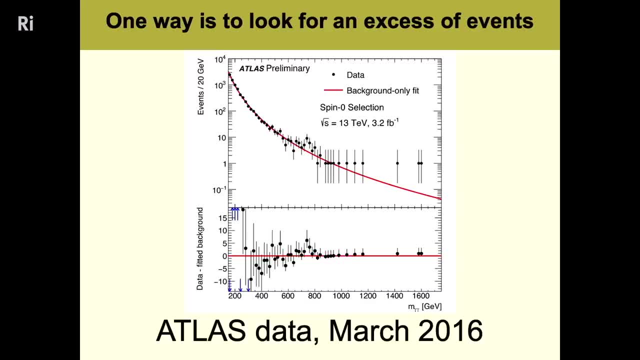 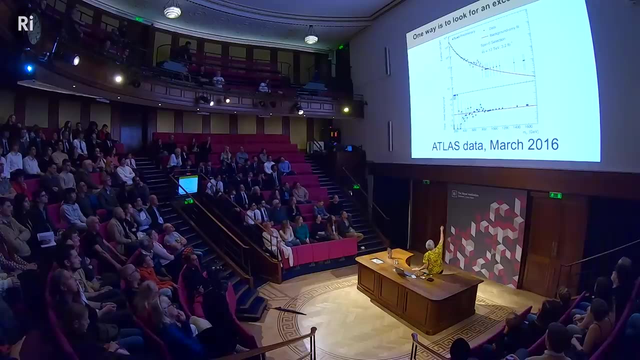 For example, a few years ago, in the 2000,. at December 2016,, just before the end of the year, ATLAS showed some preliminary results and we were seeing already a little excess of events. No, a bit like what I was showing for how we found the Higgs boson. 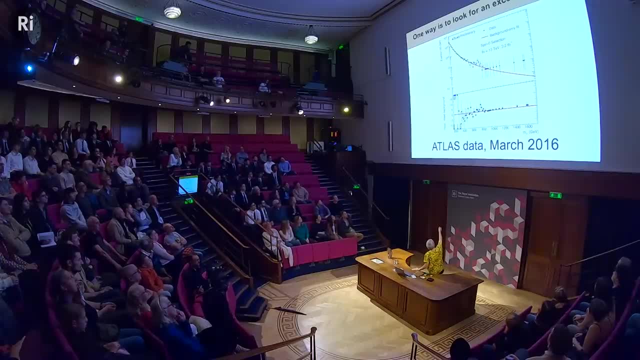 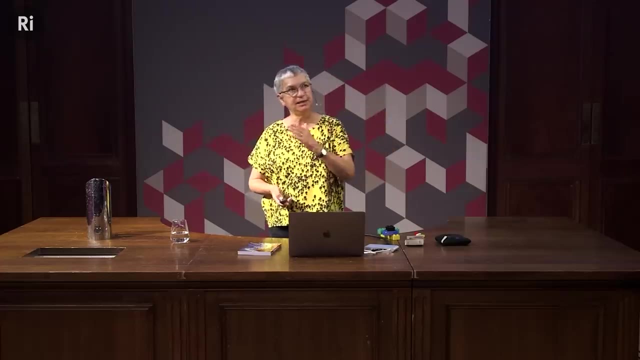 You see, here there was a little more events In the 90s there was a little more events. This is the number of events we found and the distribution in energy when we were looking at two photons coming out of the detector, And so nobody would have been too excited, especially at the end of the year when everybody wants to go on vacation. 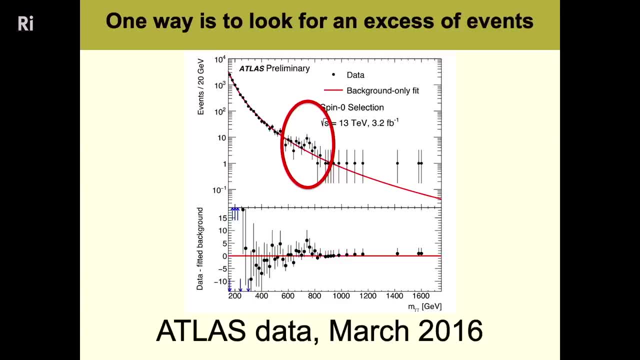 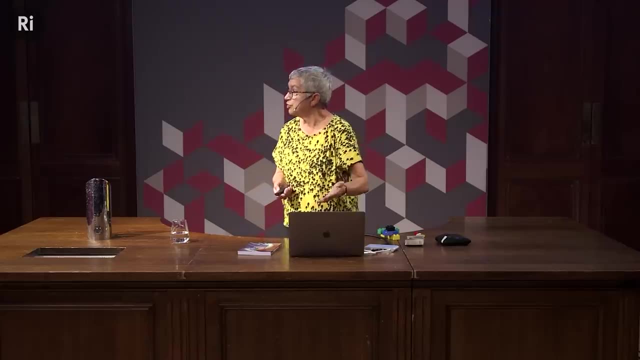 But then CMS also found the same thing. Then it was the end of the year and we always stopped the accelerator for three or four months for the maintenance. So we had to wait a few months Before we accumulated enough data to check if this was real or not. 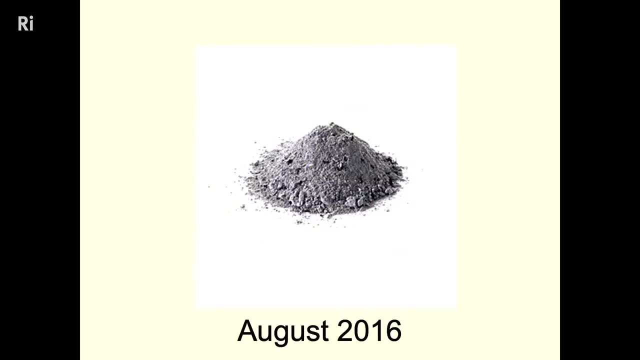 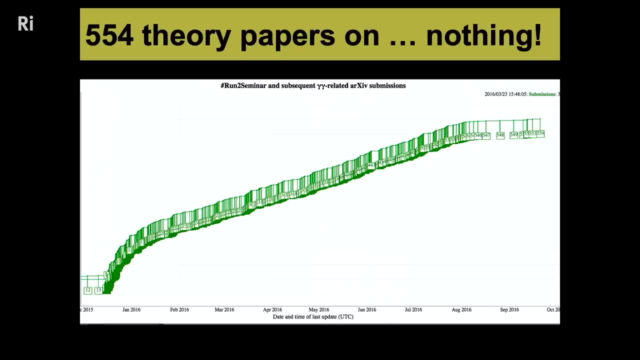 But unfortunately it all disappeared. It turned out to be a pile of ash, So there was nothing there. But in the meantime the theorists got so excited. 554 papers were written to explain what could produce such things. 554 papers were written to explain what could produce such things. 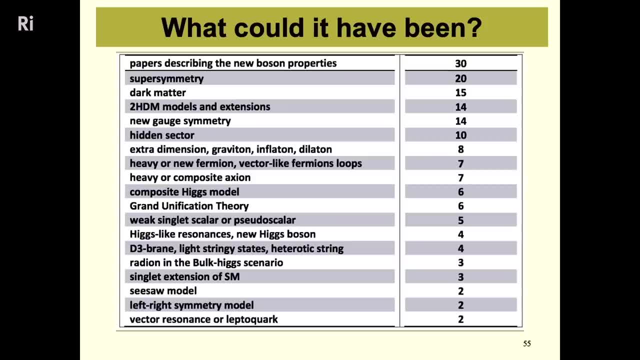 554 papers were written to explain what could produce such things, But they came up with the weirdest things Like composite Higgs, motile, grand unification theory, D3, brain light, stringy states, There are Wim Zillers, there are Hubertron. there are all sorts of weird things that are being proposed. 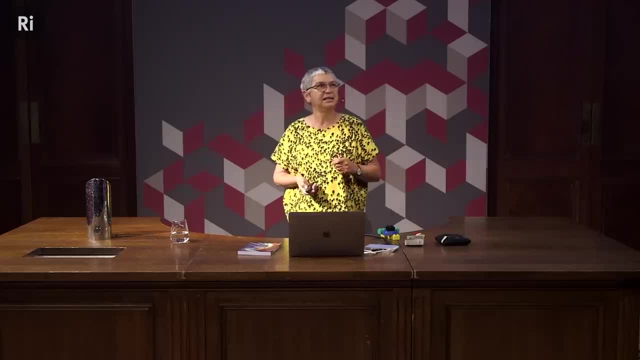 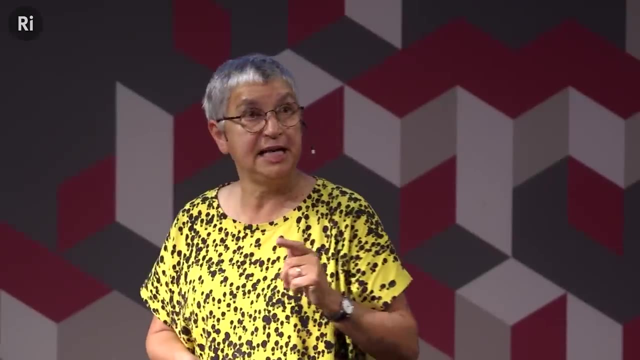 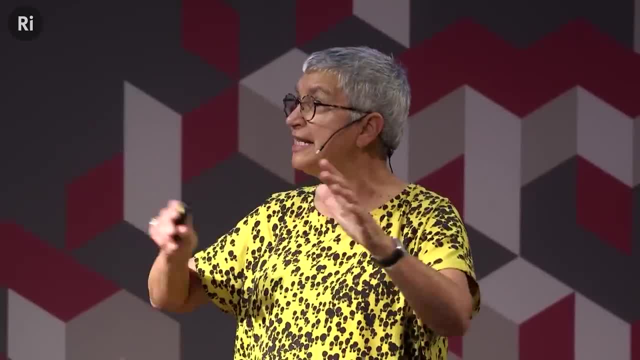 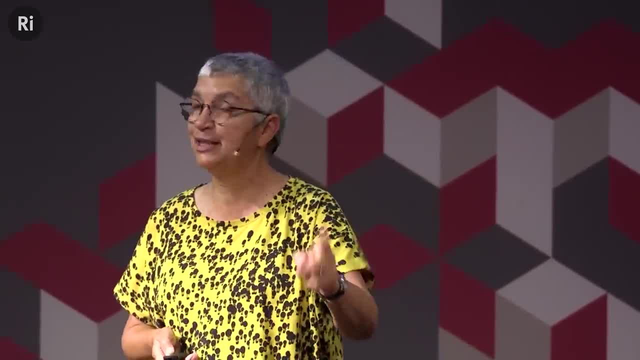 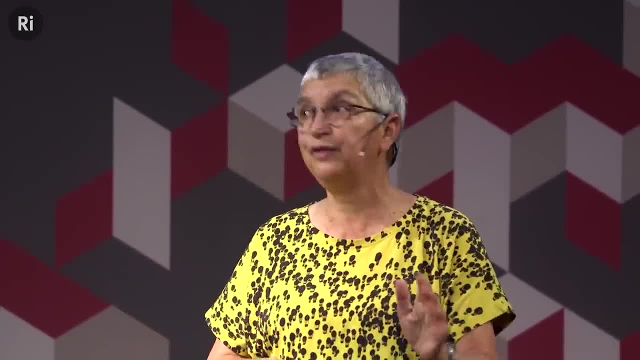 But until we find an experimental evidence, we don't know what is there. But until we find an experimental evidence, we don't know what is there. I'm sure that at least a few hundred were really good. Right now we have a few, a handful of events again. 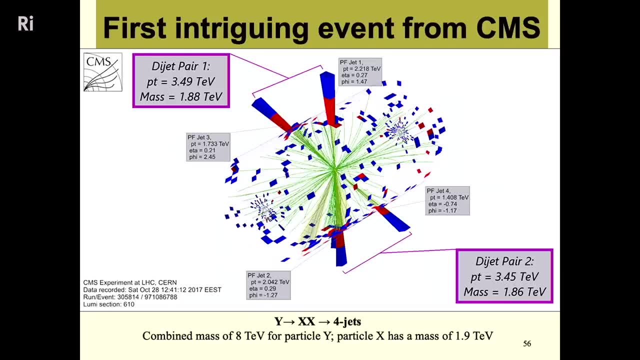 that are intriguing. For example, the CMS experiment found events where there are jets, of particle jets. When you have quarks coming out, quarks never come alone, They always produce more quarks and we end up with a jet, a bunch of hadrons coming out, all finely collimated together. 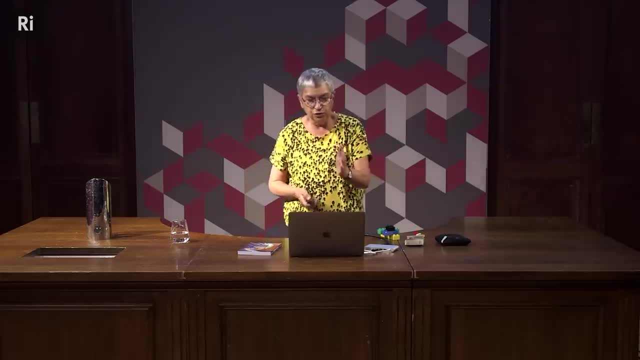 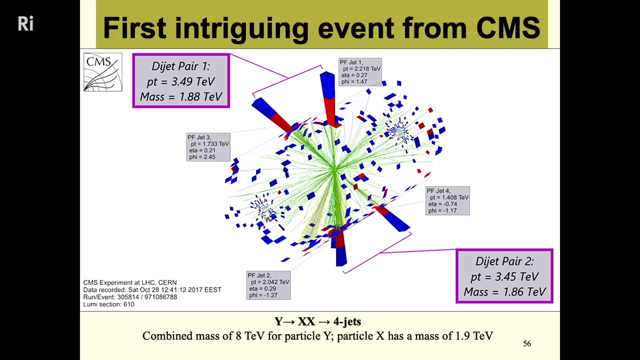 and we call that a jet. So they found some events with two jets coming in one direction and two other jets, and each pair of two jets weighs about 1.9 TeV. We measure everything: the mass of a particle, measured always in energy. 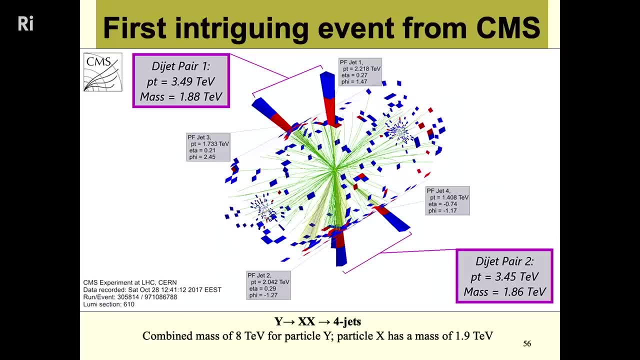 because mass and energy are equivalent, so those are tera-electron volts, It's just a unit of energy, And so both die jets have about the same mass, and the other one would be 8 TeV, so it's huge. 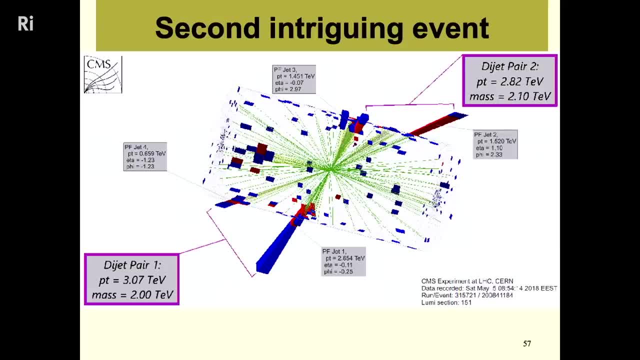 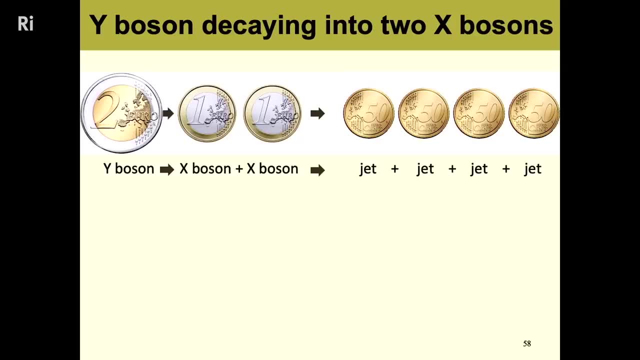 And they have two events like that that they have found, and it would be possible that a new type of boson, a Y boson, would decay into two X bosons and each of them would decay in turn in two jets. So that would be something new. 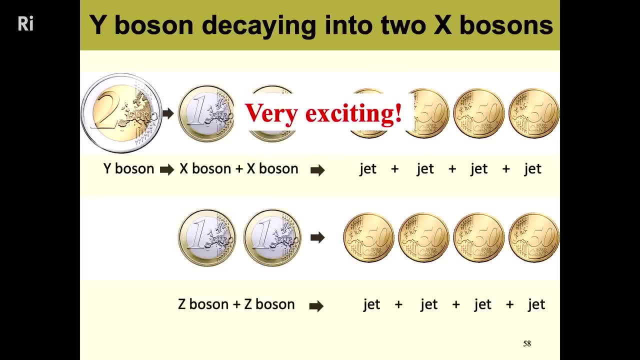 It would be very new and extremely exciting, But it could also happen that it comes from two Z bosons producing two jets each, and we've seen billions of those Things that were winning Nobel prizes 10,, 15,, 20 years ago. 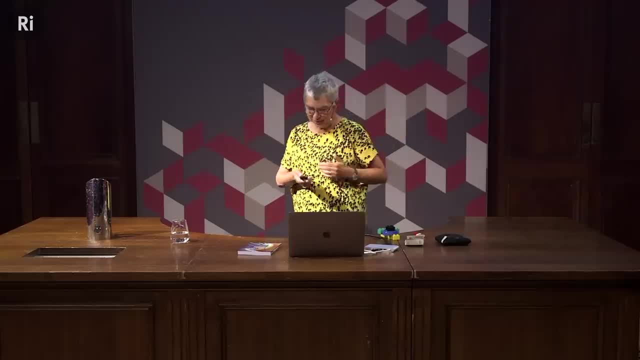 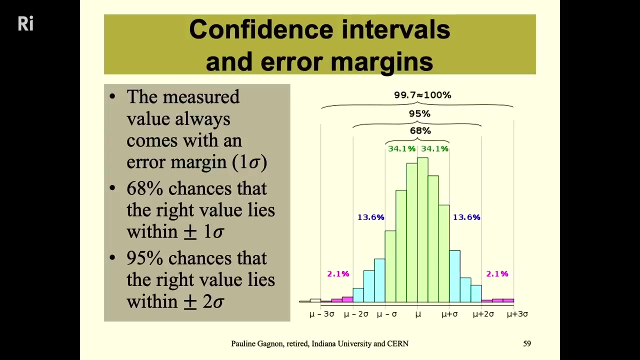 are now just background noise, that we're irritated with that, So we don't know what will happen. In physics, in particle physics, everything relies on statistics, And so we always measure. when we measure something, we also measure also the error margin. 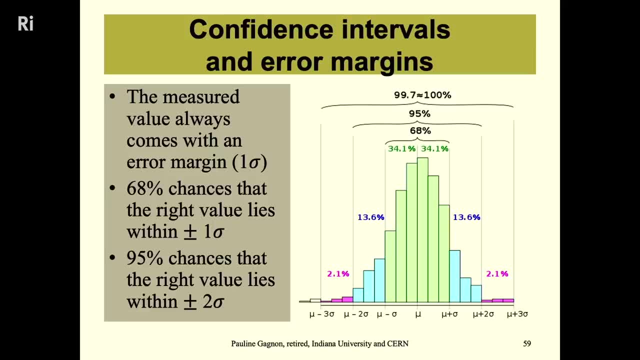 And we set our error margin. we call that one standard deviation when we know that there are 68% chances that the real value will be plus or minus one standard deviation. Standard deviation we represent by sigma, And if we take two standard deviations, 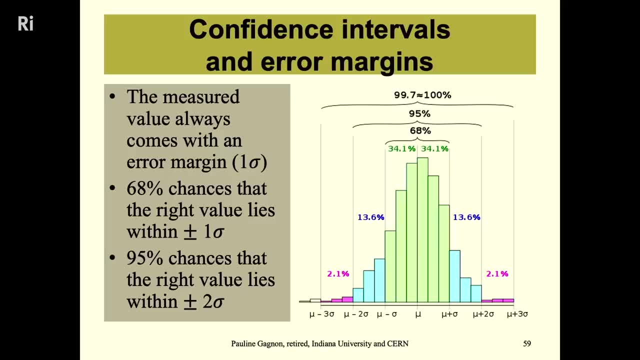 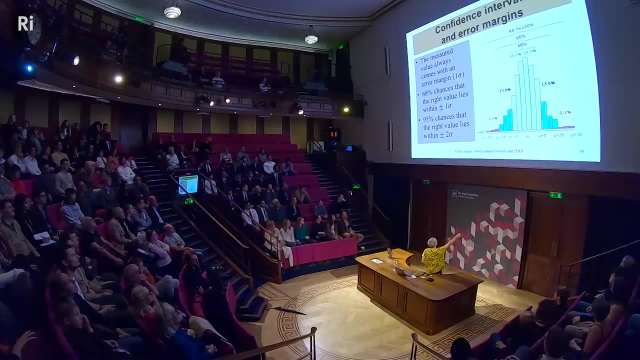 twice the error margin on each side, then we know that the real value of what we have measured. there are 95% chance that it's within that range. So this is the value that I have measured, the mean value mu. we see here: 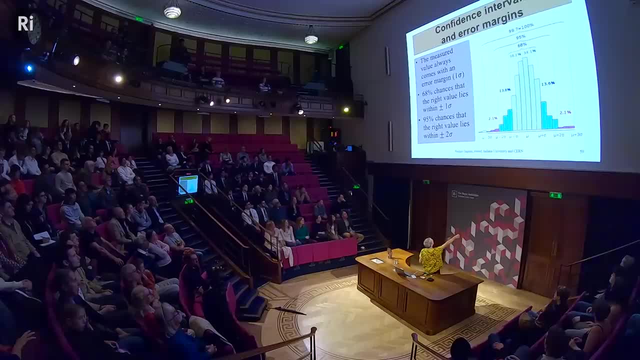 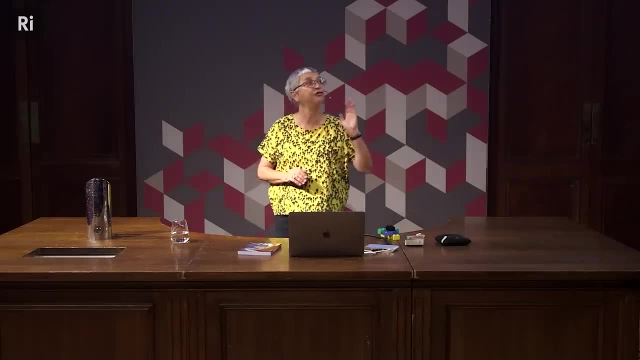 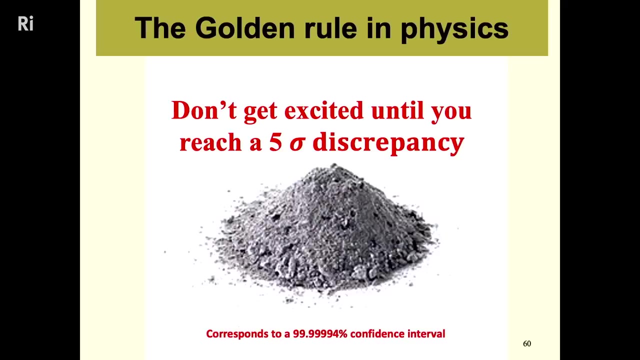 And within two standard deviations there are 95% chance that the real value is there. So in physics we don't get excited until we have a five sigma discrepancy. Five sigma corresponds to 99.9999994% confidence level. 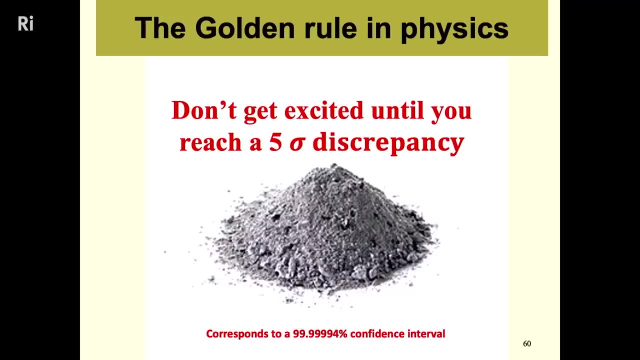 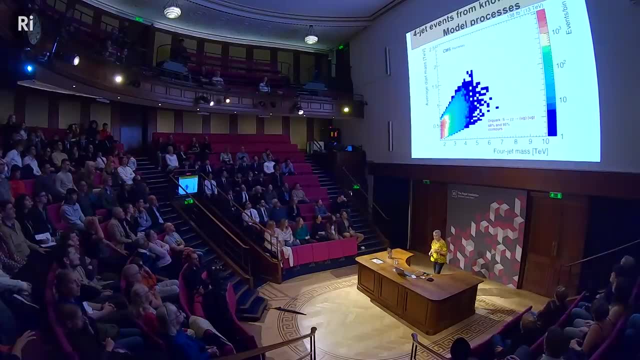 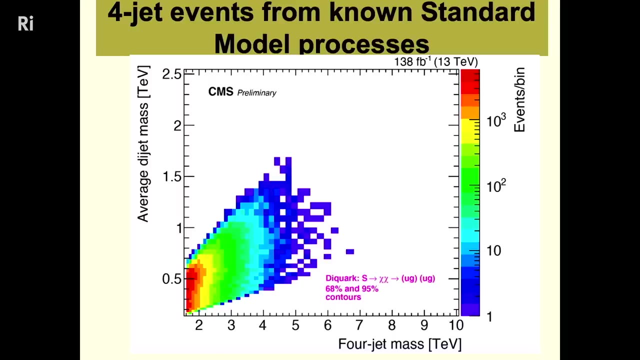 We don't want to be looking like fools, you know, saying that we found something and it turned out to be nothing. So the two events from CMS that I was showing earlier, if we were just to look at the distribution of four jets coming from two Zs: 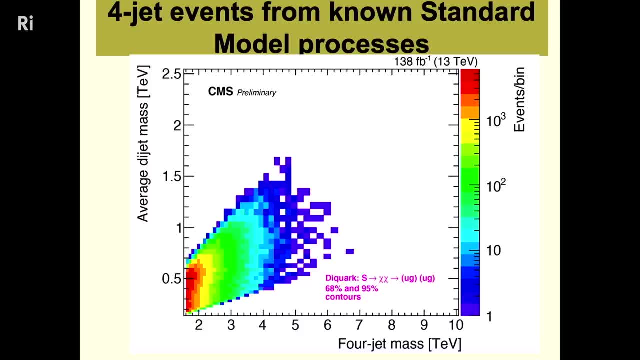 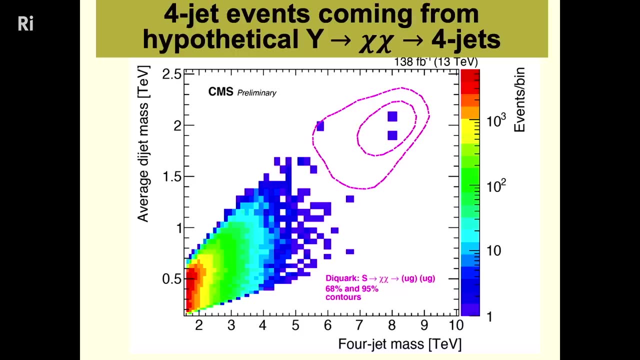 they would roughly be distributed like this. So here is the average mass of each double pair of jets and here for the four jet mass in total, And that would be the kind of distribution And the extra events that are found correspond to what we would find within a one sigma value. 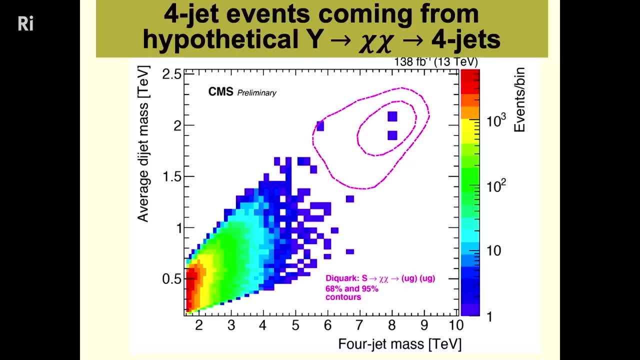 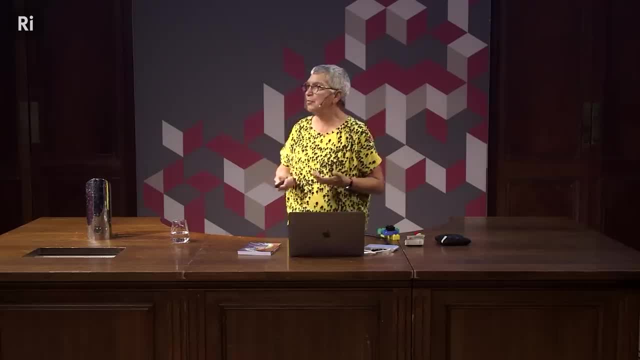 so 68% chance that it could come from a Y boson going to X boson. So the chances are we don't have much to go on these days, so when there are little things like that, we get happy. The biggest anomaly that we have at this point. 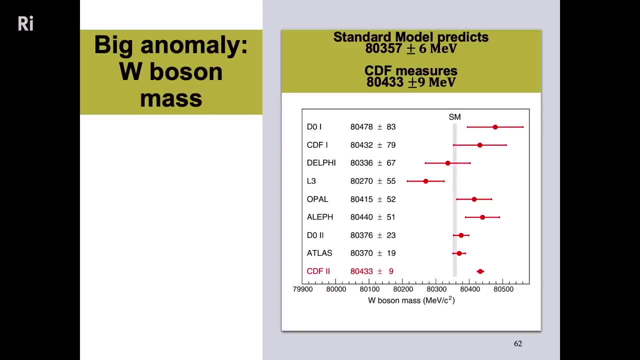 is when we measure the W boson mass. Very recently, about a year ago, the CDF experiment, which was an experiment going on at Fermilab near Chicago. they measured this mass with the highest ever precision and it was about. they measured. the mass they measured was 80,430.. 80,433 MeV plus or minus nine. So it's really really precise, But the value that theorists can predict from the standard model equation. there are all sorts of constraints. 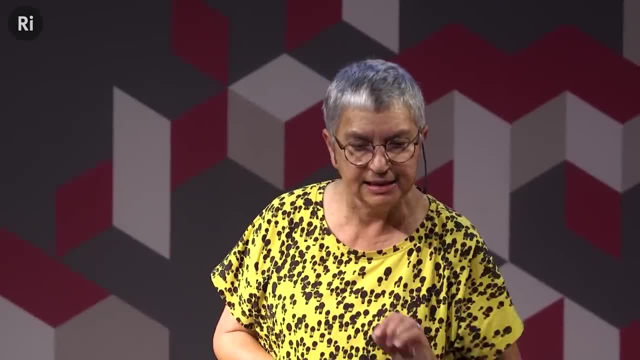 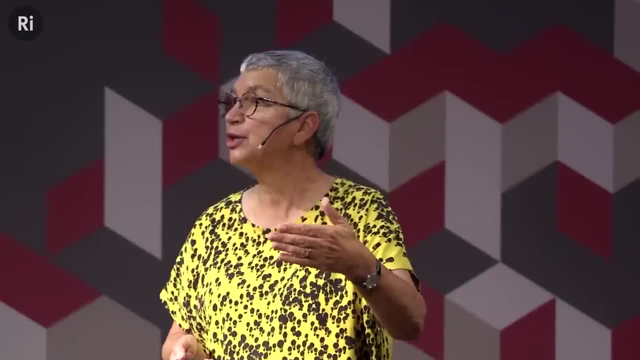 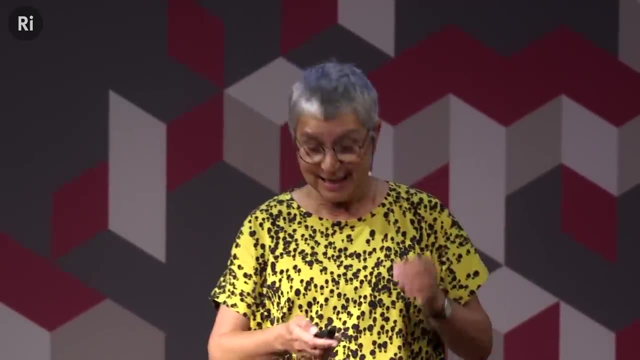 with all the mass of the Higgs and the other particles, and they say that it should be 80,357 plus or minus six. It doesn't match. There are about seven standard deviations apart. Oh, exciting, But it will take years before another experiment. 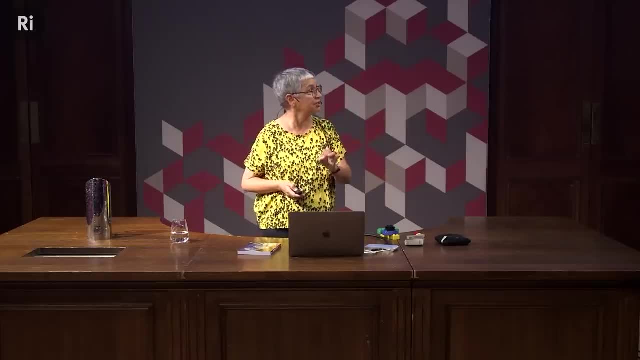 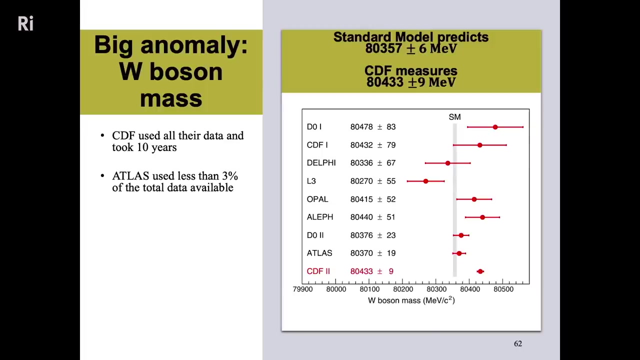 CDF is finished, so they've done that. It took 10 years to do their calculation, precisely So they're done. And ATLAS at the Large Hadron Collider could have only used 3% of their data and they have an error margin of 19,. 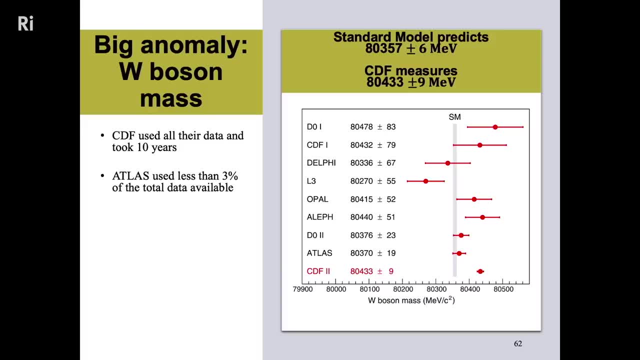 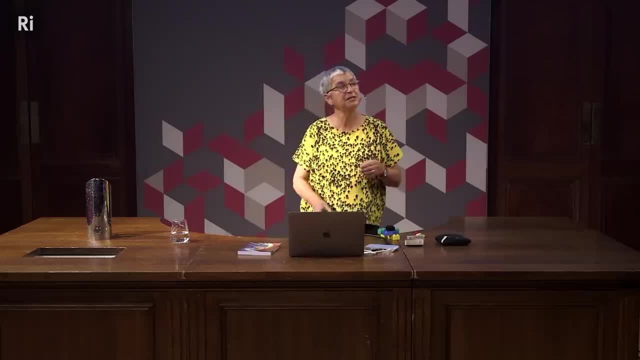 which is too big to be compared to a CDF. But to do the measurement again will take a huge amount of effort because there are neutrinos involved and neutrinos are very sneaky. That's why the little character is with a mask like this. 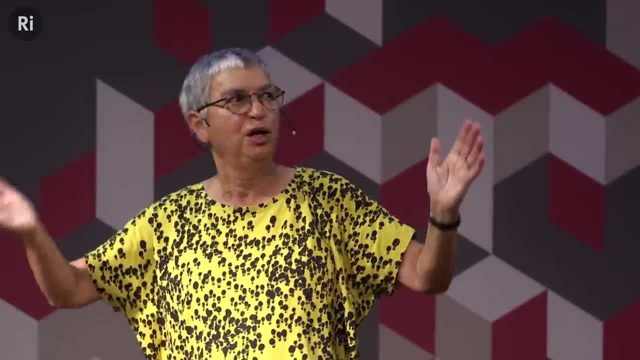 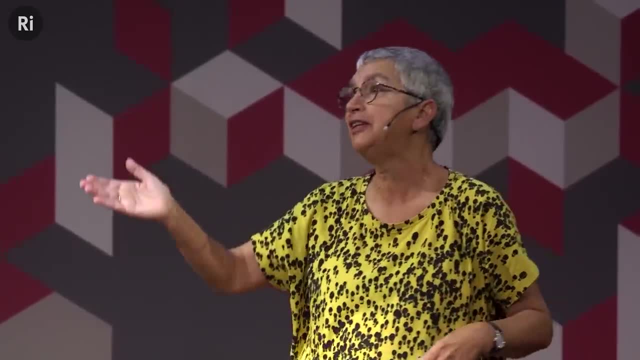 because they can go through the Earth. There are billions of neutrinos that went through this room during the time that I spoke and they didn't even stop to say hello. So you know they go through our detectors and we don't see them. 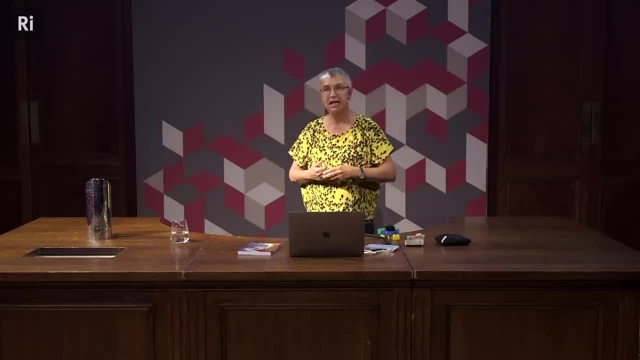 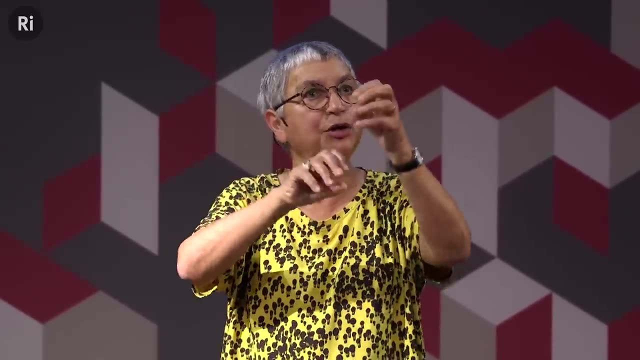 so it makes the measurements difficult for the mass of the W, And plus there is this pile-up phenomenon that many collisions happen at the same time. so it's difficult to disentangle all this, And it has to be so precise that it will take several years. 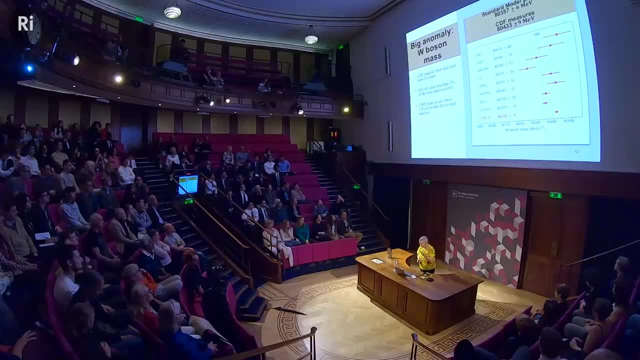 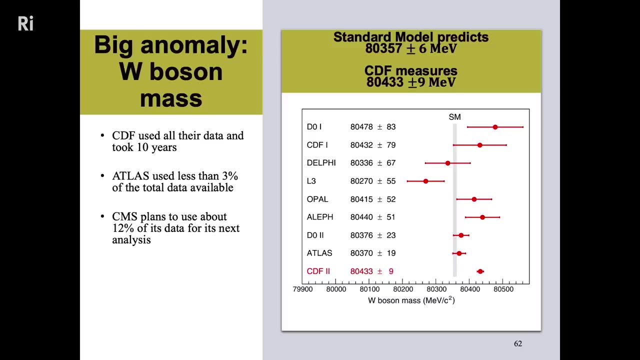 before we have new measurements on that. So the CMS collaboration at CERN plans to use 12% of their data where there is a little less pile-up- we say Not so many events on top of each other, But it's an extremely difficult measurement. 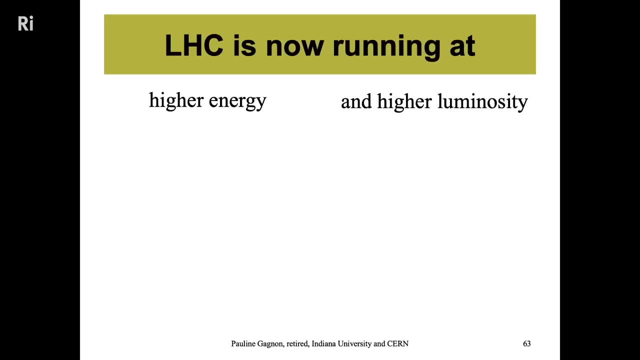 so it will take a while before we get that. The good news is that the LHC is now running, and it's running at a slightly higher energy than before and with higher luminosity, which means that it will have more data. So what are the benefits of that? 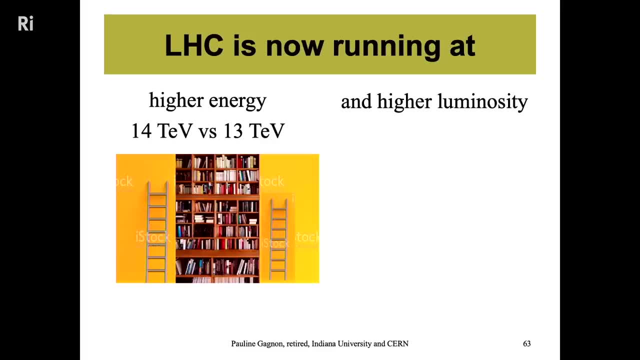 is that, if you're working at higher energy, it's like I'm telling you: oh, there is a beautiful book hidden somewhere in a library, an ancient book with all sorts of wonderful things, And I'm giving you, finally, a taller ladder. 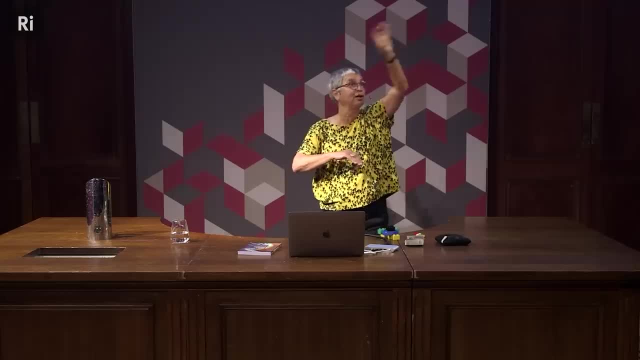 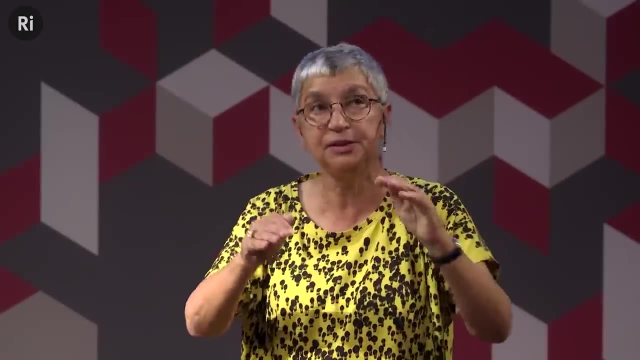 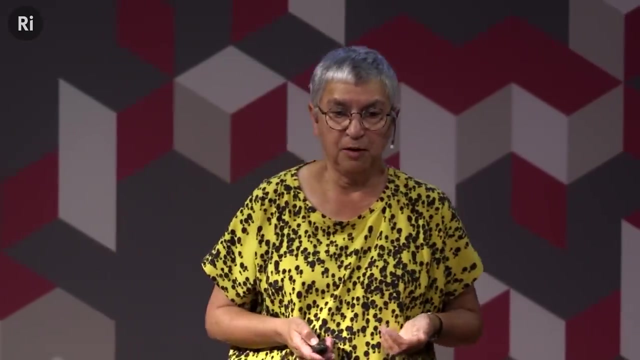 so you can reach the last rows of books at the last shelves. So when we were using 13 TeV, the energy of the accelerator. now we have a bit more, so we can reach new particles that were not accessible before, And higher luminosity means that. 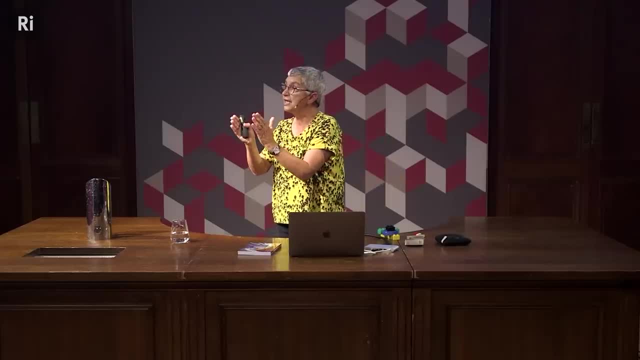 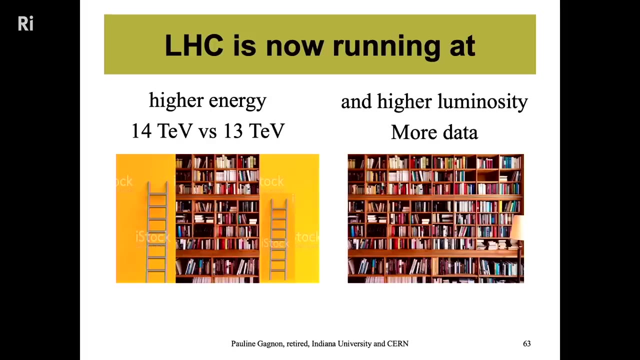 they will have more data. so we're not limited to a small section of the library but to a large one. So maybe we have a chance to find something new. But now it's really painstaking work of accumulating billions and billions and billions of events. 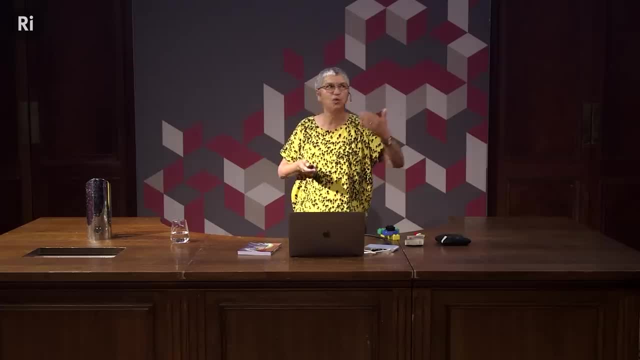 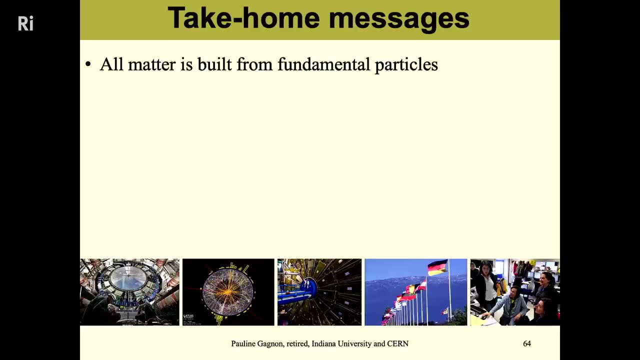 And in the next 10 years or so we should manage that and maybe we'll come up with something. So here are my take-home messages for you before slowly ending this lecture. So if you can remember that, all matter is made of a handful of elementary particles. 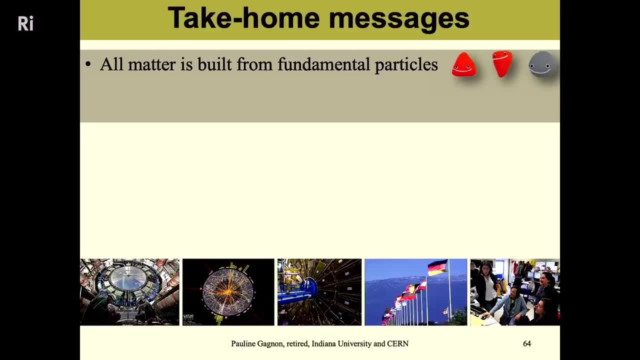 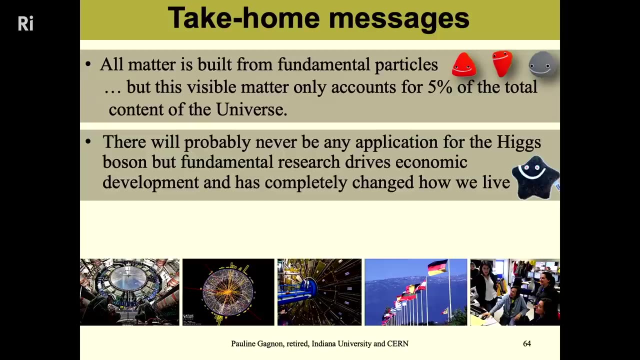 and those particles are the up down quarks and the electron. but this visible matter only accounts for 5% of the content of the universe. So what we have studied only explains 5% of what is out there. There will probably never be any application. 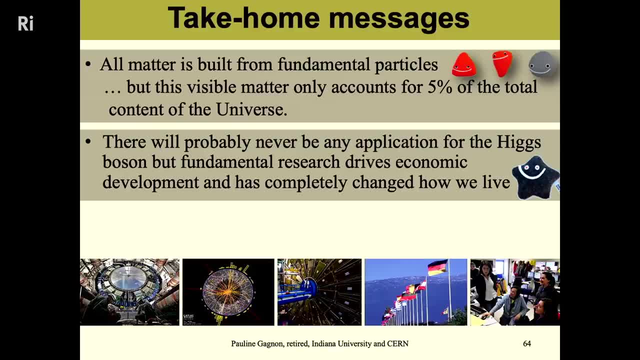 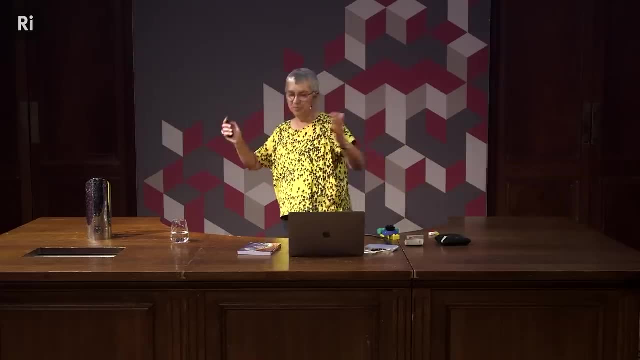 for the Higgs boson. but fundamental research drives economic development and has completely changed how we live. with the World Wide Web, It's a sure statement to say it has changed our lives- Electricity as well. Thank you, Michael Faraday. And any new particle or new phenomenon. 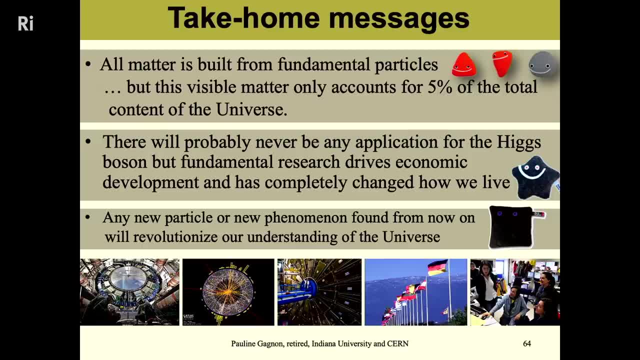 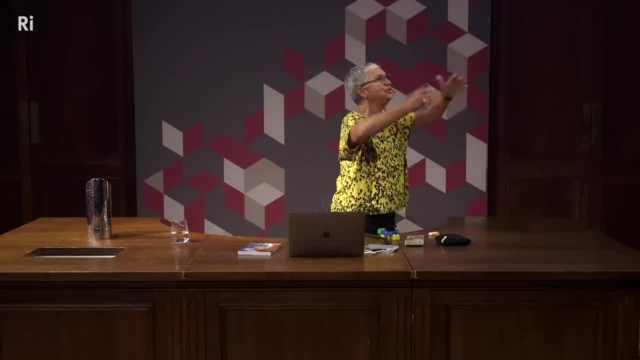 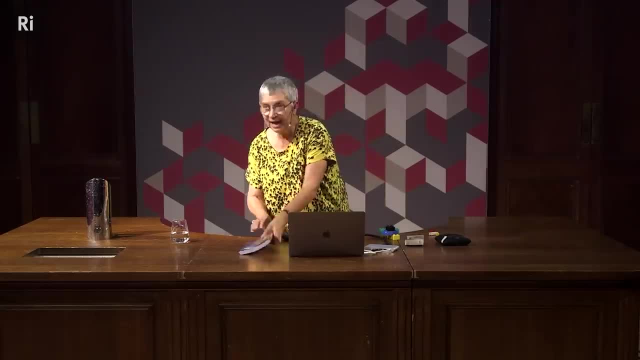 that we find from now on will revolutionize our understanding of the universe, because then it will finally tell us: ah, what is this new theory that we need to add on to the Standard Model? So before you go, I just want to tell you that I have this book. 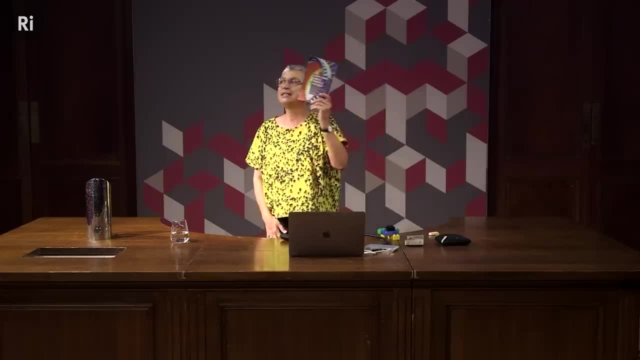 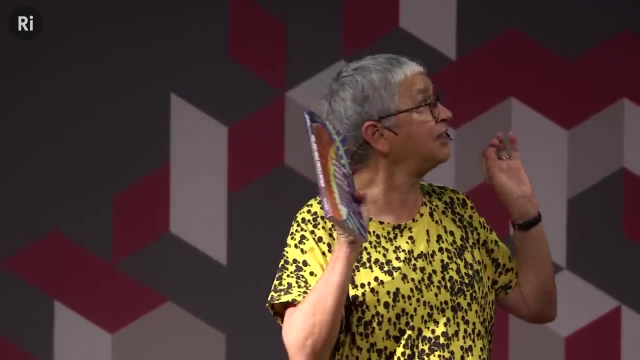 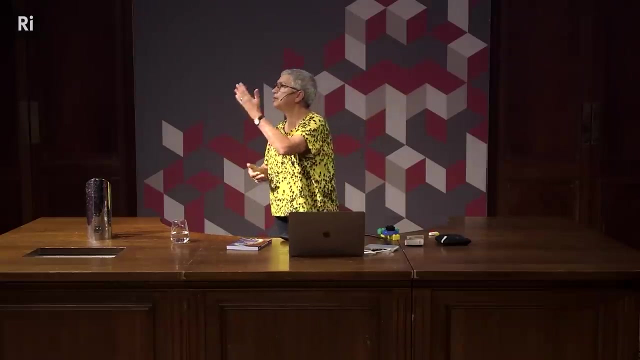 Who Cares About Particle Physics, And I swear this is the best popular science book on particle physics that I have ever written, And so I highly recommend to you all. and of course, tonight you know, I had an hour to explain to you all this. 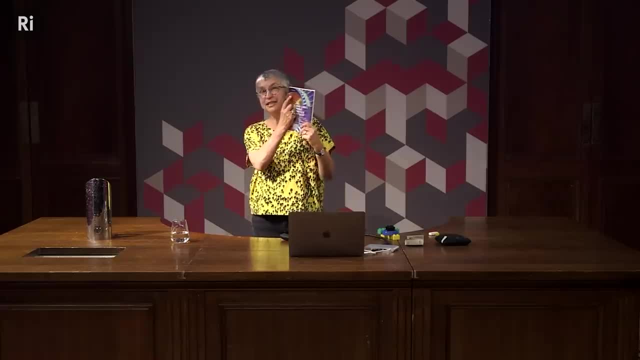 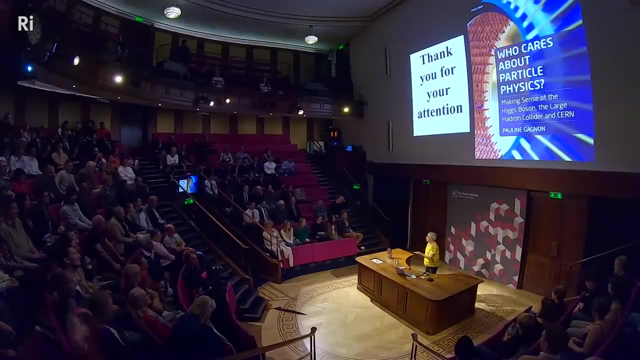 and with a bad accent on top of it. This is all written in absolutely proper Oxford English, so it would be much easier, And so you will learn everything about the Standard Model, how the detectors and the accelerator works, how we work at CERN. 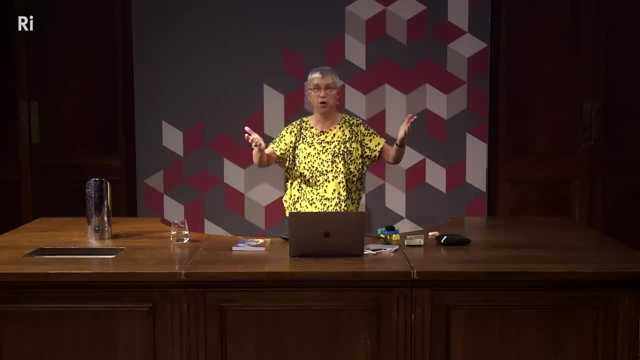 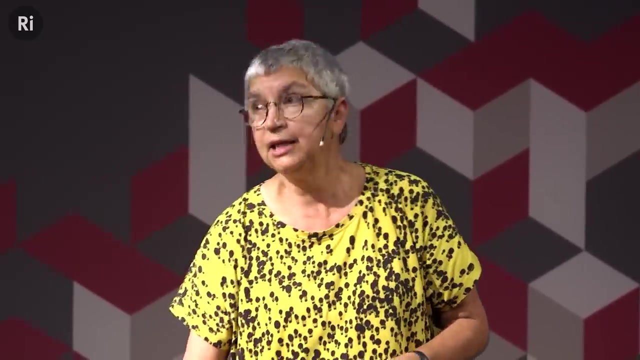 because nobody gives orders, We all go freely and do what we want and it works, And because you ask people to give their best. And then and then also about diversity in science, or the lack thereof, and also the story of Mileva Maritzenstein. 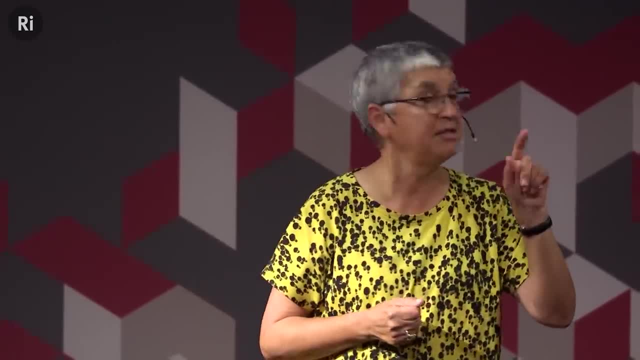 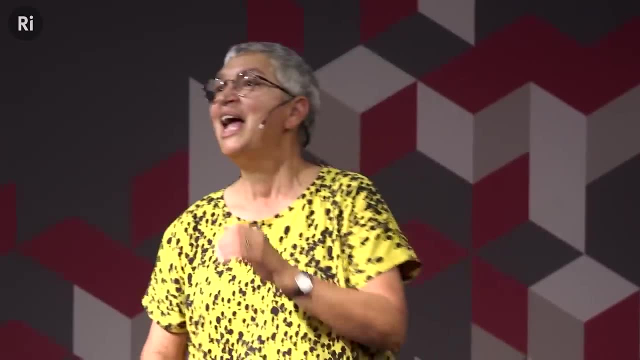 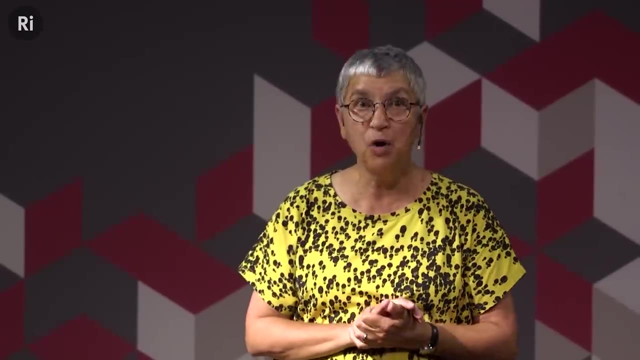 I've mentioned a few times the equation E equals MC squared. Who wrote this equation? Everything that Albert did in the beginning of his career was done in collaboration with his wife, Mileva Maritzenstein, But this part of the story is unfortunately not known. 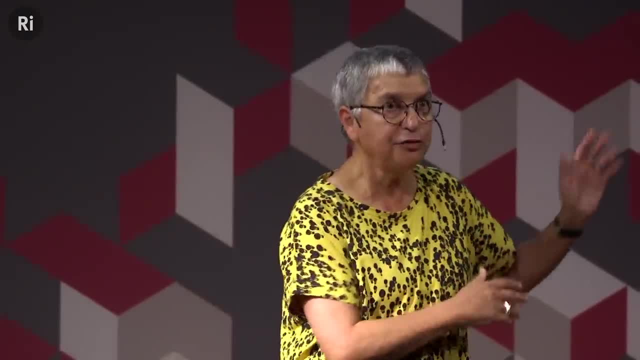 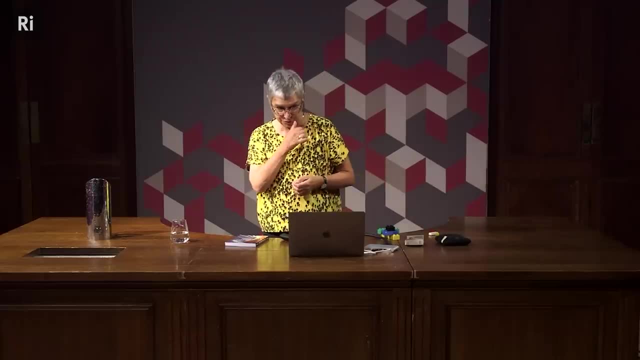 but there is a chapter in my book on this, So I'll be offering the book at a reduced price from Oxford University Press tonight, and a special price as well for the students. So if you're interested, I'll be there. And before I go, 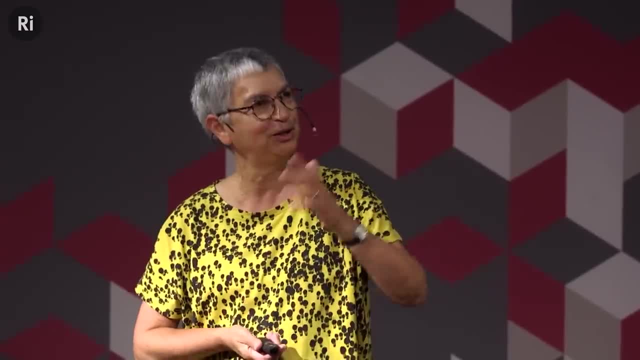 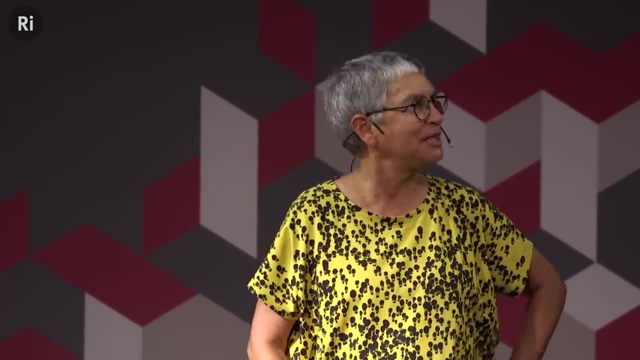 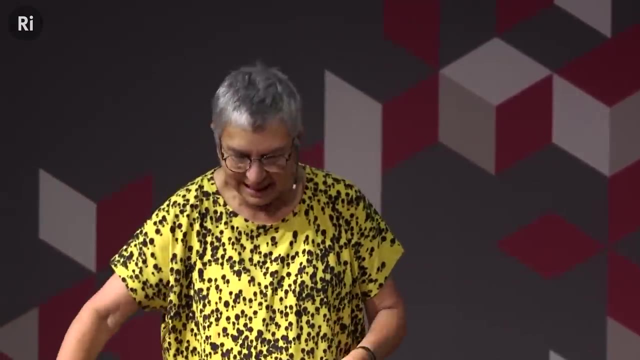 I tell you this musical about Tina Turner and all that. Alicia Paul Moses did such a performance and such a finale and all that, And it's just you have to see it. It's amazing, you know, But I need you to help me. 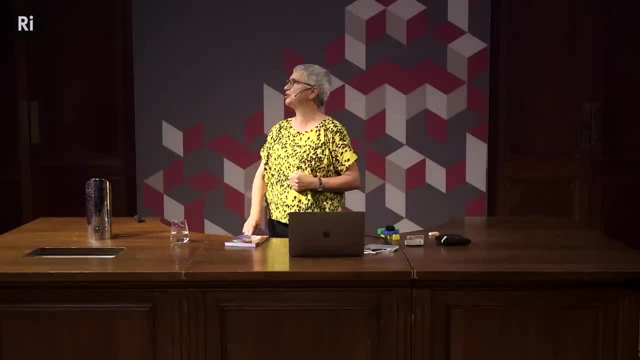 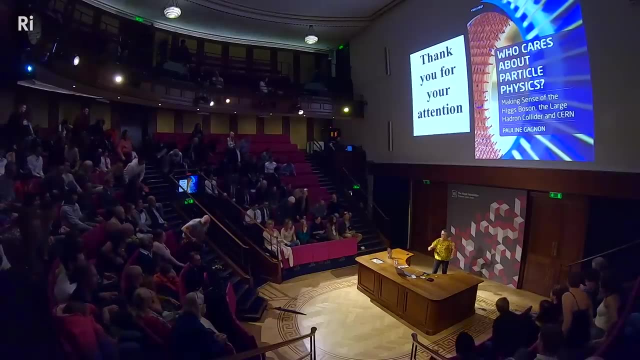 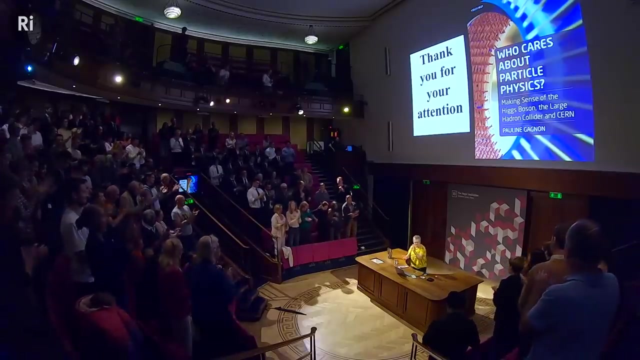 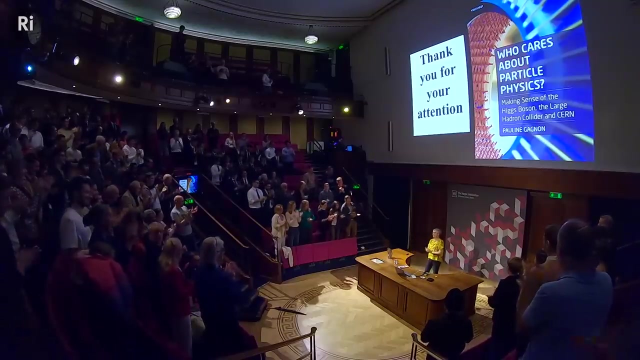 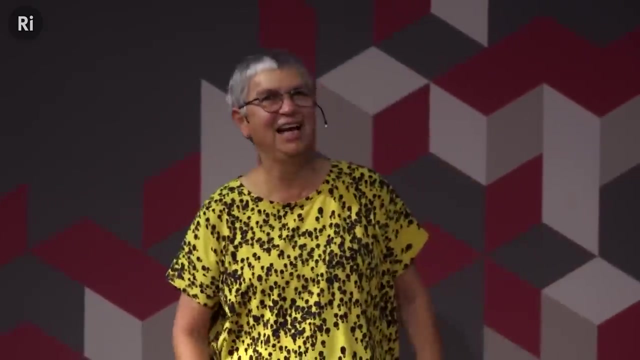 Now we should rock the Royal Institution tonight. So please join me. Stand up all of you, please, And let's try to give a bit of spice in that lecture, you know, And be quite silent. That's one way to get a standing ovation. 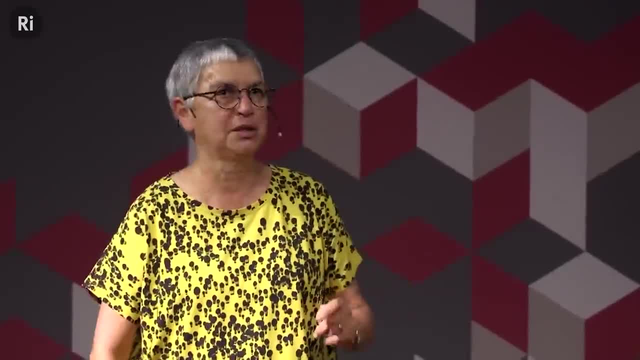 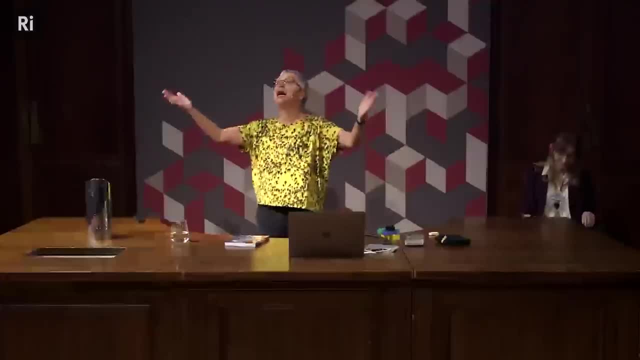 But what I was going to tell you from Tina was: oh, what's Higgs? what's Higgs got to do? What's Higgs got to do? got to do with it. But now I hope you can answer that question. Thanks a lot.